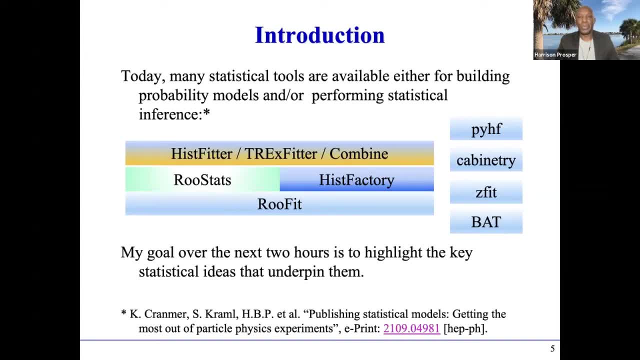 it is very easy to simply run some of those tools to arrive at the results, some of which we've actually talked about today, some of the SUSY results And, in fact, if you ever get a chance to look at the talk by my colleague Kyle, who is a professor at the University of New York, 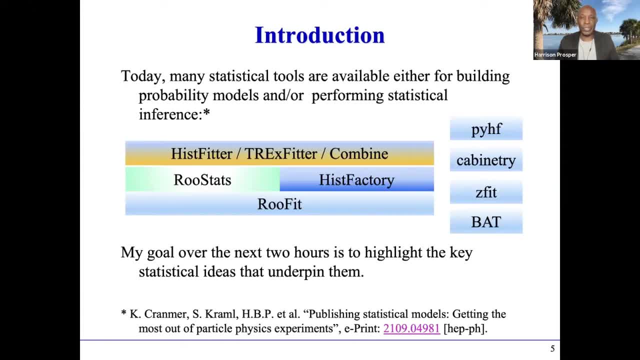 he's going to talk about the results of these tools And he's going to talk about the results of välkrana. He's very fond of showing a picture of a of the Higgs combination between Atlas and CMS And you'll see in that model an incredibly complicated model that we use to actually arrive. 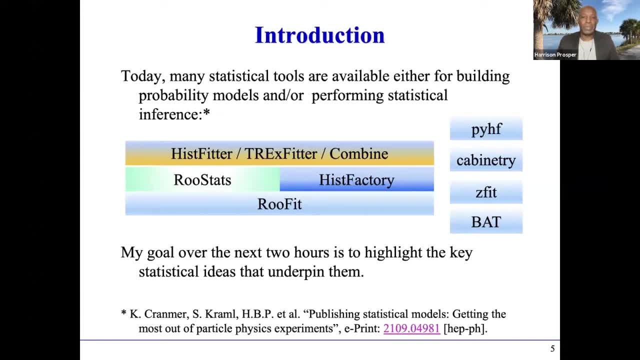 at these various results, But I think what I want to do, though, is I want to really focus on, on really basic things, So I'm going to actually consider a very, very simple model which, nonetheless, is actually realistic, because it's based on a very, very simple model, And it's 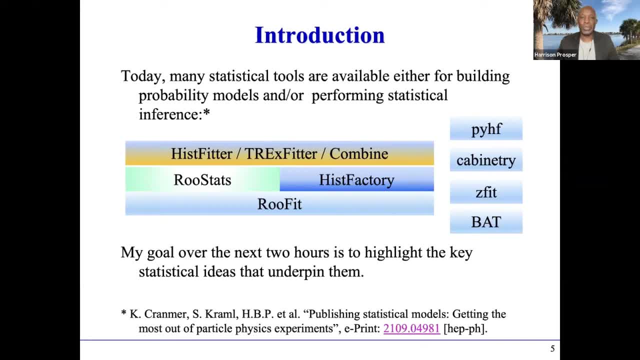 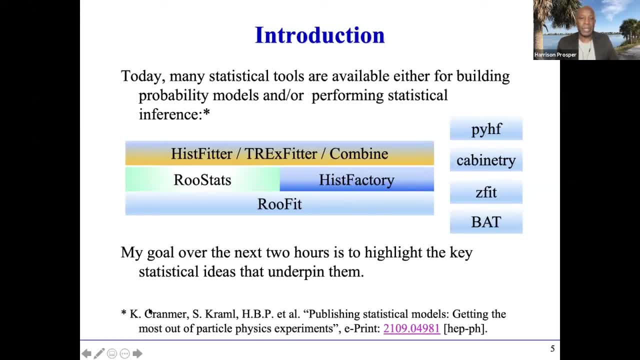 By the way, I would like to take the opportunity to advertise this recent paper by Kyle Sabina and myself and the 33 other colleagues, entitled Publishing Statistical Models: Getting the Most Out of Political Physics Experiments. I am of the opinion that the field would benefit greatly from having we experimentalists 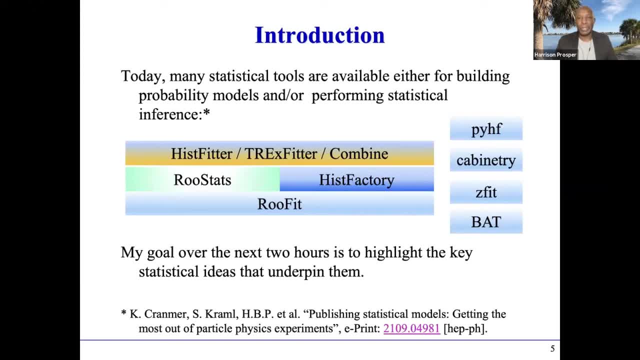 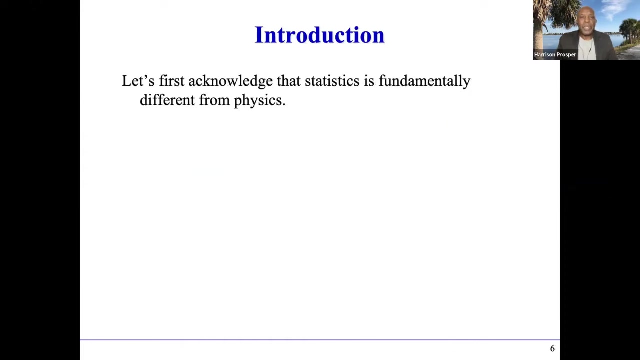 actually make our models available to the broader audience of you know statistician friends, our theoretical physics friends, because I think if those things were made public we could really make a great deal more use of these data that have been collected. Well, let's first acknowledge something that I think is really true: that statistics is. 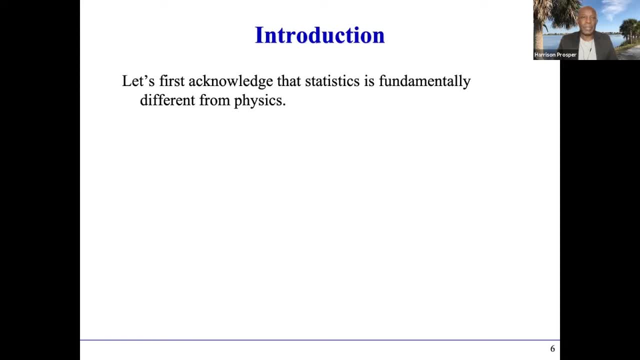 not physics. It is very different from physics And in fact, let me just quote Richard Feynman. The great thing about physics is the following: right is that you can have a fantastic idea, a beautiful theory. We've been discussing supersymmetry, which is a beautiful theory. 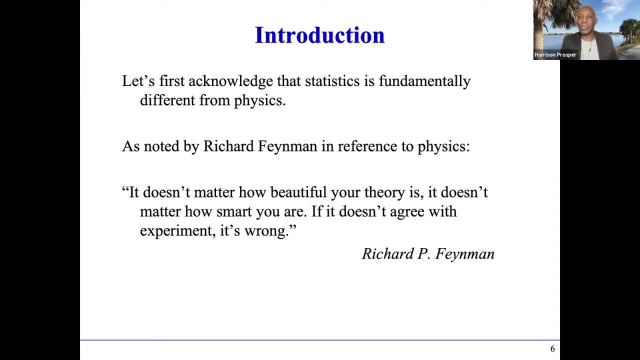 And let's say this is 2040.. We've been working extremely hard And yet there is no evidence whatsoever of supersymmetry. Then at some point, you know we have to move on Or, worse still, we actually find something that actually categorically disagrees with. 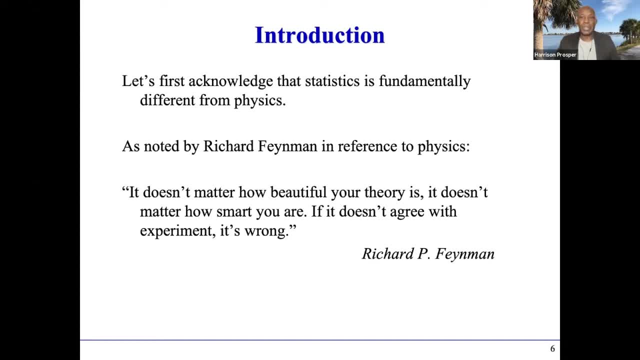 the prediction of supersymmetry, then it would be wrong. So this is what's fantastic about physics, because we have nature as the arbiter of what is correct, And this is marvelous, Whereas in statistics we have a lot of physics. 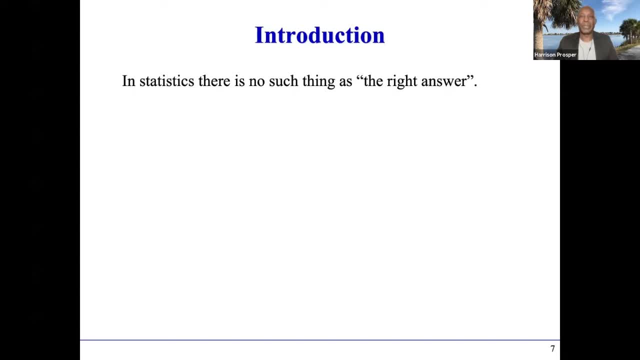 There's no such thing as the right answer. There are many answers, in fact, And these answers are based on different assumptions and different principles. And because they're based on assumptions and principles, well, you may have one colleague who has made certain assumptions or prefers certain principles, and they will arrive at 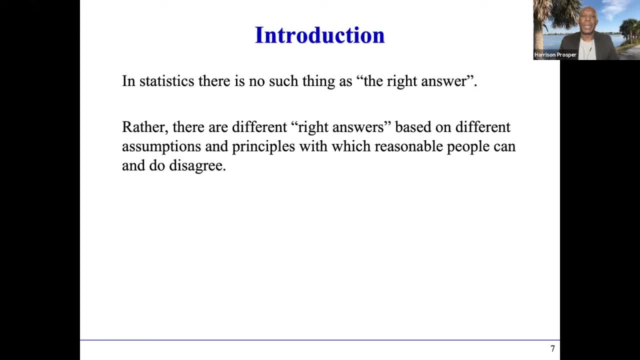 a different answer using exactly the same data, And this is an important point to bear in mind. And this is an important point to bear in mind when one is engaged in these analyses. So, even all the papers that have been published so far from the LHC, especially the ones in 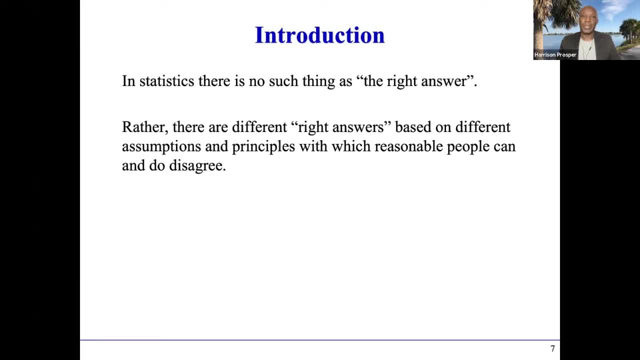 which limits have been set, for example, for Susie. underlying those results are assumptions and principles with which people could disagree and do disagree, And therefore any change in those assumptions could actually lead to- could have led to- different conclusions, And this is something that's important. 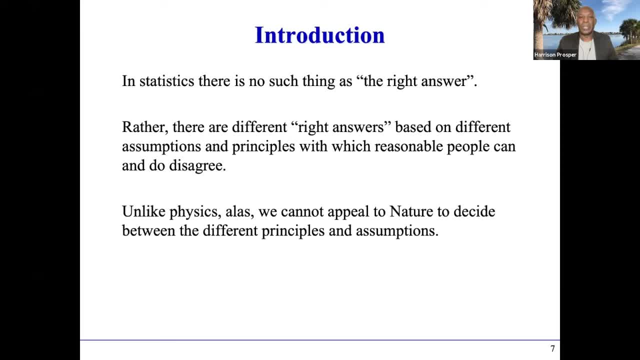 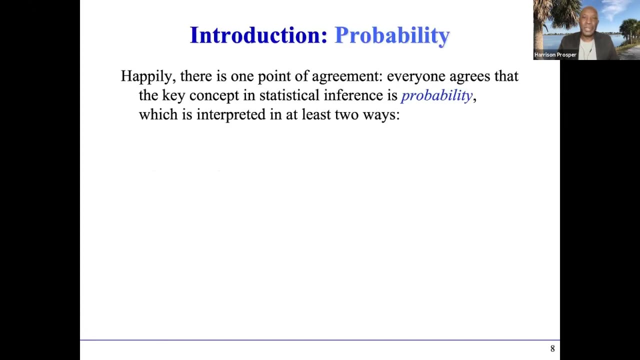 And unfortunately, we cannot appeal to nature to decide between the different principles. At the end of the day, it's really a matter of intellectual taste, And that can vary from one person to the next. Nonetheless, the good thing is the good news is that there is one thing that everyone seems. 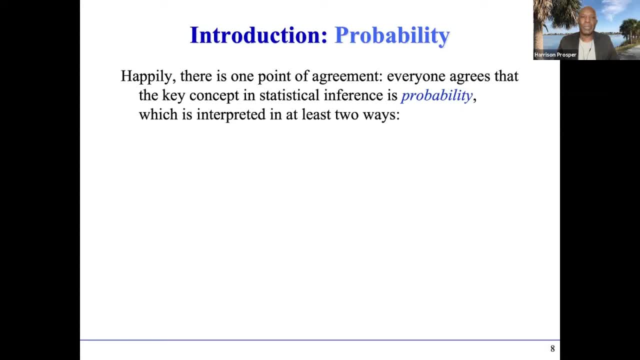 to agree upon, which is that the underlying concept, the basic concept that underlies statistical inference, is probability. However, it's not just probability, However. so we all agree, this is really a key. but this concept, this notion, is interpreted in at least two ways. 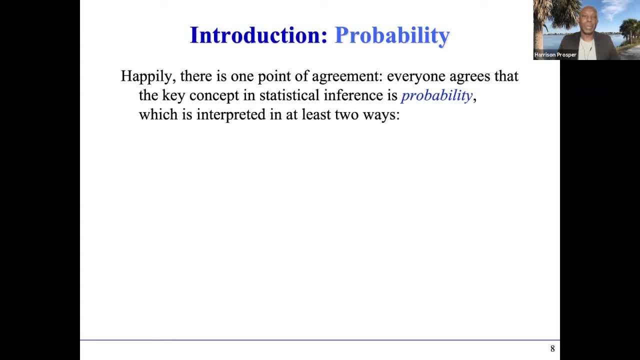 There are many other ways, but at least two that are used in particle physics. The first one is actually the older interpretation, which goes back at least two centuries and probably more, And that is the degree of belief in a proposition. So we'll mix a proposition. 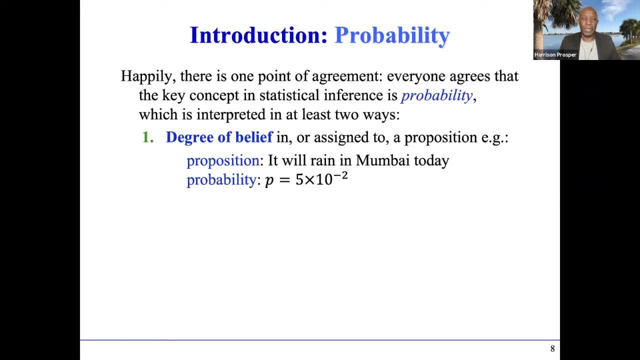 It will rain in Mumbai today, And you, specifically, And you specify some probability. Now, of course, the event today, 22nd of November 2021, is a singular happening that will never happen again in space-time. Nonetheless, you can assign to it a probability, that is the degree of belief in that particular. 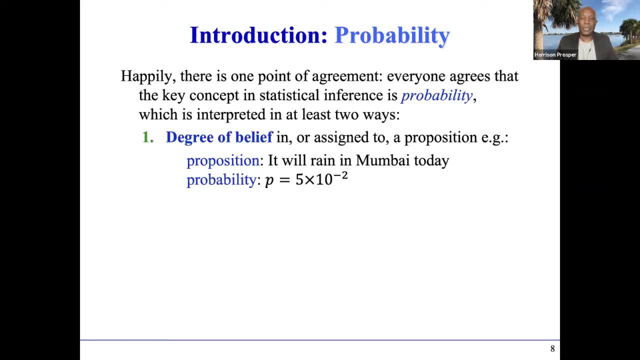 statement. So that's one sort of interpretation of probability. The other one, with which we're much more familiar, and the one that physicists don't typically prefer, is the relative frequency interpretation. So what one imagines is that one repeats a certain thing many, many times. 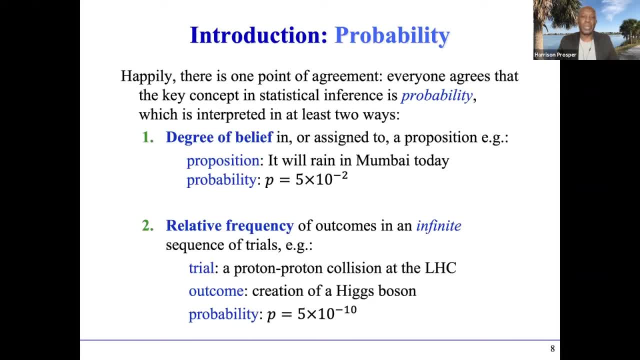 We have a fantastic ideal machine for doing that, the LHC, where every collision is a trial And either something happens that's interesting or something happens that's not interesting. So perhaps one outcome could be the creation of a Higgs boson, and we hope that one day. 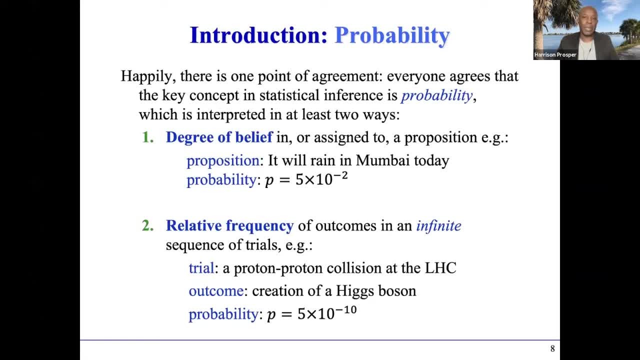 the creation of something truly new and unexpected, and one assigns a probability to this, And so the idea here is very simple. The idea is that you repeat these trials many, many times, You count how often a particular outcome is realized and you take the ratio of these. 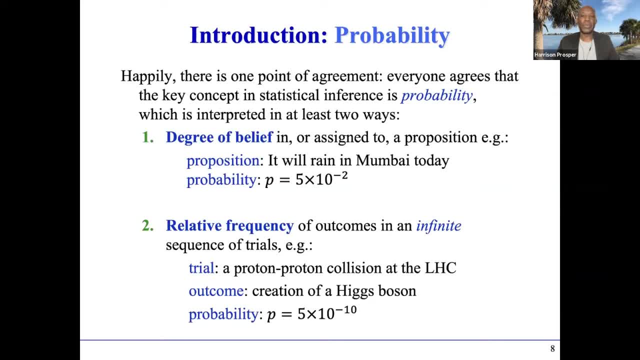 two counts and you call that the relative frequency, And one presumes that if you continue to do this for an infinite number of trials, that fraction will settle down to a number that we call the probability. So these are the two interpretations. 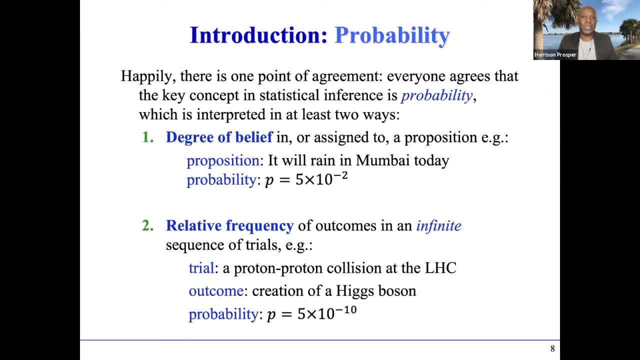 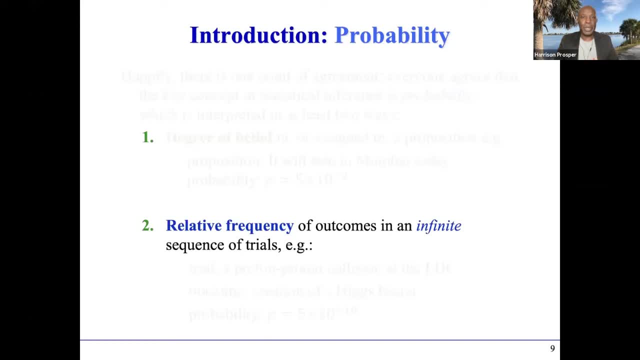 And, as you can imagine, they lead to different ways of reasoning about statistical analysis. So we're going to start by considering the Frequentist approach, which uses this relative frequency interpretation And you know, please feel free, especially the students, you know this is for you. so 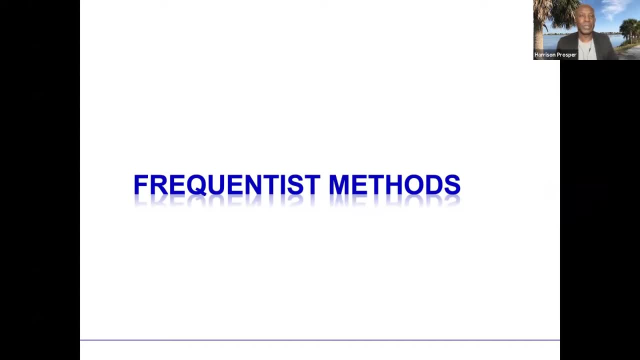 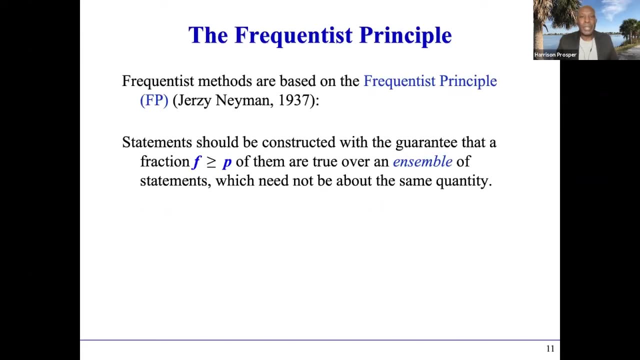 feel free to ask questions at any time. Thank you, Thank you both throughout the two talks. So if we go back to 1937, there was this amazing paper by Yajek Neyman who basically espoused this particular principle. His idea is this: 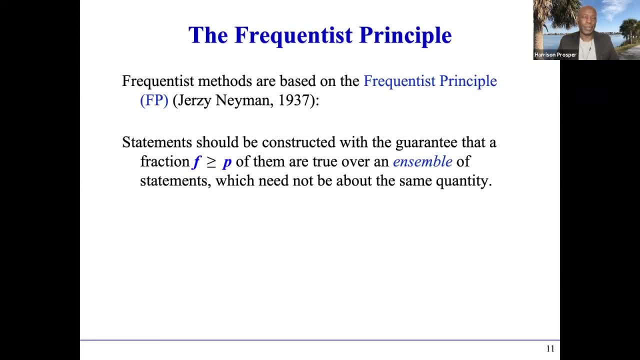 We should construct statements. you know, let's say, some particular parameter is below some threshold. Once you construct statements with a certain guarantee. The guarantee is that over an ensemble of statements, you guarantee that a fraction f greater than or equal to p will be true. 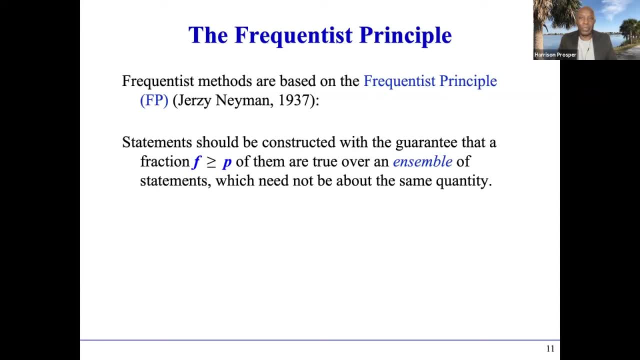 Now, of course, we are not privy to which statements are true, which ones are not true. Right, We will never know, because we can only ever know, probabilistically, something about the true nature of the world. But the point is, is that one wants to construct statements that are true? 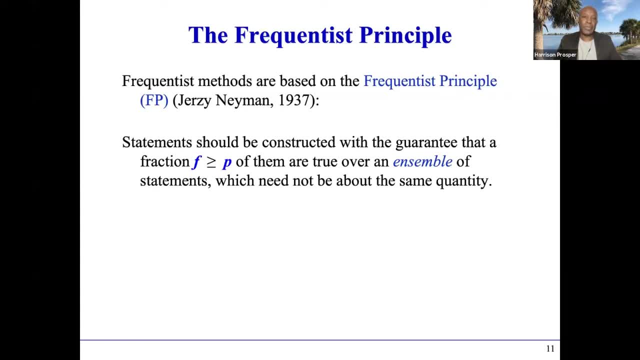 Right, And if you construct statements such that you guarantee that, whether or not you know they are true, what you at least want to guarantee is that, over a huge ensemble of statements, some fraction- minimum fraction- of them are true. This is the so-called frequencies principle. 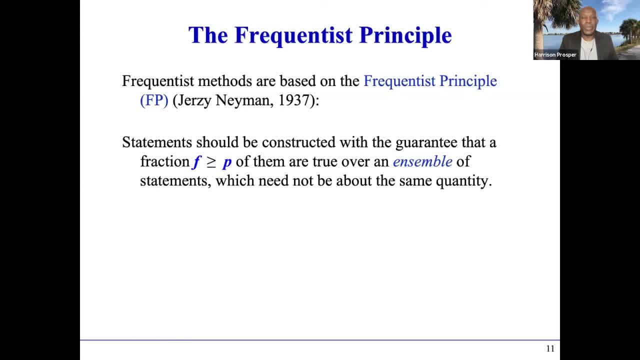 And it's a very important one because in some sense it's sort of a quality control, a kind of a guarantee that we are doing something that's reasonable. So here is an example: In 2014, the Earth was very bad- the Sion's collaboration published this nice paper on the analysis of Higgs decaying to 2z. 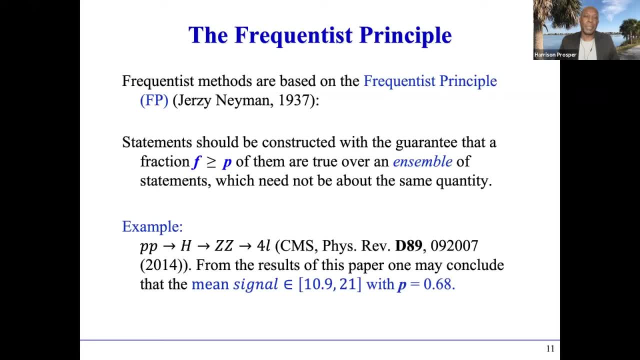 bosons, which then subsequently decayed to four charged leptons. And if you look at the results of this paper, one thing you can conclude is the following statement: that the mean signal, that is, the mean Higgs signal, in this particular channel lies within this range: 10.9 events. 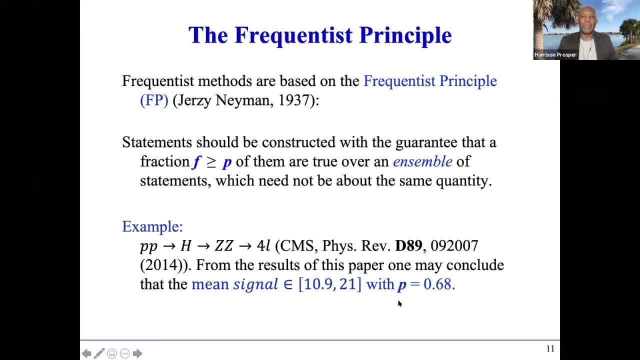 21 events with a probability of 0.68.. So that's the statement. The statement is either true or false, And we do not know which it is, because we do not know what the true. we'll never know what the true signal is. But the point is that if this statement has been arrived at in a certain 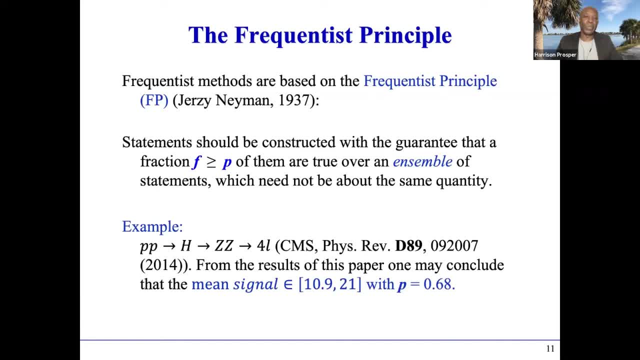 way. then there's this guarantee that if you look at many such statements from ATLAS CMS, going back 100 years to the discovery of the electron by JJ Thomson in 1897, all those statements that have been made with a probability of 0.68, the presumption is that 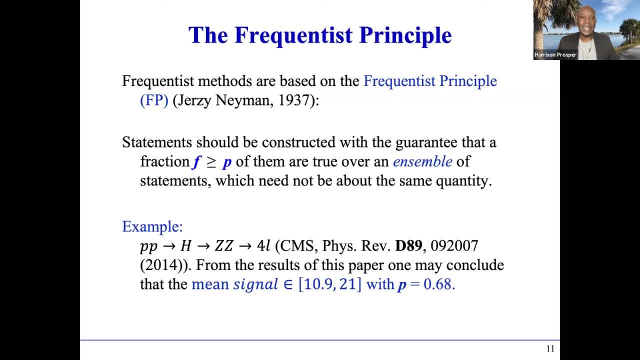 at least 68% of those statements are true, even though we do not know which ones are true and which ones are false. That's the Frequentist principle, And that's what one tries to adhere to by constructing things in a certain way, as we shall find out shortly. 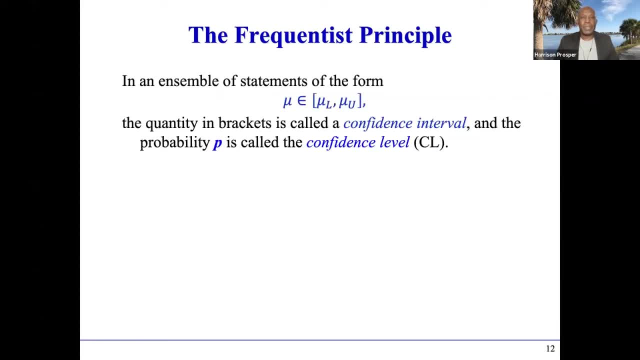 Now, the statement I just showed you about the signal is of this form: right, that some parameter lies within some bounds, And those bounds can vary from one experiment to the next, because the upper bound, lower bounds of mu sub L, mu sub U depends on the data that have been. 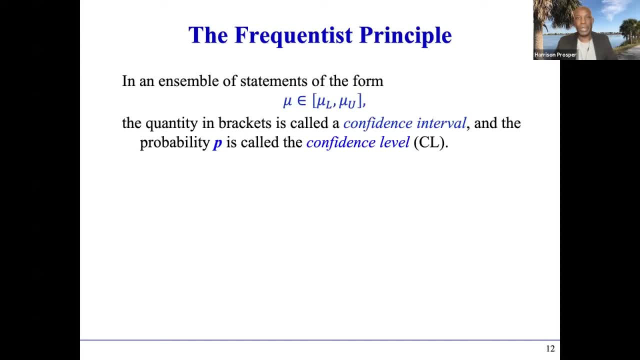 observed And obviously, if you repeat the experiment, you get different data and that will lead to different lower bound and different upper bound. So these intervals vary and it is these intervals are referred to as a confidence interval- And you'll see why the word confidence is used in this context- And the probability p. 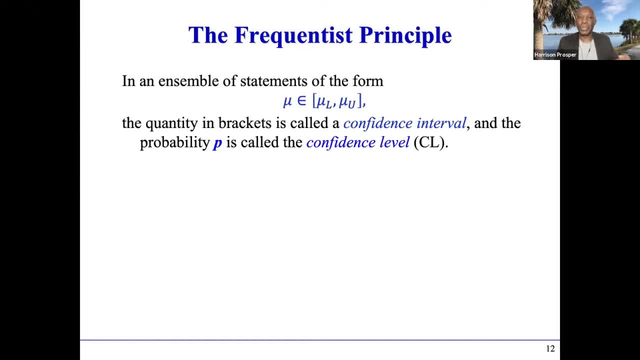 remember p was that lower bound because we wanted to guarantee that a fraction f greater than or equal to p of all these statements are true, That p is called the confidence level And the statement I showed you before has a confidence level of 68%. 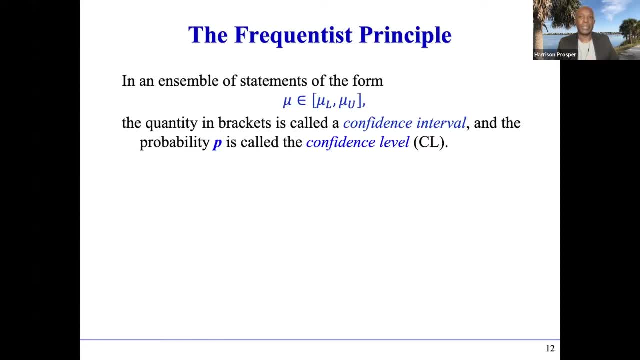 So we want to be able to construct such statements. That's very important. So you've just seen, for example, in these very nice talks on supersymmetry, these various curves in two dimensional planes, these so-called occlusion limits. well, those have a very definite meaning. 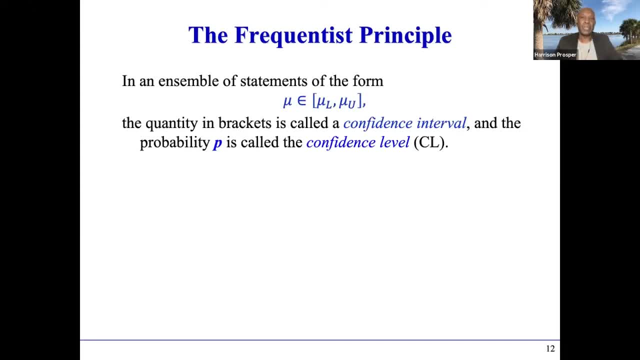 And the meaning, of course, is that, again, if you were to repeat the experiment, you would have the experiment a thousand times, a million times, a billion times. then, of course, these curves would vary. They would vary all over the place on these planes, And what one wants to guarantee is that 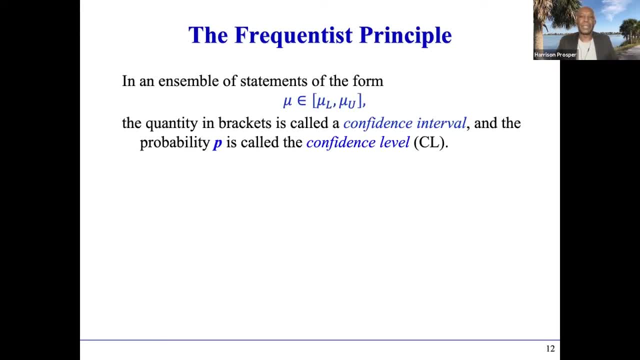 among this ensemble of statements, the 95% of the statements that each true value lies within or is above such a curve, 95% of those statements would be true. That's at least the goal. Now, the fraction f of true statements over this ensemble of statements is called the coverage. 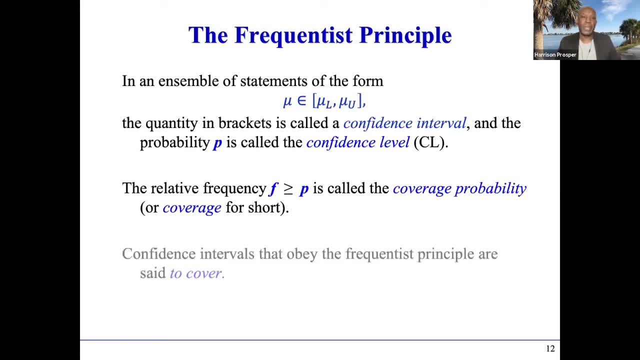 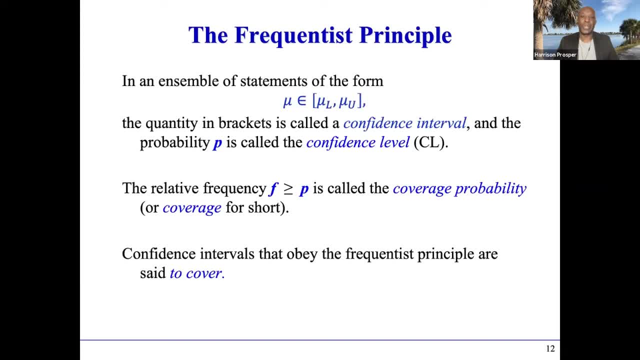 they actually include the true value, whatever that might be- of a particular parameter of interest. It could be some SUSY particle, the mass, or it could be the Higgs boson mass, or whatever it is that you're measuring. Then we say that those intervals cover. So that's the idea. 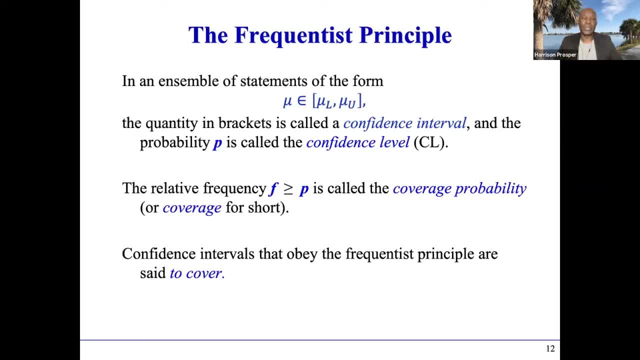 So the idea then, just to summarize, is that you have some procedure that allows you to compute a limit right or an interval or something like that, and you have some procedure that allows you to compute a limit right or some some, you know some sort of a bounded surface, and the idea is: 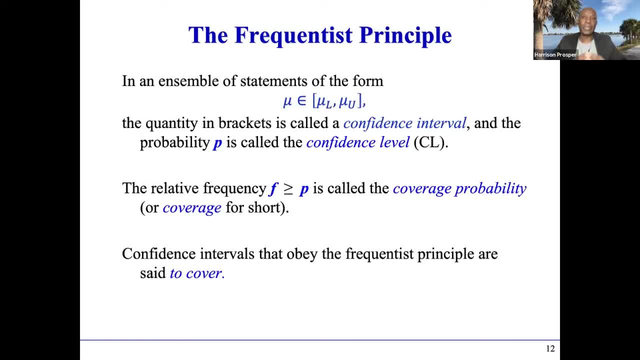 that you want to guarantee that, if you apply this procedure repeatedly on different different experiments and you make a statement that the true value of the quantity that you're trying to measure it lies within that boundary, that you want to guarantee that a fraction of those 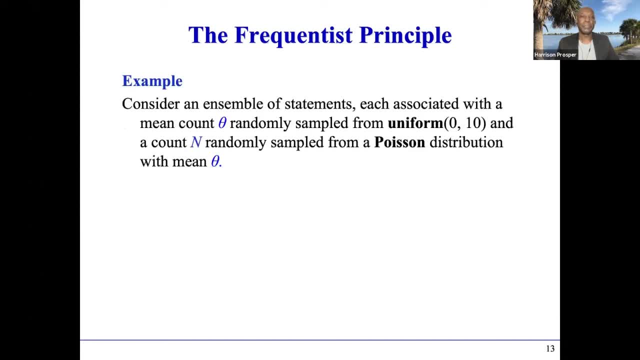 statements would be true. That's the goal. So here's an example, But I put in here. so, by the way, I've I've included in the slides Josh sent to to Shima later. I put in some exercises that I would really recommend the students try. 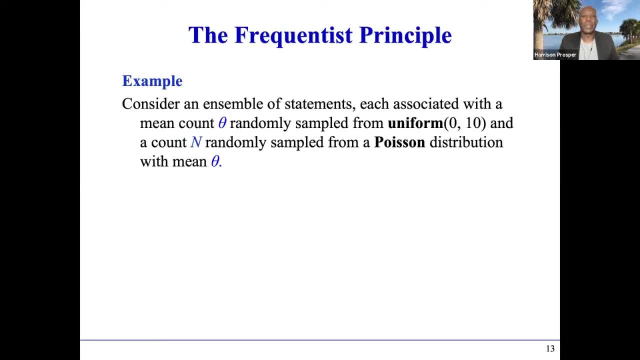 because I think those would be very helpful to clarify some, some concepts. So imagine that you you live in a world in which the mean count is randomly sampled from some uniform distribution, say from zero to 10. And that kind of makes you know. that's just a very rough thing, but it. 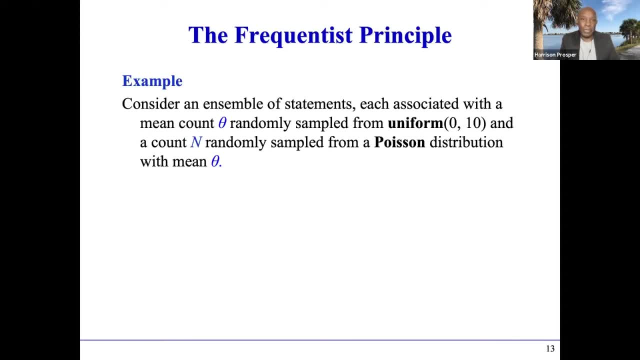 but after all, we never actually repeat the same experiment, right, We always do a better experiment. We are never, ever going to repeat run one of the LHC, nor are we ever going to repeat run two of the LHC. What we do is that we do another experiment And and therefore the mean. 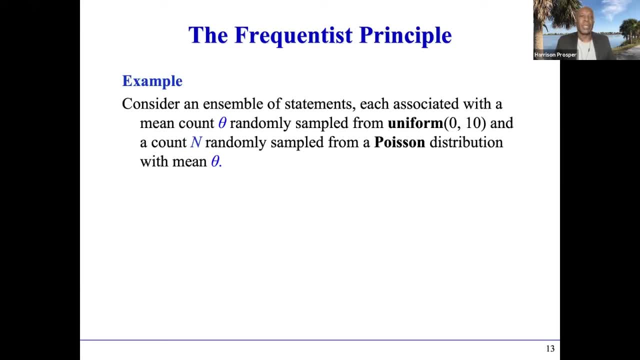 counts in the different experiments is going to be different And and therefore in in reality that's what one expects. So imagine that: yeah, so we have a uniformly sampled mean count And then, given a mean count, there's a randomly sampled count n from a Poisson distribution with mean. 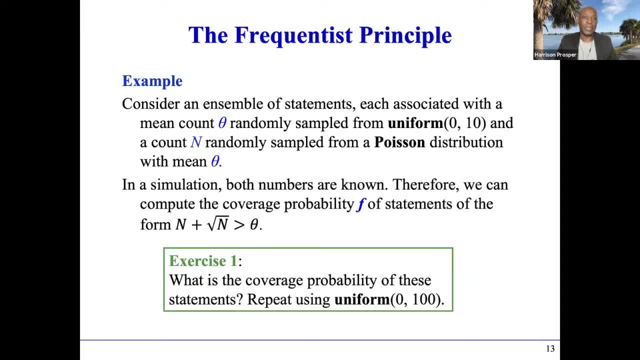 theta. So now we're going to ask a question. Let's make a statement. Let's suppose we make the statement that that n plus square root of n exceeds theta. Now of course, in the real world we can never decide whether that statement is true or false. right, It's, it's. we have no. 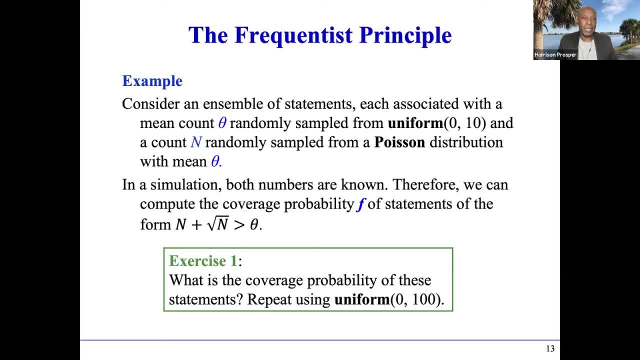 way to do so. However, in a world that's simulated on a computer, we know everything because we are godlike in the computer right. We, in simulation, we have the, we have the, the, you know the knowledge of everything that exists within our simulation. Therefore, we can actually 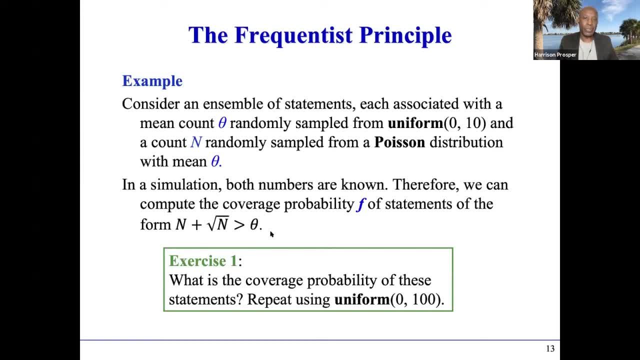 count how often such a statement is true, And that would be the so-called coverage probability. So one exercise that I would recommend that students do is just to do that is to literally sample from this distribution and then to simply count how often this particular statement is true, And that counts. 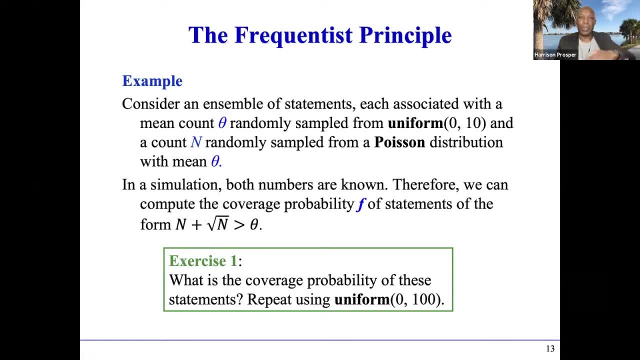 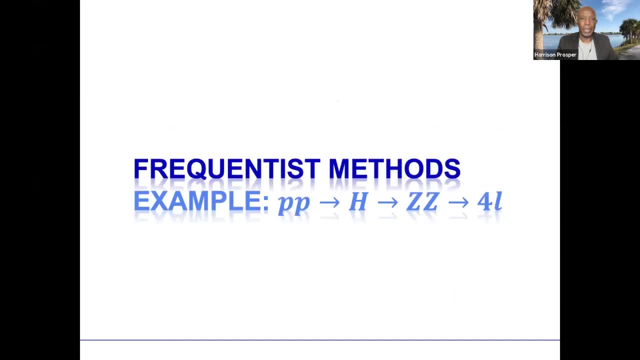 that fraction that you get is called the coverage probability, and the lower bound of that will be the contents level. So let's take a very simple example. We're going to look at this data that was published by the CEMIS Collaboration in 2014,, in which we looked for 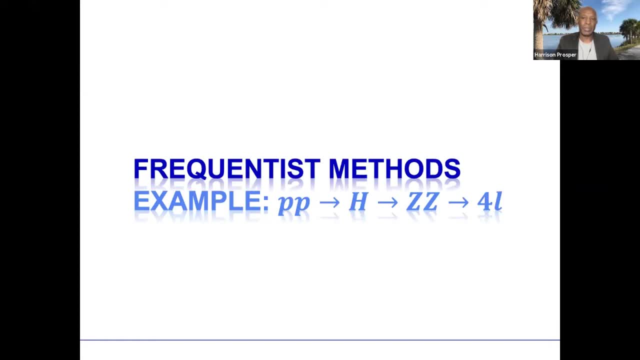 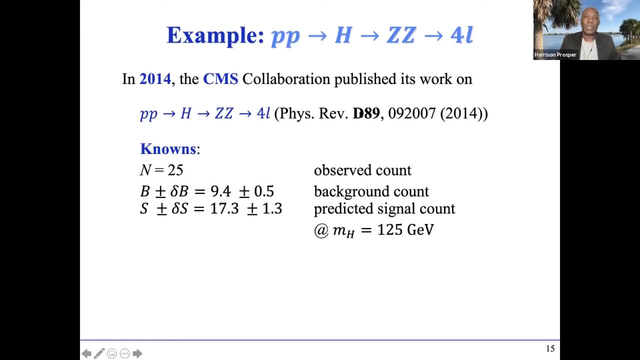 four charged leptons coming from the Higgs decay. So if you go and read this paper from CMS, you'll see that there are lots of numbers in that. but there's a summary which I've listed here that there were 25 events were observed. 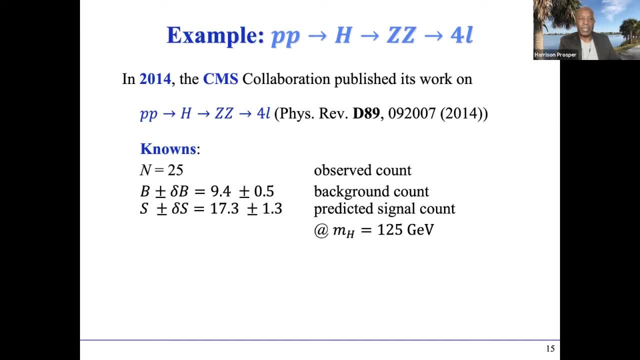 That's the actual number of events that satisfy all the selection criteria that we found. And then there was this estimate of the backgrounds coming from Pfeet going to ZZ and Pfeet going to Z-Boson, et cetera. 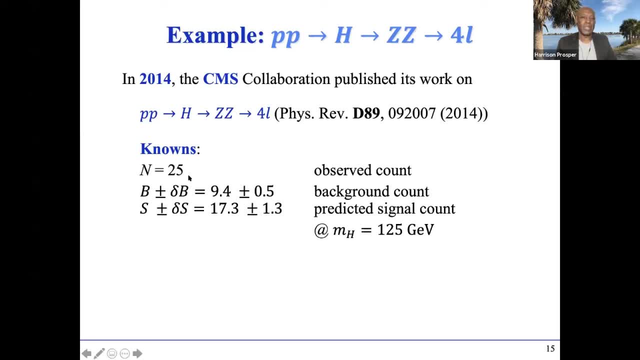 So all these backgrounds collected together and this was the estimate, that the background, plus some uncertainty in the backgrounds given by this: 9.4 plus minus 0.5 events. And if you go to your friendly local neighborhood theorist they will then predict that well, 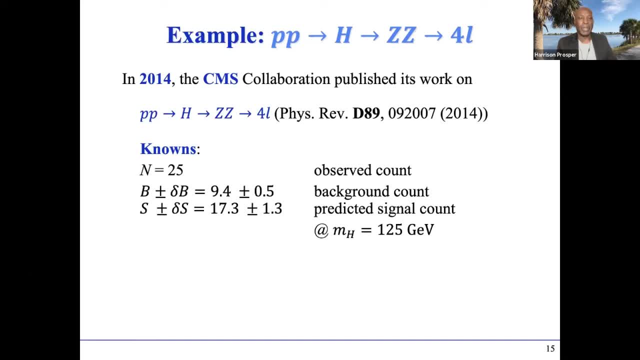 if the Higgs-Boson mass is 125 GeV, then in that experiment the expected signal according to the tunnel model prediction was 17.3 plus minus 1.3.. So these are the known things and these are the unknowns. 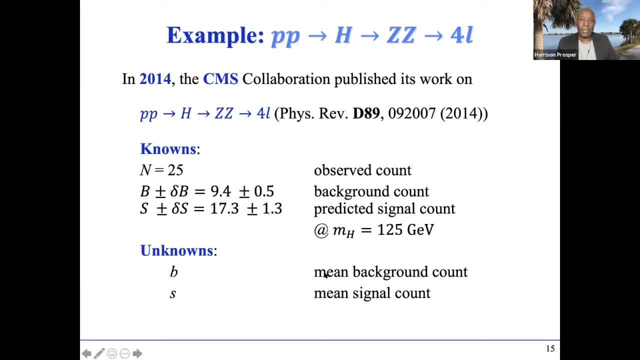 We do not know the mean background in that experiment, in that analysis, nor do we know the mean signal, And we shall never know these things right. Those are the unknowns, And we would like to say something about these unknowns. 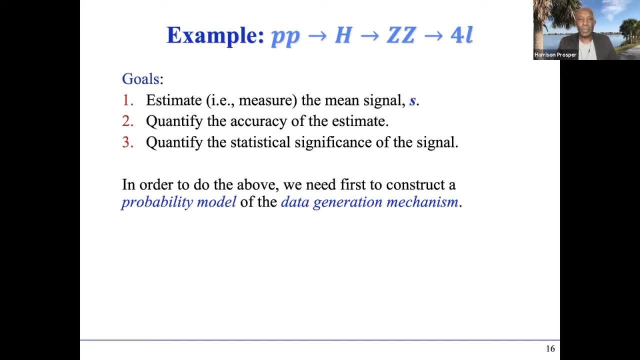 Well, actually, we want to make our goal somewhat more targeted. What we really would like to do is to measure or estimate the mean signal S right, Because if we know the mean signal S and we know the integrated luminosity, we can arrive at a cross-section. 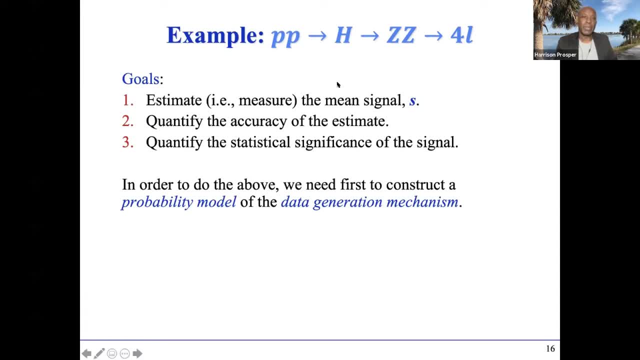 and that's something that is of interest to us. But, of course, just measuring, giving a number for the signal, is not enough. We all have learned from the very beginning, when we were young students, that you also need to quantify the accuracy of the estimate that you provide, right. 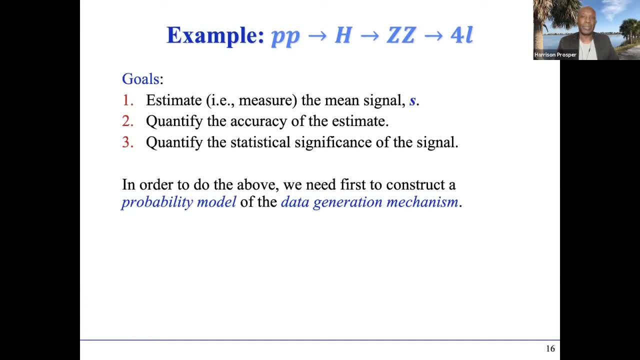 You must give some bound on the accuracy of your estimate. And finally, we'd like to ask the question: is there really a signal, Is there something that's significant that one should tell the world about? So those are typical goals that we have. 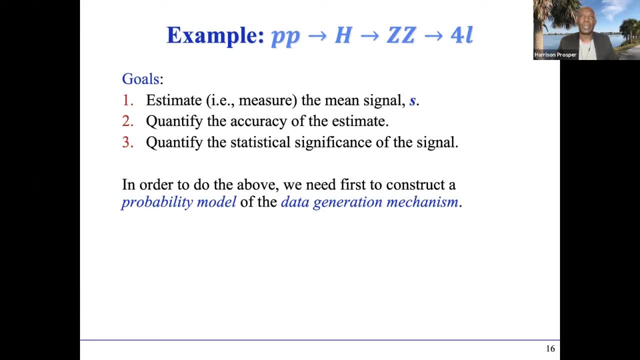 And we've just heard some beautiful talks on this goal, applied in the context of supersymmetry. right, We are trying to determine whether or not this hypothesis is true, And we do so by getting data, making measurements, And if we see nothing? 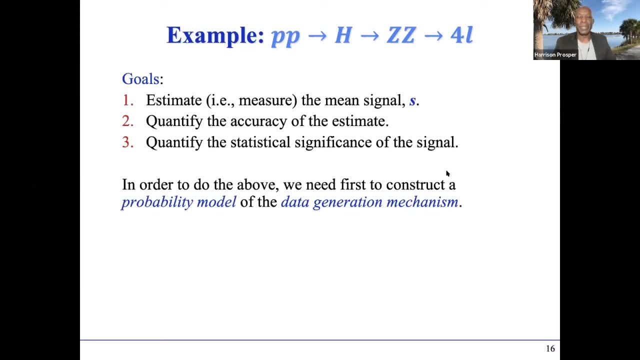 we then try to quantify the significance of the null result, But, of course, to do this we need to have a model of the data generation mechanism. and we need to have a model of the data generation mechanism. and we need to have a model of the data generation mechanism. 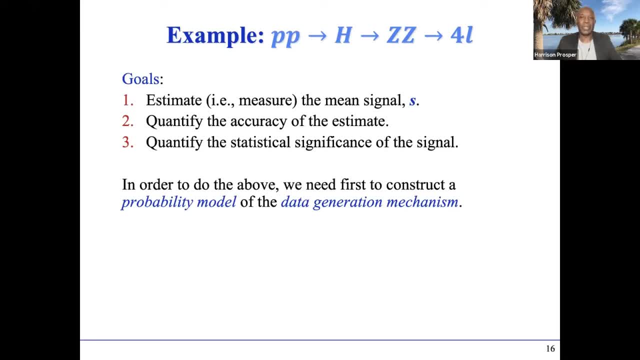 ie we presume that there is some mechanism that generates this data, the LHC right- Every collision is a perfect stochastic machine right. Every collision of protons, according to the quantum mechanics, generates this stochastic data, And we want to have a model of this. 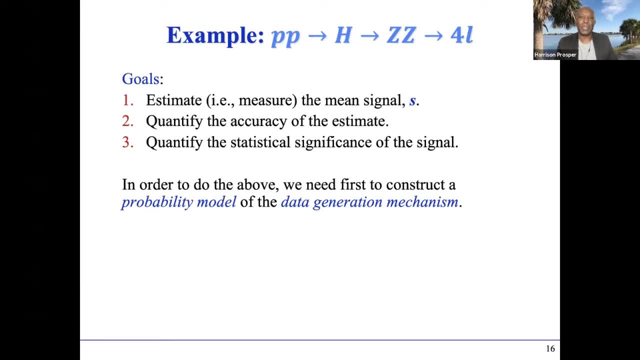 And given the model of that, then we can say something about the parameter S, which is the thing of interest to us. But let's start from scratch. Since these are supposed to be pleasurable talk. I really want to start from scratch. 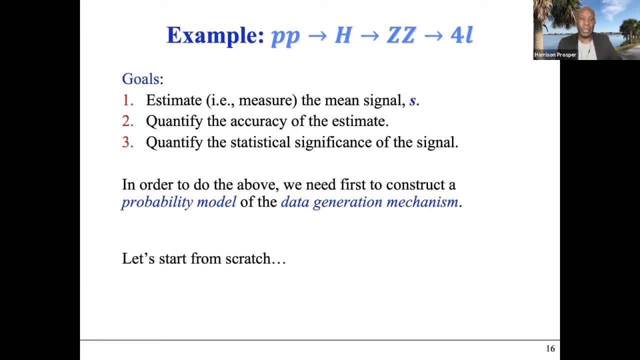 because, in principle, this is what one should do: One should really think very hard about the data that you have acquired in order to be able to construct a probability model of the data generation mechanism. Now, of course, we already know what the answer is. 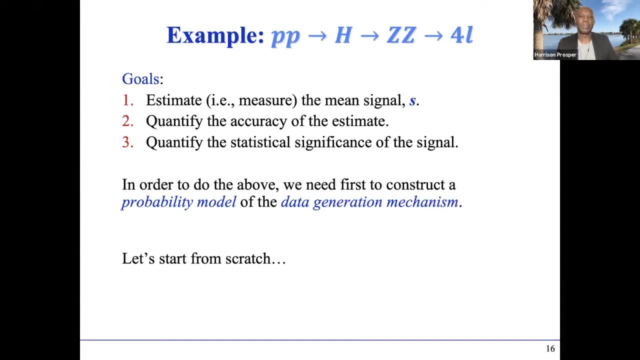 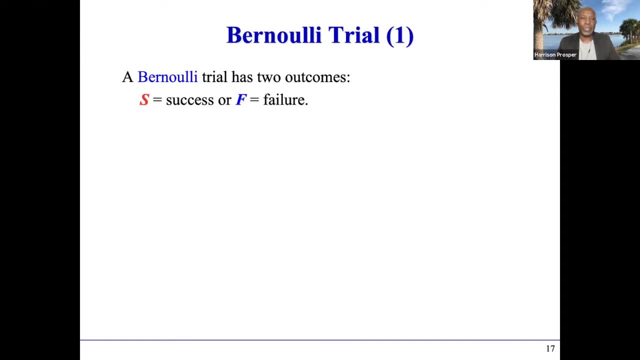 The answer is going to be a Poisson distribution. Let's start from the very beginning. So imagine that you divide what happens when two protons collide into two classes. There's a success and there's failure. So let's say, you know, two protons collide. 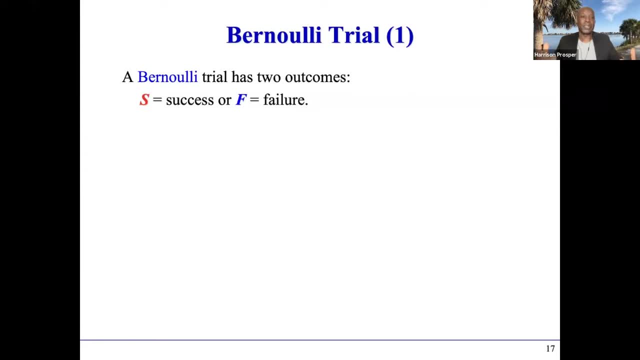 and there's a success. Maybe one day, the creation of a SUSY particle or perhaps creation of a Higgs boson, that would be a really, you know, that's a success, And the failure to create a SUSY particle or a Higgs boson particle would be, let's say, a failure. 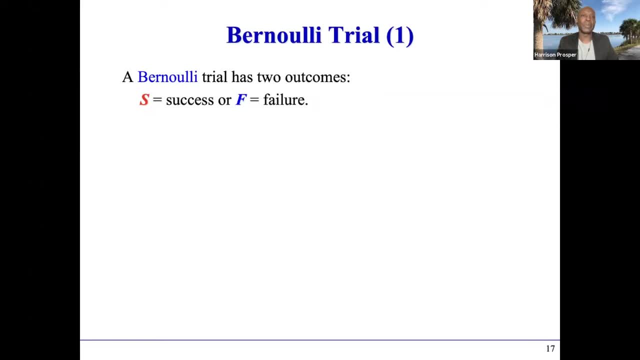 So there are two outcomes, and this is the nature of a Bernoulli trial, And the LHC is just a fantastic. in fact, it's probably one of the most extraordinarily beautiful examples of Bernoulli trials, where we attempt to make each trial the same right. 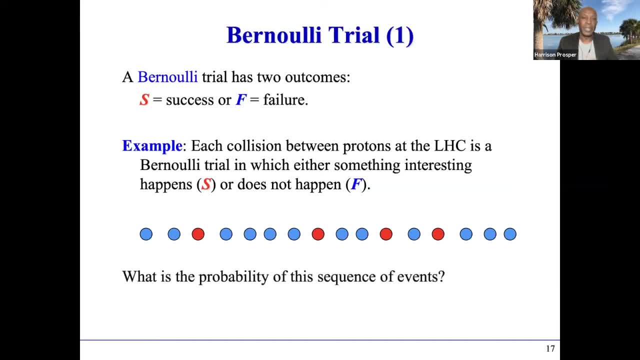 And there are successes and failures. Now here's a question: What is the probability of the sequence of events? Well, the answer is: there is no answer. It is not possible to proceed without making assumptions And, of course, if you make different assumptions, 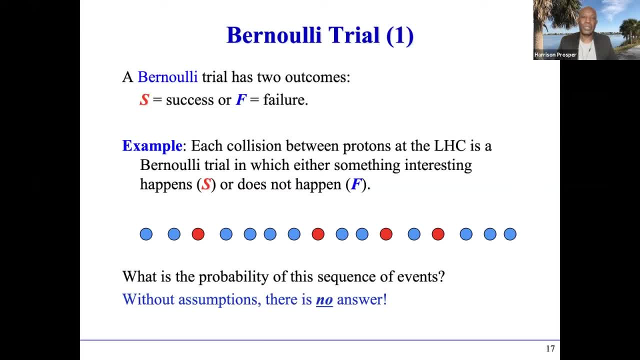 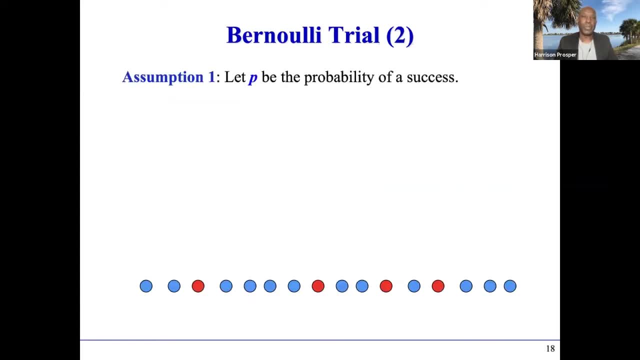 you'll get different answers. So there really is no answer to this question, unless you're willing to make some assumptions. So let's make some assumptions. The first assumption: we're going to assume that the probability of a success is P. Okay, that seems like a reasonable thing to assume. 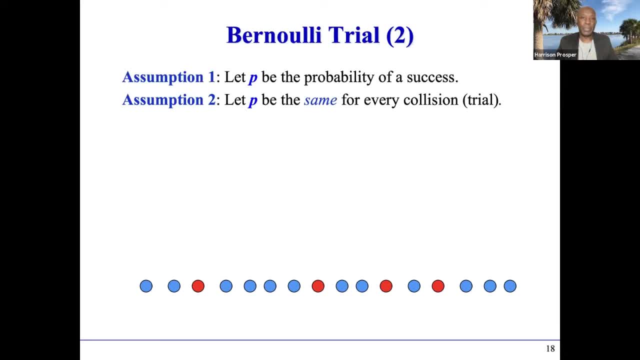 The second assumption. we're going to assume that the probability of the success is the same for every collision. So every proton-proton collision, the probability of a success- let's say the creation of a SUSY particle- is the same. That could be wrong. 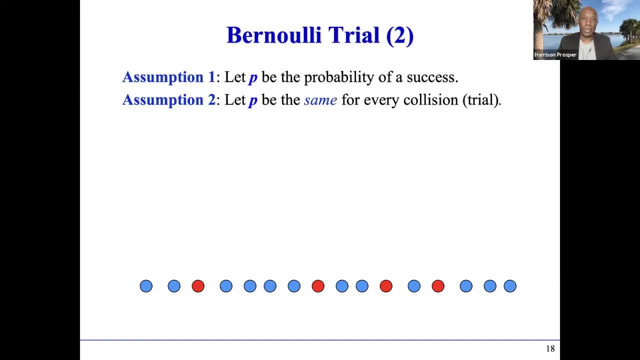 Of course that could be a misguided assumption, but that's the assumption we're going to make. We should assume, which seems reasonable, that creating a SUSY particle and not creating a SUSY particle, these are mutually exclusive events. If that's the case, 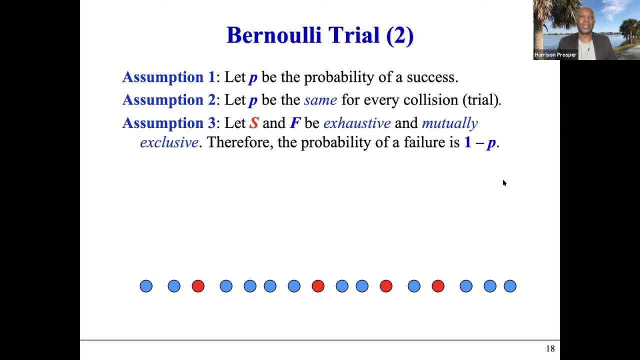 then the probability of a failure is one minus P, because there are no other possibilities. Okay, so here are our assumptions, And those three assumptions are now sufficient for us to write down the probability of a particular sequence. It's just going to be P to the power of K. 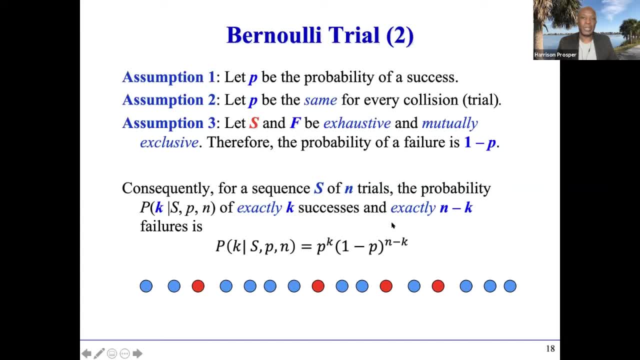 if there are K successes, exactly K successes, and one minus P, N minus K if there are exactly N minus K failures. So okay, we succeeded, given our assumptions. Now let's say assumption two were wrong. Let's just say in some sort of random fashion: 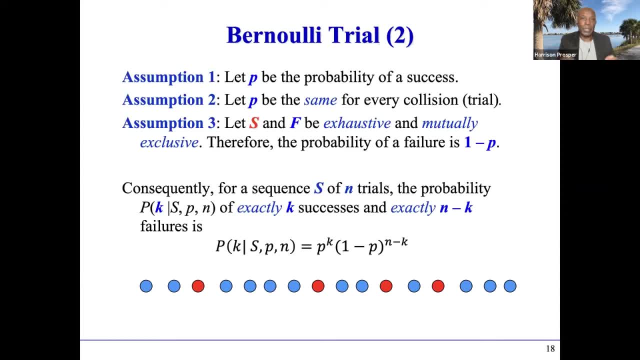 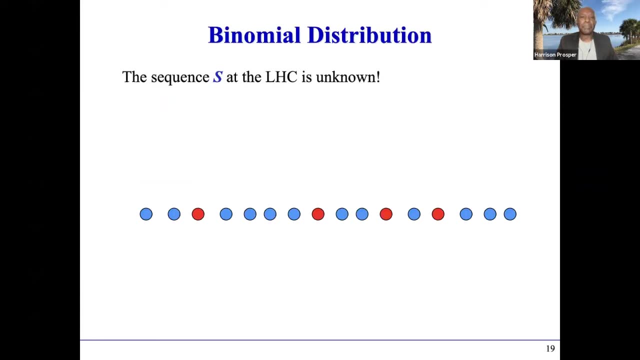 the probability of a success for every proton collision just changed, Then of course, this would be a much more complicated expression than this, But given those assumptions, that's the probability of that sequence. Okay, so that's progress, But unfortunately, though, here's the problem. 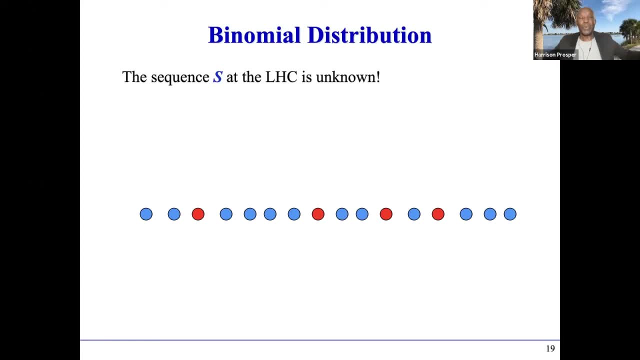 There's now been this long sequence of collisions at the LHC, but we don't know which ones. which of these collisions really is a success, which one's a failure. We have a good reason to believe which events might be: Higgs, boson events. 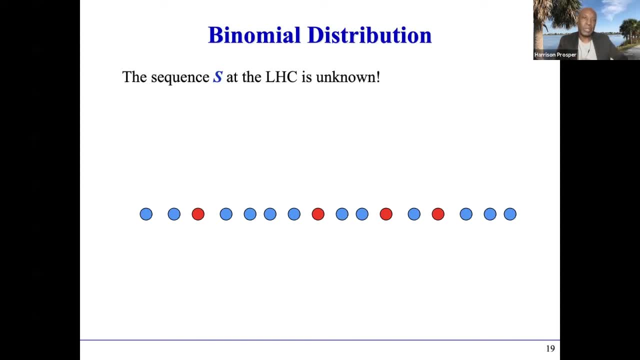 but we don't actually know, And so since that sequence is unknown, then we need to somehow do something about that. So what does one do? Well, if you go and look up your books on probability theory, it tells you. they tell you that the way, 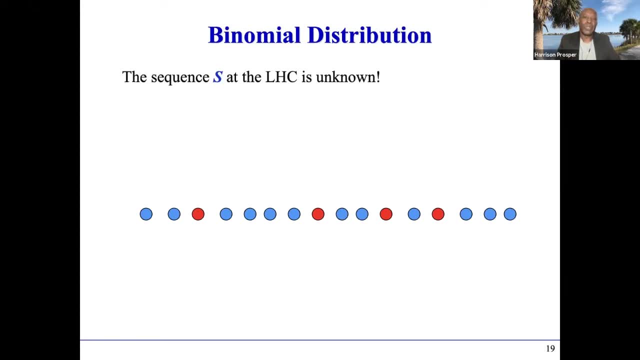 when there's something in your problem about which you are either clueless- you have no idea about this- or it's a parameter that is not of interest to you, then what theory tells you you should do to eliminate that particular quantity? is which, in this case, the sequence? 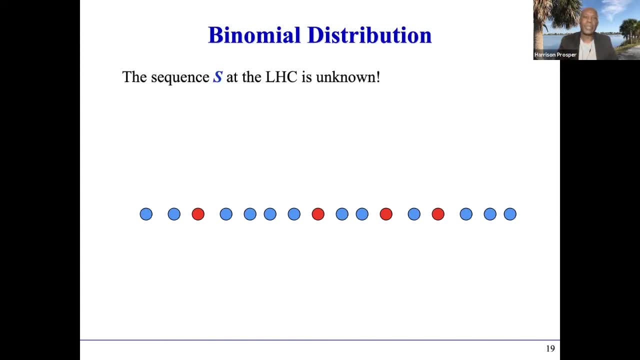 is to simply sum over, to integrate over the things that you don't care about, And so let's do that. Let's simply sum over all the possible sequences in which there are K successes and there are N minus K failures, And that's what we've done here. 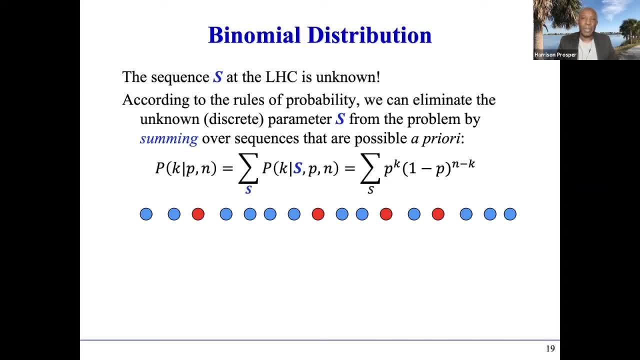 Okay, Now, now we have to make another assumption, That's number. now, assumption number four: Let's assume that each sequence where you have the same number of successes and the same number of failures, let's assume that each sequence has the same probability. 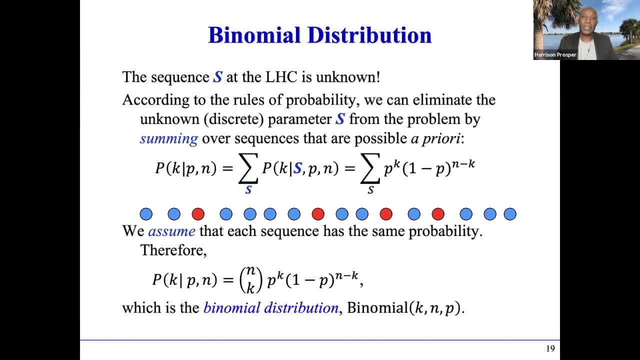 That may not be true, but let's assume. then, If that's the case, then of course the number of terms in the sum is just N. you know, choose K and low, and behold, you arrive at the binaural distribution. 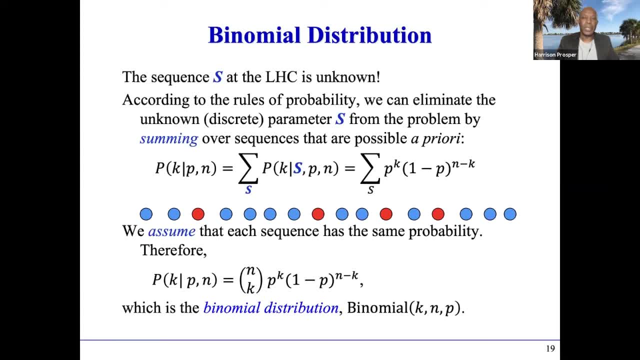 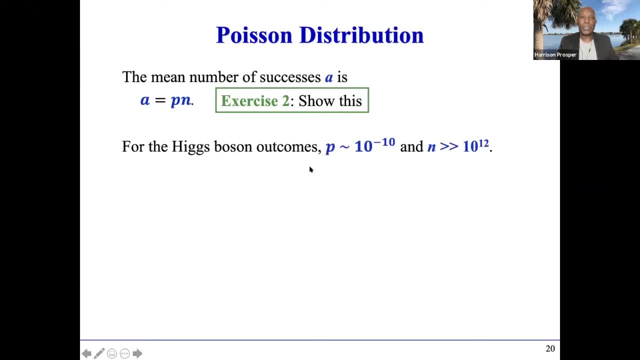 given those four assumptions. Now, of course, it would be insane to use that distribution for the LHC right. why? because the probability for creating a Higgs boson is, of all, the 10 times 10, so it's very, very small and the number of collisions is trillions. 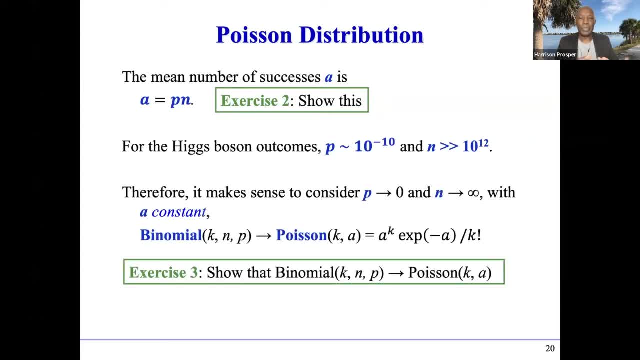 So it is completely reasonable to take the limit that p goes to zero and n goes to infinity with, say this, product constant, And if you do so, of course you arrive at the Poisson distribution, which is, of course, the distribution that we all use for a counting experiment. 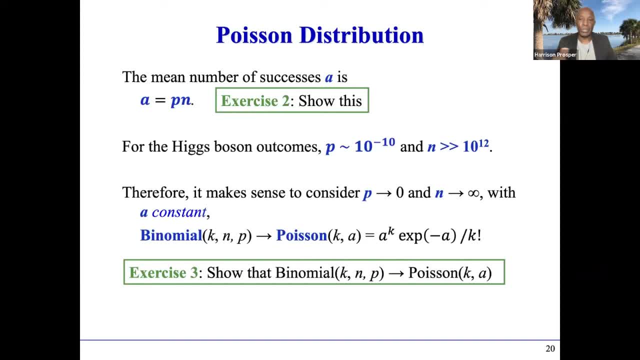 Of course, you can derive that distribution in many other ways. For example, you can use some sort of stochastic modeling and you get to the same point. The point is this: is that that distribution, there are assumptions that underlie it that we think are reasonable, and that is why we use it. 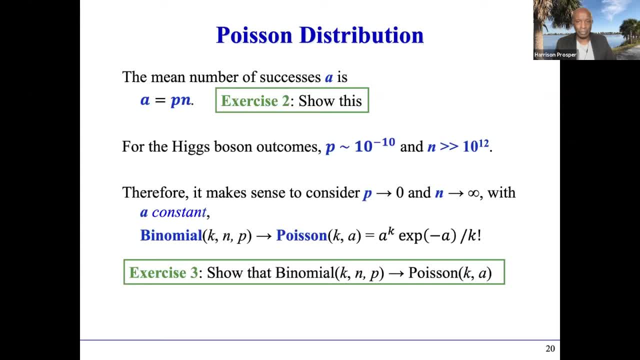 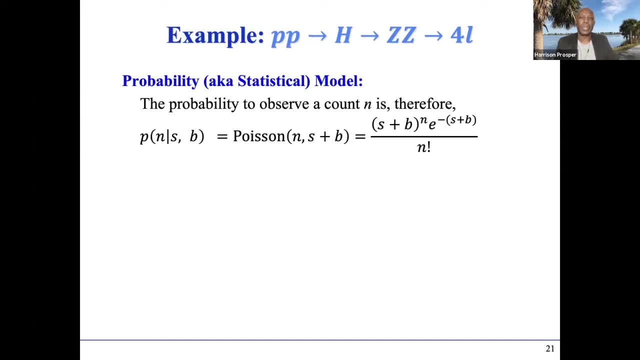 And we have seen that we arrive at results that make sense. Okay, so we have agreed that the Poisson distribution is what we should be using, and so let's go back to this data then. So here is the probability model. It's just some of the signal-pushed background, because we assume that these are not interfering and they're additive, and that's it. 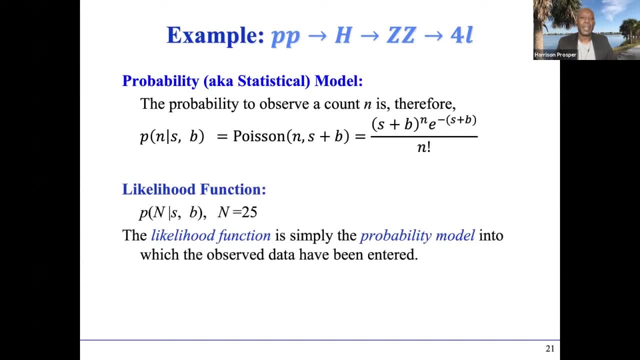 So we have our model, Okay, and now we're going to plug in to our model the actual distribution And we have the actual data we have acquired. So in this case, there's only one datum, which is the count of 25 events. 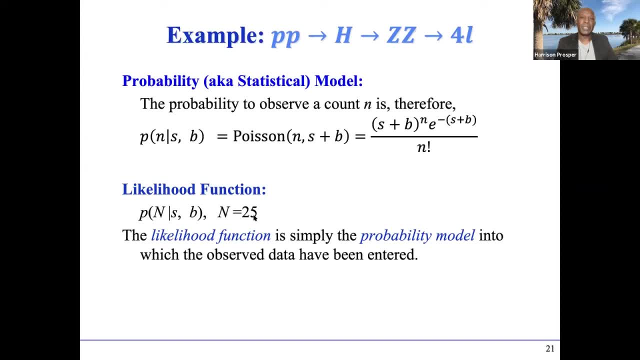 And once you've done that, once you've plugged in the data into the probability model, the statistical model, you then arrive at what's referred to as likelihood function. And so, again, going back to the Higgs combination between ATLAS and CMS, this is gigantic, very, very complicated probability model that's been constructed by the two collaborators. And so, again going back to the Higgs combination between ATLAS and CMS. this is gigantic, very, very complicated probability model that's been constructed by the two collaborators. And so, again going back to the Higgs combination between ATLAS and CMS. this is gigantic, very, very complicated probability model that's been constructed by the two collaborators. 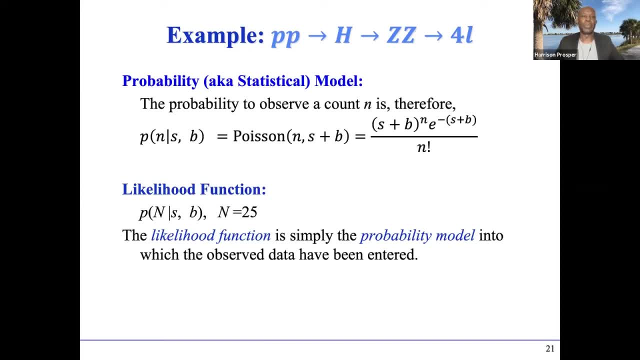 And then one plugs in the data into these models and one arrives at a function that's called the likelihood function, which, given that the data are constants, can be regarded as a function of the parameters of the problem, In this case the mean signal and the mean background. 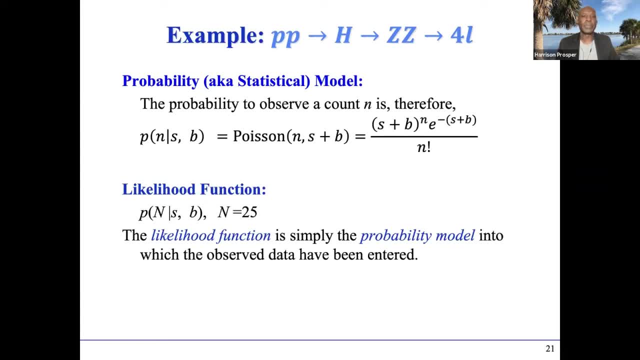 Okay, so we now have our likelihood function, But we notice that there's some extra information that we have. We also have an estimate of the background. right B plus or minus delta B is 9.4, plus or minus 0.5 events. 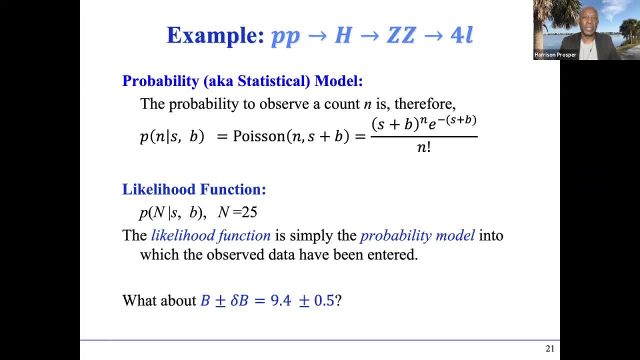 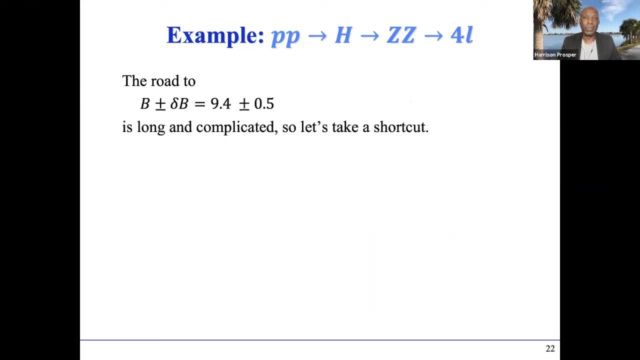 So how do we incorporate that into the problem? That's clearly something that's of interest to do because it's useful information. Well, if you read the paper from 2014, you'll see it's a long, complicated road to arrive at the likelihood function. 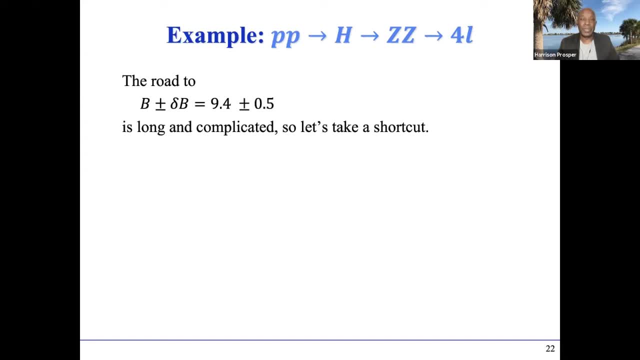 So you can see that it's a long, complicated road to arrive at the likelihood function, But we're going to take a shortcut. We're going to take a shortcut because we want to keep things, We want to simply focus on the essentials. 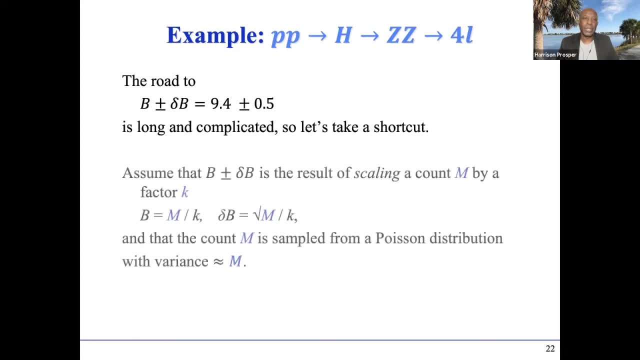 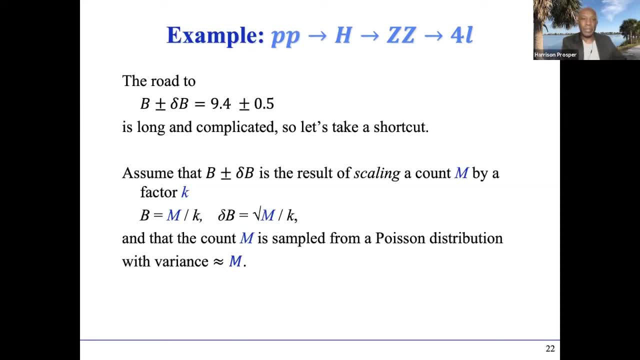 So imagine that you have this fabulous Monte Carlo simulation of the experiment CMS in this case. So imagine that you have this fabulous Monte Carlo simulation of the experiment CMS in this case was applied to the real data, and let's suppose I get m counts. Well, I'm then going to scale. 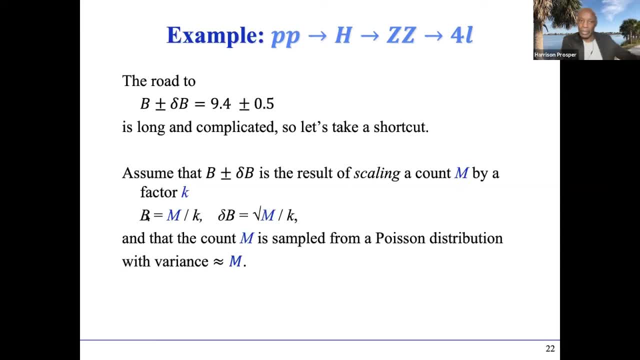 m by k to get the background estimate in the real data. and then I presume that, well, m is from a Poisson distribution and we all know that the standard deviation of a Poisson distribution is square root of the mean. so we're going to assume that delta b is equal. 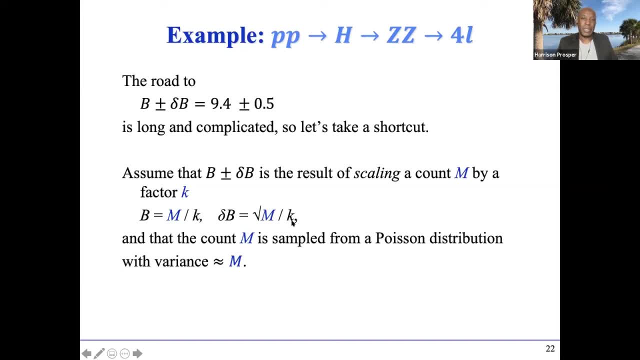 to square root of m divided by k. All right, so that's our shortcut. Of course, in reality, as I said, this is quite a complicated thing, but this is actually a reasonable mock-up of what actually was done. Okay, so if we do that, then of course you can just simply. 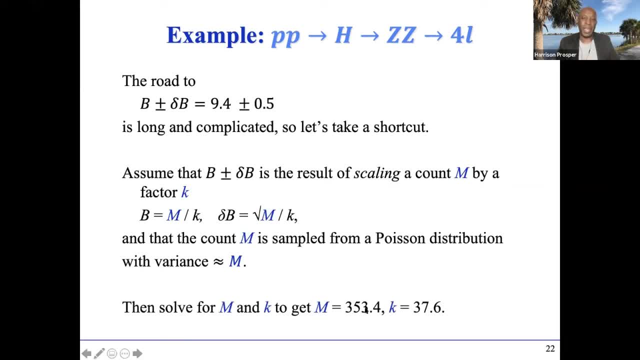 invert these equations to arrive at the effective counts, and so what this tells you is that, if to arrive at this background estimate, it would be equivalent to running a simulation in which and you apply selection criteria to your simulated events and you then arrive at 353 events, past all the cuts, all the selection criteria, and you generated. 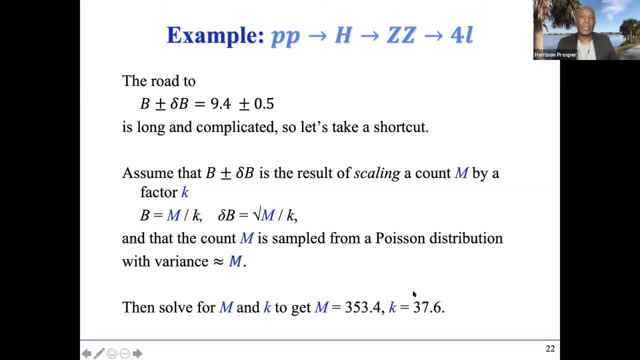 so many events that you have something like 38 times more integrated monosity for the simulation compared with the real data. Okay, so we now have the effective count and the scale factor And, of course, if the scale factor was not precisely known, then of course you could add. 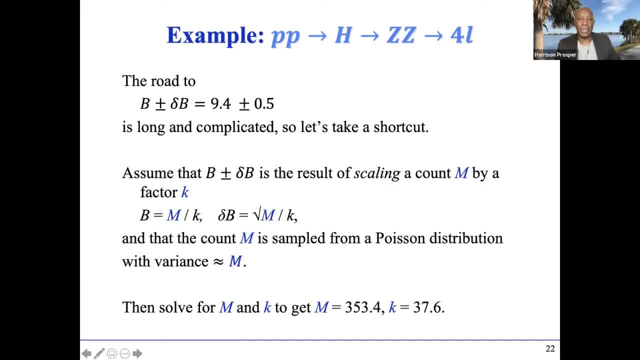 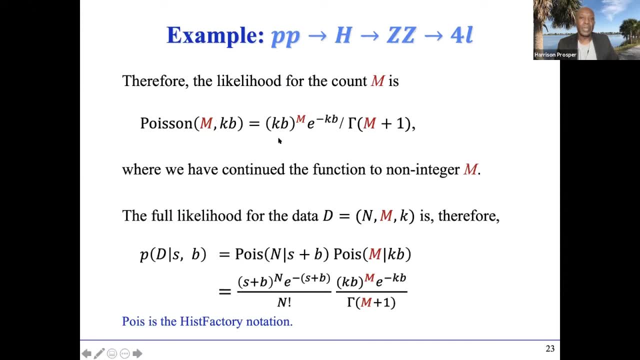 more complications to take that into account and so on, But let's keep it simple. So, now that we have these two numbers, we can then construct the Poisson distribution. Now, because m is not integral, right in this case, then I've just simply used the trick of replacing the n factorial. 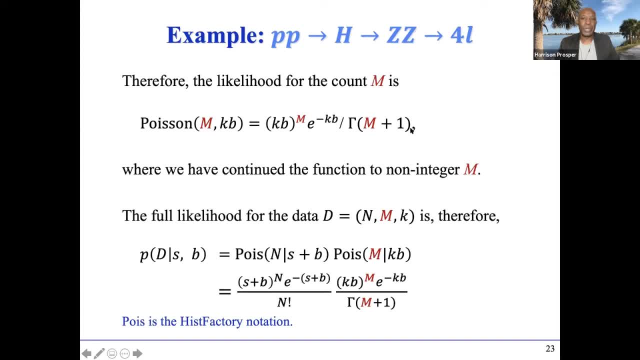 here by the gamma to make this all work. So, now that we have this, we can now construct our full model, which is just the product of the original piece that we talked about. By the way, I'm using now I'm using Poiss is the if you go. 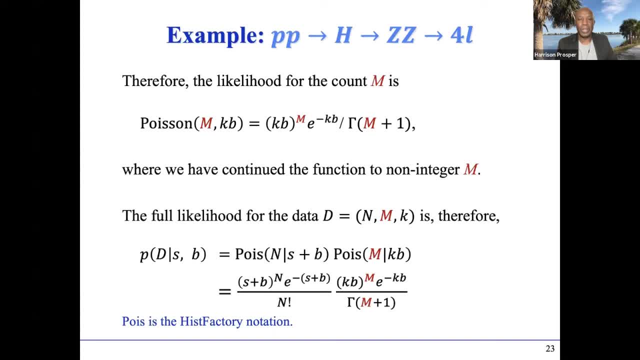 and look at the HisFactory documentation on the web, then you'll see that they use this notation. So I'll use this notation in case one of you decides to go off and try out PyHF or one of those other programs. And so now we have two pieces. We have this Poisson distribution that pertains to the 25 events. 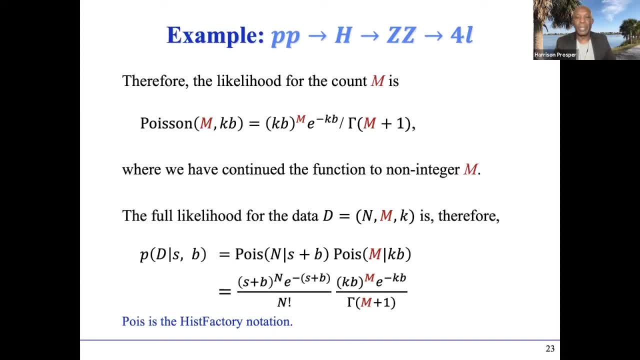 that were reported by the CMS collaboration, And this is something we constructed based upon our shortcut to get back at the effective count from which the estimate in the background was derived, And so here is a full-blown likelihood function And, as I mentioned, suppose that this factor 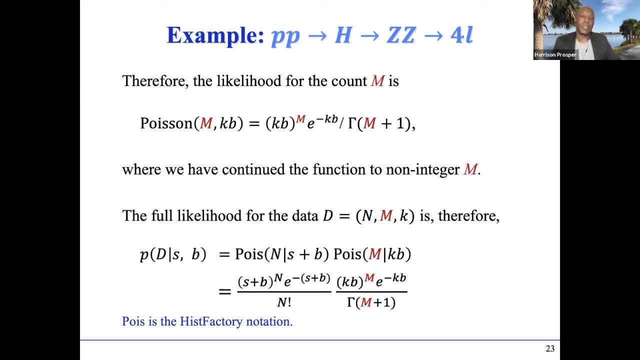 k was not precisely known. Supposing there was some uncertainty in k itself, then of course one would simply multiply this function here by another function that accounts for the uncertainty in k, And so it goes. So now that we have this, we can now proceed to our task of trying to say: 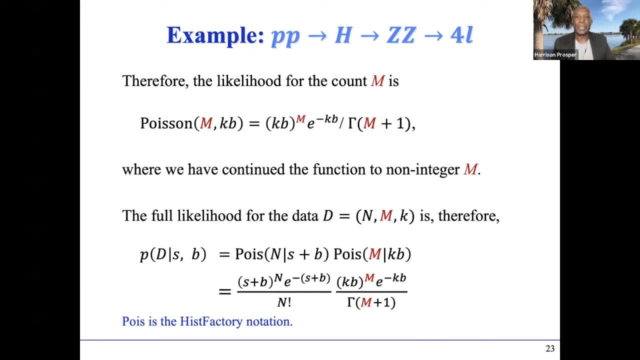 something about the mean signal in this particular experiment Before I move on. are there any questions? Is there a plus or ego after the begin? It's okay, Hafiz Ali, I don't see a mean. Okay, just a simple question. Why is there a plus 1 in the denominator with the M and not just M? 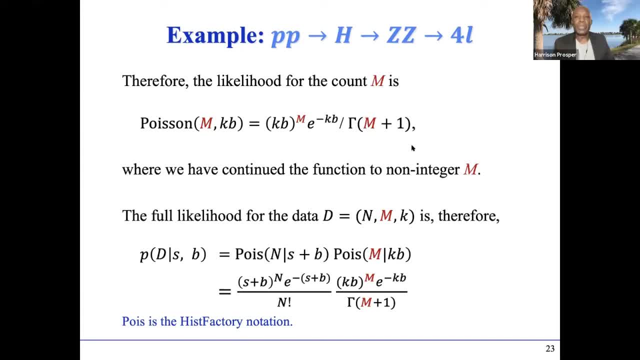 Oh, so, so ordinarily this would be, this would be M factorial right. Yes, And so M plus one of …. Oh, M plus 1, or gamma of M plus one, is that the Jews have the M factor and they haven't ever beenraried up either. They might find this significant. We have so many, so many reasons, So why theymphine itself …. Well, M is a very, very significant binary recognition. Some, many times, it was some of the equations for chemical regression: Estamos y waves …. 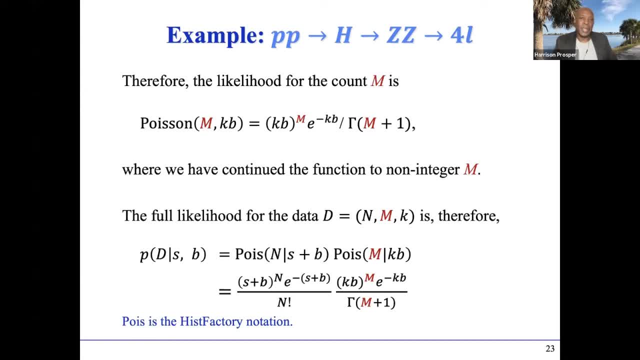 200,000 times. So only the word geribride is a number, And so … well … m factorial and not just gamma, Yeah yeah, And of course I could not use m factorial because the m was non-integral. although that's a detail, This doesn't actually make any difference to the 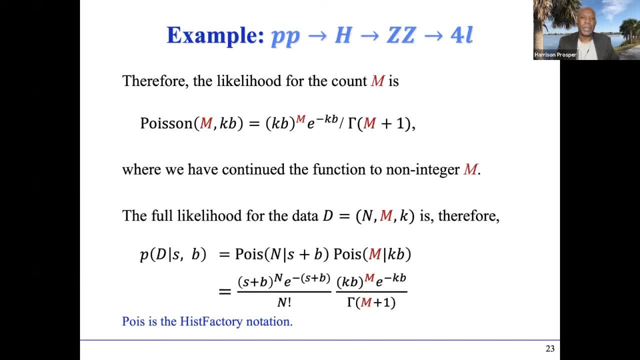 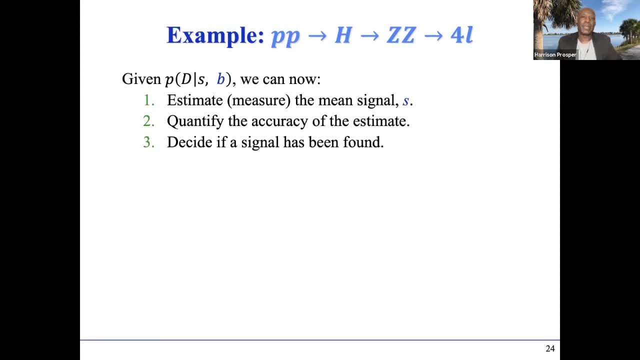 inference. Okay, thank you, Thanks. Okay, so we now have our likelihood, And the only difference between what I've just done and what's done routinely by ATLAS and CMS and the other LHC experiments is that, of course, the functions that they arrive at are far more complicated, because, 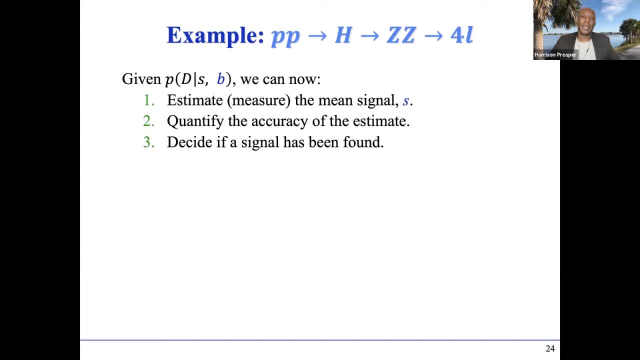 they've got to take into account many things. For example, you may find that you've got to take into account the fact that the trigger efficiency in the simulation doesn't quite match the trigger efficiency in the real experiment and therefore you have to have some scale factors to correct. 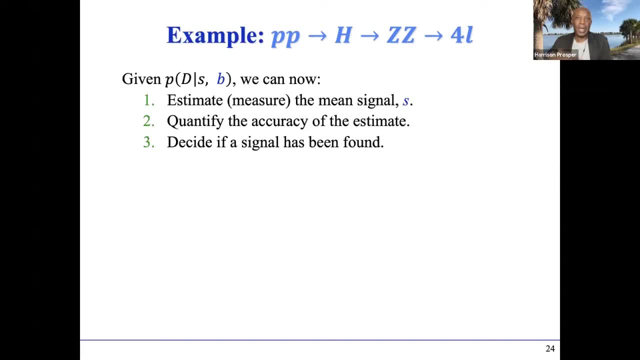 for the efficiencies. But then of course those correction factors are themselves uncertain and therefore you've got to take into account uncertainty in these correction factors and so on. For example, let's suppose you're doing analysis. where you're looking you have jets in the event, For example. 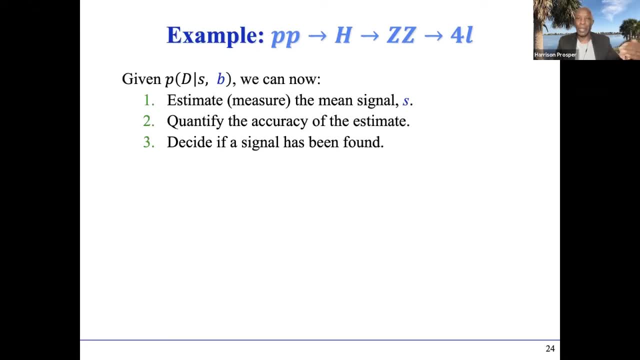 you may be interested in trying to look for vector-bottom fusion events relative to ground fusion events in the Higgs sector. Well, there are jets. Well, jets, of course we measure them with some uncertainty and we scale the measured quantities for, let's say, the transmittance. 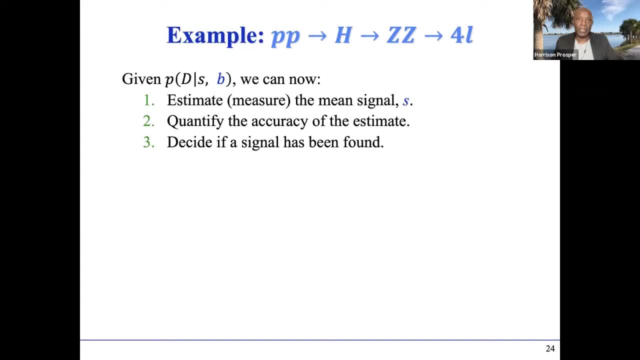 of the jets, so that on average the PTs of the jets, the transmittance of the venter, agree with the venter of the jets prior to entering the detector. But then of course these corrections are uncertain, and there too one has to take into account the uncertainty That's another term, and so on. 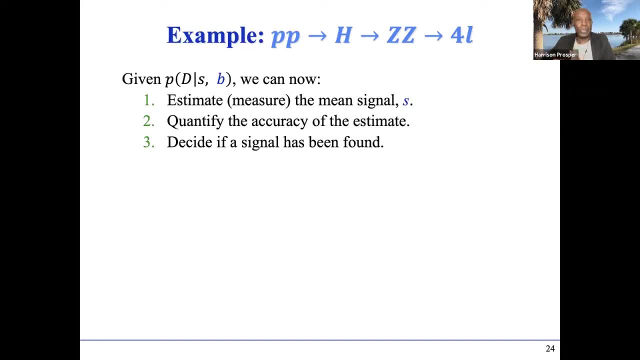 So as one goes through step by step, trying to understand where all the uncertainties arise in the analysis, then this simple function that I wrote down gets progressively more complicated as you're taking into account more of these details into consideration. But fundamentally, it's the same problem that we're addressing right now. 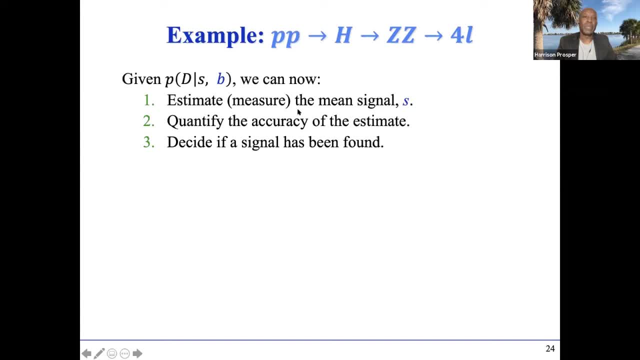 So we have this function and now we can measure the signal in principle. from it, We can quantify the accuracy of the estimate and we can decide, you know, is there a signal or not. And those are the key things that we want to do as particle physicists. Now, in our field, the basic standard, 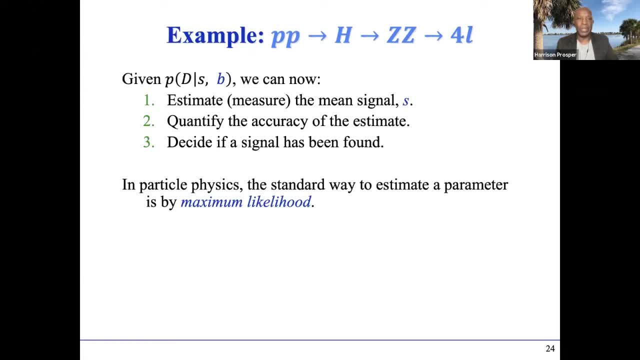 way to estimate the parameter- and that's not just in our field, but many other fields- is by maximum likelihood right. This is the method that was actually first used by Carl Frederick Gauss- of Gaussian fame and many other things, of course- and popularized. 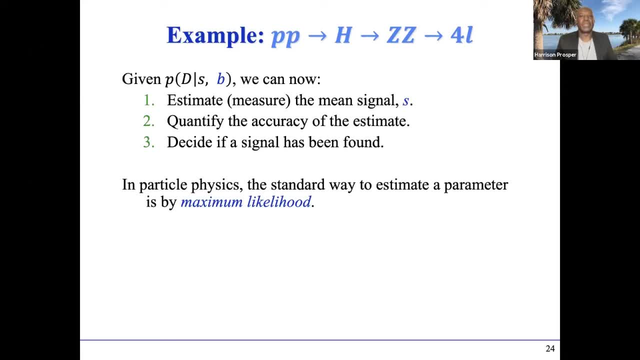 by Ronald Fisher in the 1930s. And basically it just simply says: I have this function here, I simply maximize it with respect to the parameters of interest and that gives me an estimate of the particular parameter of interest. But unfortunately there's a problem. 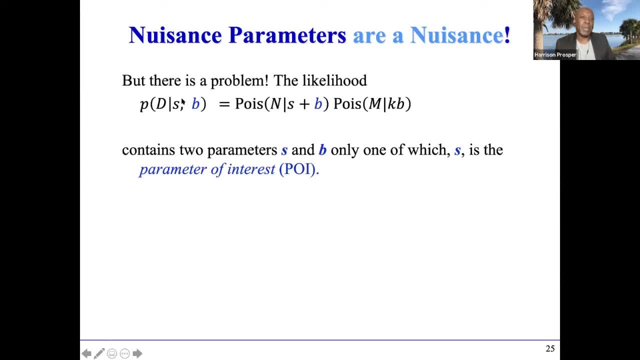 because I we only care about the signal, We don't care about the background. The background is necessary, of course. that's part of the model, that's for sure. We can't simply ignore it. But that's not what we care about. We only care about the signal, the so-called parameter of interest. 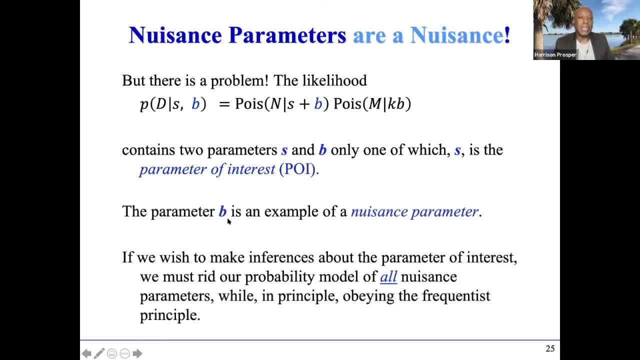 Well, in this context, the parameter b is an example of a nuisance parameter. Why nuisance? Well, because they really are. these really are a nuisance and, in fact, a huge amount of work has been done over the years trying to find ways to get rid of these parameters in a way. 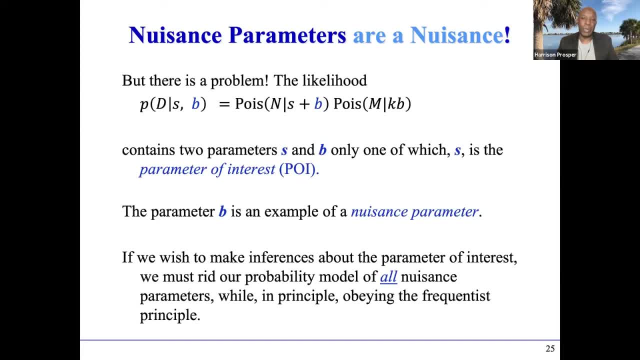 that preserves the so-called frequency principle. That's the goal. You want to get rid of this parameter. And now, in these models that are used at the LHC, there are literally hundreds of such parameters, And no doubt in the era of the high-lunosity LHC, as our analysis become more. 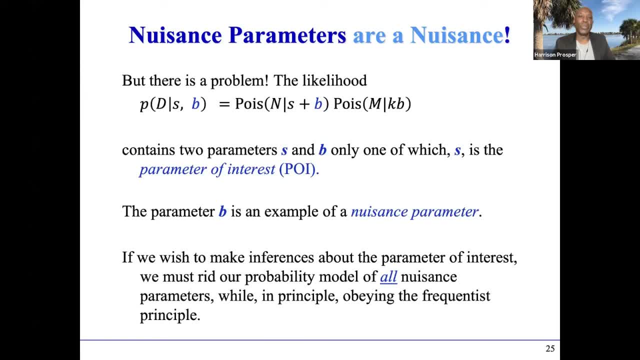 and more sophisticated as we venture into looking for new ways of looking for new ways of looking for SUSY, for example, you could merely imagine. the number of parameters that we need to get rid of could number in the thousands. So one has to get rid of all these parameters somehow, while still 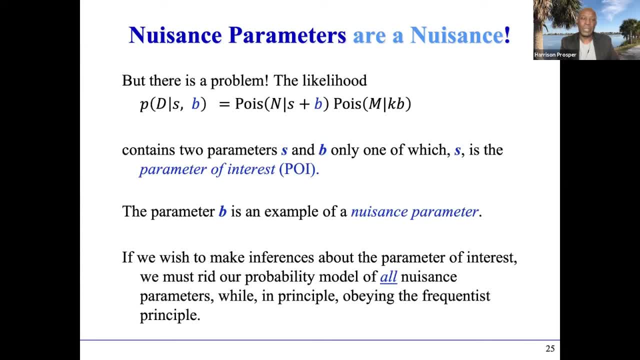 preserving this principle, this frequency principle, That is, you want to write statements such that if you were to repeat that procedure many, many times on different experiments, then some fraction of those statements you're guaranteed to be true. That's the goal. 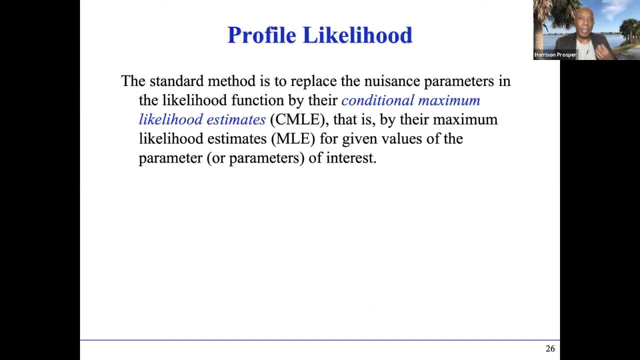 So let's see how that's done. Well, just as the maximum likelihood is the standard technique for basically writing out an estimate, the basic technique for getting rid of parameters that you don't care about is to basically replace them. So, in our case, replacing b by the conditional maximum likelihood. 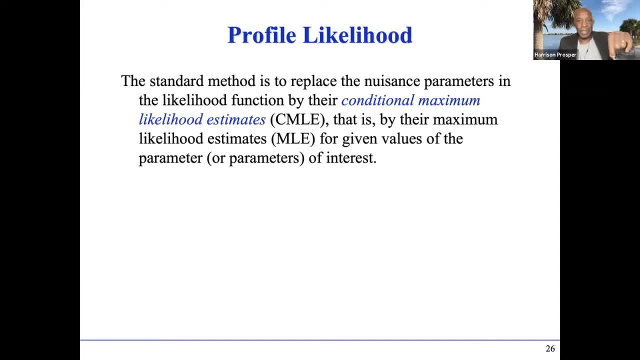 estimate. So what does that mean? Well, it means that you keep Sfix the signal and you maximize respect to all the parameters that you don't care about, that you want to get rid of so called nuisance parameters, And that's it. You maximize respect to all the other parameters, you change the value. 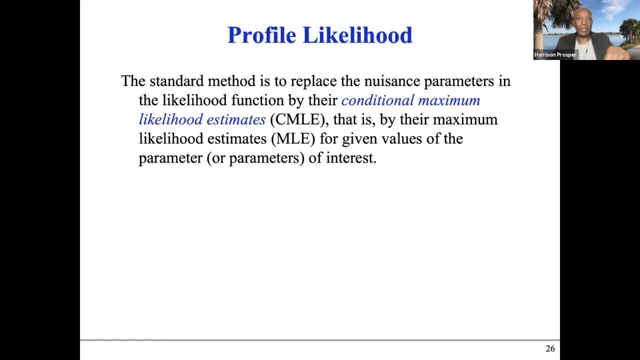 of S, you maximize respect to all the other parameters and so on, and that way you sort of map out a function that depends ostensibly only on the parameters of interest. So that's what we're gonna do. That function that you write, that is called the profile likelihood. 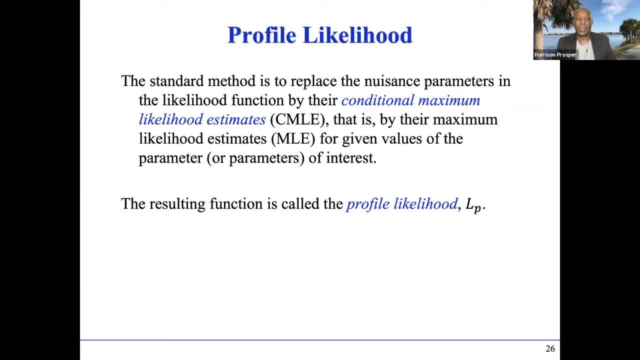 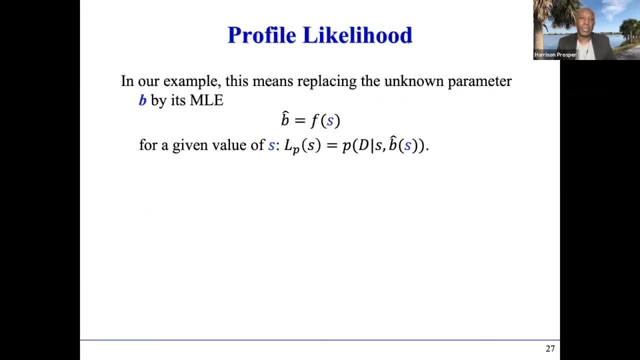 And that is something that's been used in particle physics, you know, for decades. So there's nothing new here. So we have the profile likelihood. So what can you do with it? Well, as I said, this is what one does. So here is the original likelihood and we simply replace b- the unknown. 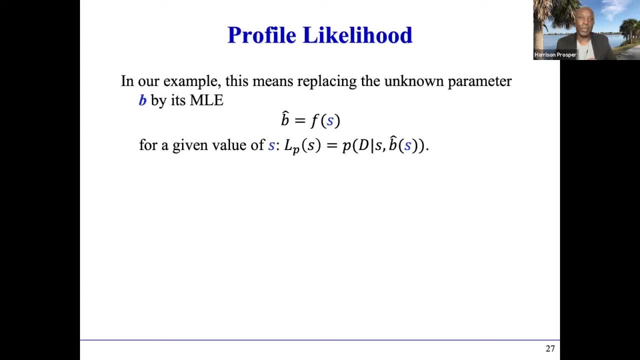 the true, unknown, mean background which we'll never, ever know. because we're not privy to such information, we're going to replace it with an estimate thereof. This estimate depends on the particular choice of the value of the signal s, And so, if you look at this function, this looks to be. 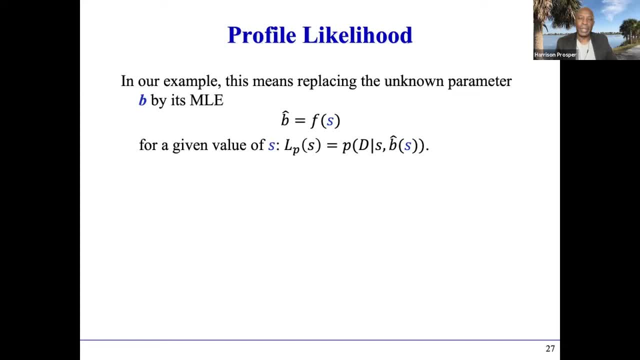 a function simply of s, and that's called the profile likelihood, And that's the standard technique that's used in particle physics. Now, obviously, if I replace a true thing by an estimate thereof, then that is obviously an approximation right? We're doing something. 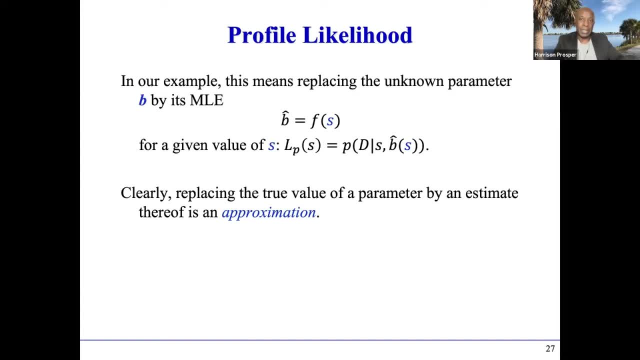 not quite right. We're replacing something that we don't really know by our best guess, our best estimate of that thing, That's an approximation. Well, the point is that it's an approximation and therefore this principle that was written down. 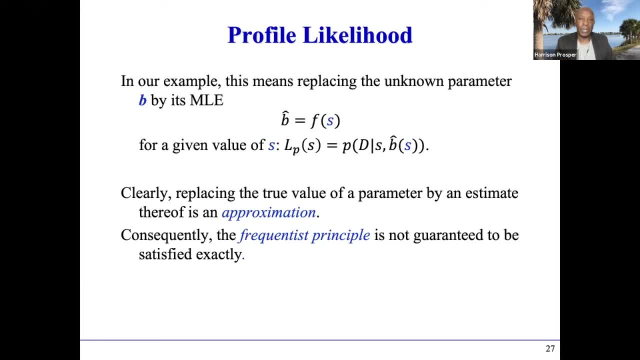 by Neyman way back in 1937, well, there's no guarantee now that it's going to work exactly. It's going to be exactly satisfied, right? You may apply this procedure many, many times and then discover that you say, oh, I have a 68% interval, or I have a 95% limit, but in reality, 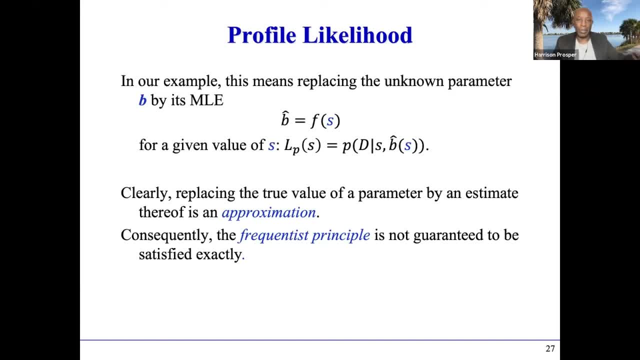 it turns out to be 86% right, And that would mean that your procedure is not satisfying this guarantee, this frequency principle, Because, after all, it's an approximation. However, the good news is that it turns out that this procedure, this approximation, has a very sound justification, which is, of course, 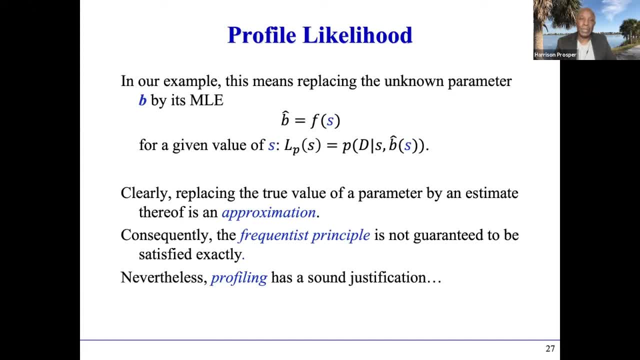 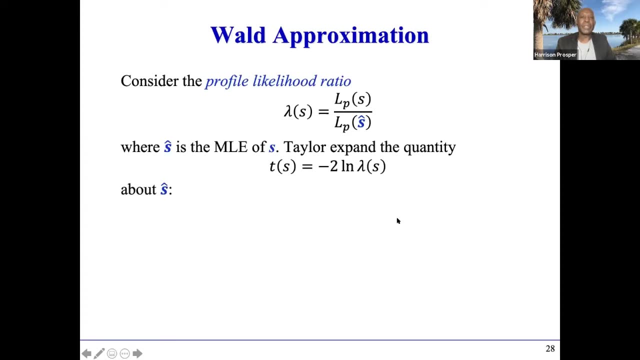 why it is used routinely, right? I mean, there's no way we can get around it. That is what we do, because that's the standard technique that's very generally applicable. So why is this a reasonable thing to do? Well, let's consider the ratio of. you know this ratio here. So in a numerator, 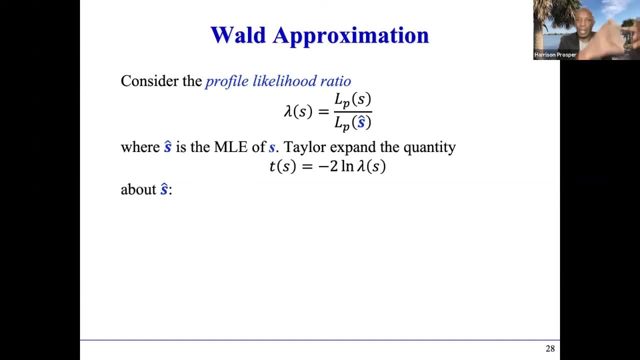 we have the profile likelihood And remember that is just our likelihood function, where we simply maximise respect to all the other parameters of the problem. There could be hundreds of those- for different fixed values of, in this case, the signal And the function. 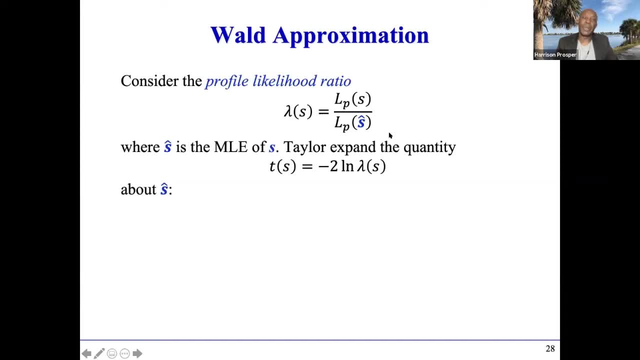 in the denominator is the same thing as in a numerator, but now we're going to maximise respect to, in this case, the signal. So it's the. it's the profile likelihood as a function of s divided by the profile likelihood at its maximum value. 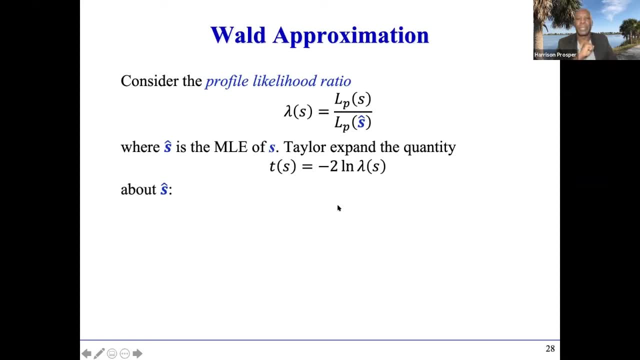 Okay, So we consider this, this quantity, here And now let's consider the negative twice log of this ratio. I'm going to tailor expand that about the estimate of the signal s hat. Okay, So we just do a tailor expansion. Here, we, there we go, And then you, you, you, obviously the first. 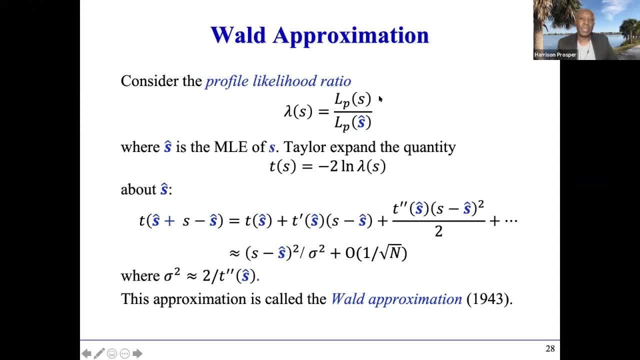 term disappears Why? Well, because if I replace s here by s hat, I get one. Well, the log of one. well, we know what? that is right, So that disappears. And likewise, this term disappears because these are the maximum likelihood estimates, And so this is going to be zero, And so 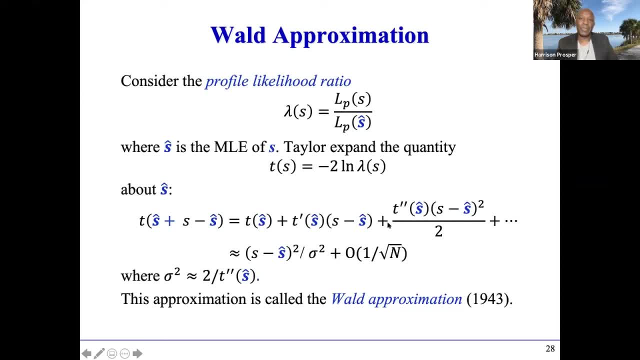 So the only term, the first non-trivial term, is this quadratic term here And of course you have terms that you can show are rather 1 upon the root n, And this approximation to this statistic, as it's called, is called the Vald approximation that was specified by Vald way back in 1943.. 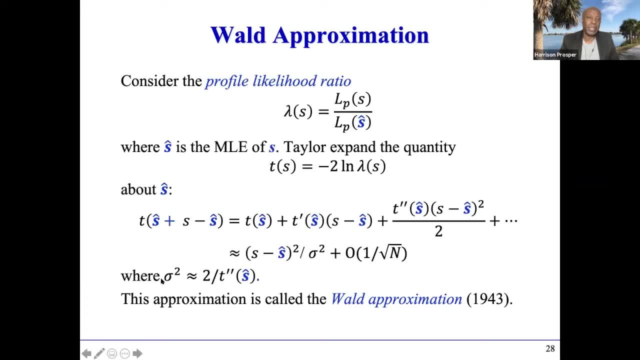 And you can see that, you can convince yourself that this is basically an approximation to the standard deviation of the distribution of this estimate. So, OK, so that's the first thing that's useful is that if you use the probability likelihood and do this, then this quantity here, negative twice log of the likelihood ratio, is approximately equal to this quantity here. 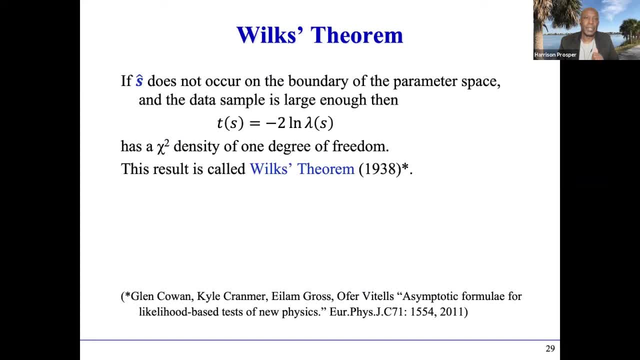 OK, That's one useful thing. The second useful thing is is that so long as your estimate of the signal does not occur on the boundary of the parameter space, so it occurs within the interior of the parameter space, so long as that's true, then there's this amazing theorem by Wilkes 1938, which states that this number here: 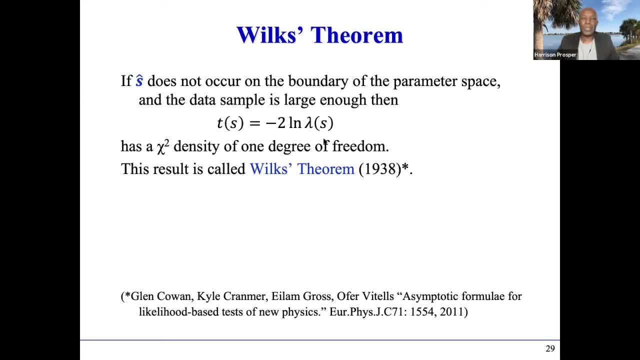 is approximately a chi-squared variate and therefore has a chi-squared density of one degree of freedom. So this is amazing. What it means is that, even though t depends on s, its distribution does not depend on s, And that's fantastic because it means then you know what that distribution is. 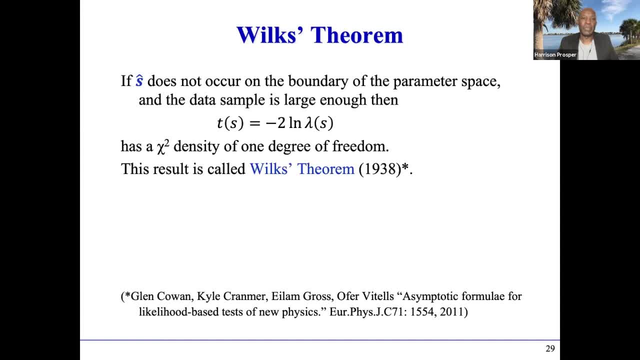 It's actually just a chi-squared density And that is going to be very useful. And actually this- both Wilkes theorem And the Wald approximation- have been beautifully exploited by my colleagues in this paper here you know Glenn Cohen, Kyle Cranmer, Alain Gross and Ofer Vittel. they've written this very nice paper in which they've combined these two theorems to show how one can actually construct a whole variety of ways to test hypotheses, set limits etc. 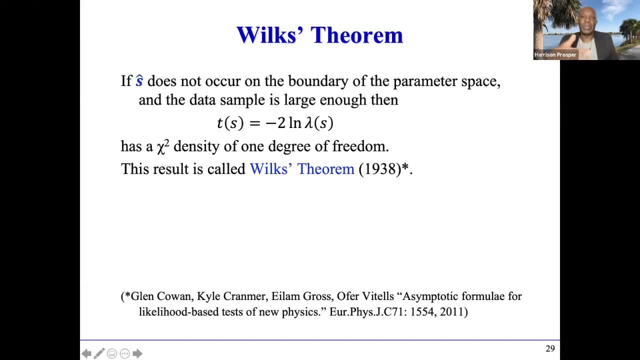 to the degree that one has enough data Such that this is actually true. So I really recommend this paper very, very much. Okay, so the profile likelihood is a good thing to compute, because you can avail yourself of both Wilkes theorem or variations thereof. 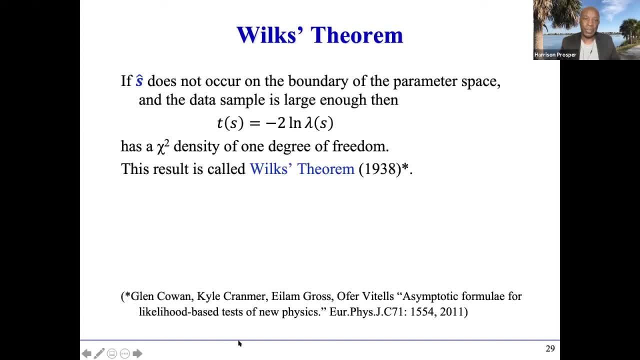 And you can avail yourself of the Wald approximation, which is what they have done in this paper. So that's why the profile likelihood is useful And students should verify this theorem, But what I'm saying is that you can actually use this theorem through simulation. 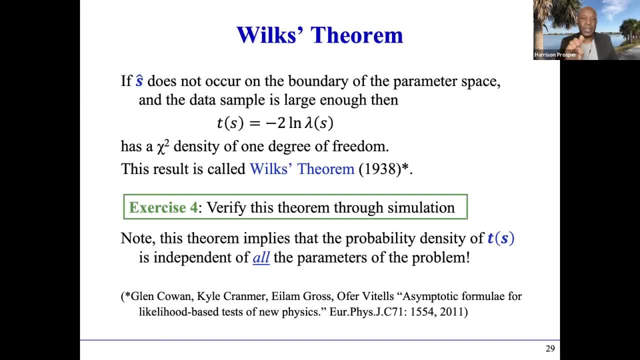 Actually what I might do, since there are these exercises. I may actually put together a Jupyter Notebook with the solution so that people can have a look. So this is really amazing. This theorem implies that even though T depends on S, its distribution is independent of all the parameters of the problem. 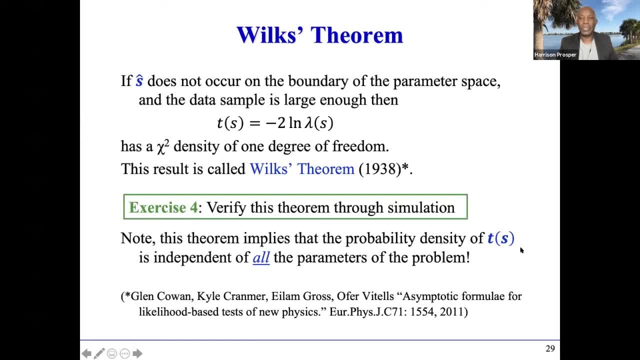 When you have such a quantity- I think it's referred to as a pivotal quantity by statisticians. I think it's referred to as a pivotal quantity by statisticians. So that's actually very good because it means that we know the distribution of T, and that's actually very helpful. 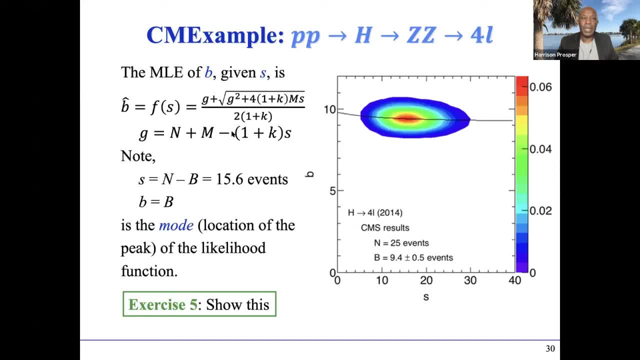 Okay, so let's go for the procedure. Let's apply it to these data. We first of all find the maximum likelihood estimate of the background for a fixed signal, S, And so here's a solution, And we then simply work through this. 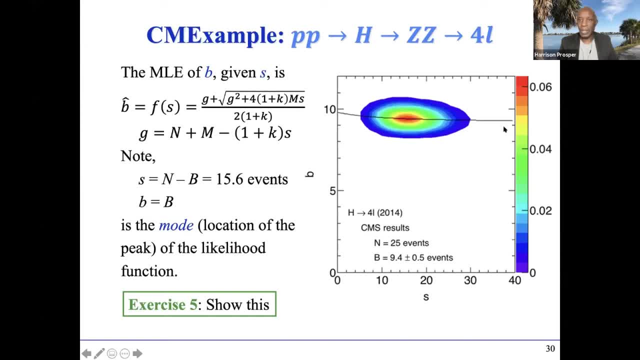 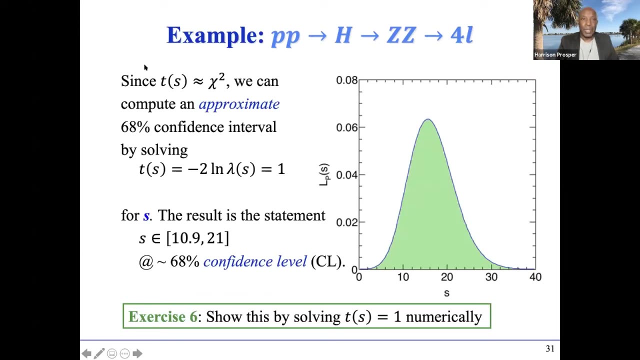 And in fact you see this line here. this line is basically the line that maps out the profile likelihood. So if this was projected downwards, you then would see the profile likelihood as a function of the signal. So, because of Wilt's theorem tells you that this quantity minus twice the logarithm of the likelihood ratio. 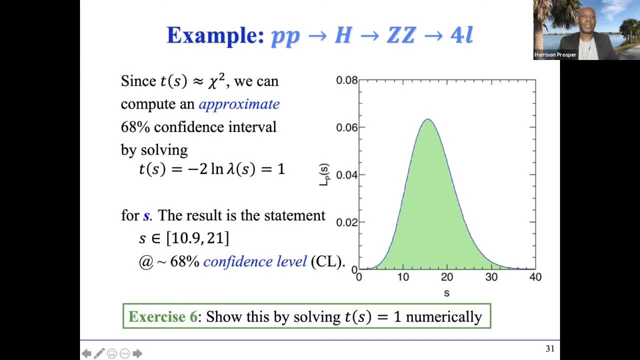 is approximately a chi-squared variate, then that's great because we can- just we can- approximate. we can get an approximate confidence interval by simply solving this equation. We simply set this number equal to one and solve for S, for the lower bound and the upper bound. 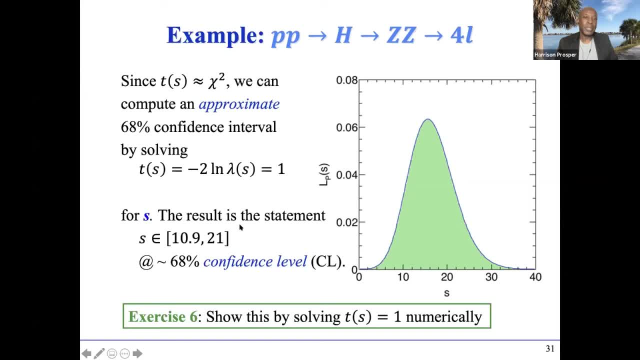 And if you do that, you arrive at this statement. So now we can assert that in this experiment, in this analysis of CMS, where we found 25 events, that the mean number of Higgs boson events in that analysis, in that luminosity, whatever it was, is between 10.9 and 21 events with a confidence level of 68%. 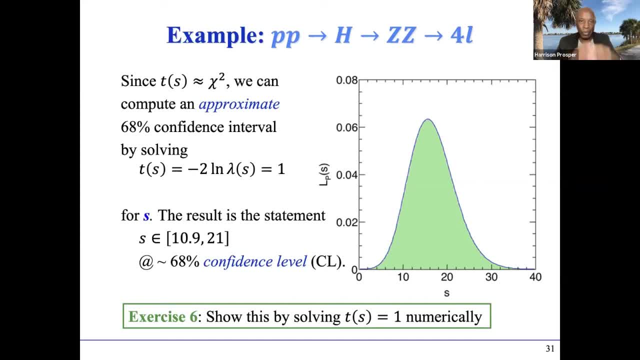 OK, And so this is the procedure, And this is just a simple example of a procedure that's used even for, you know, for all the analyses of which I'm aware at the LAC, including the ones searching for supersymmetry, for example. 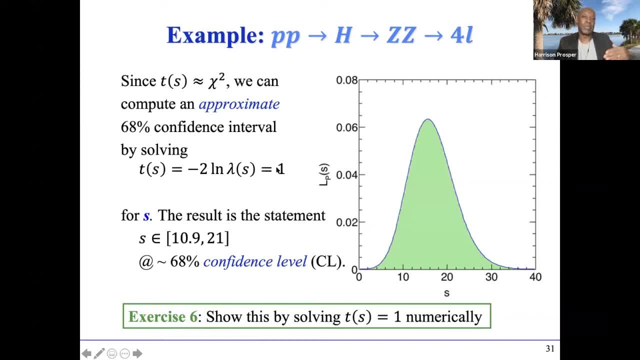 So if this was searching for supersymmetry- you may only be interested in the limit, because you, let's say there's some indication that there's nothing interesting going on- then, rather than setting this equal to one, you may set it equal to- I don't know- 2.7 or something like that. 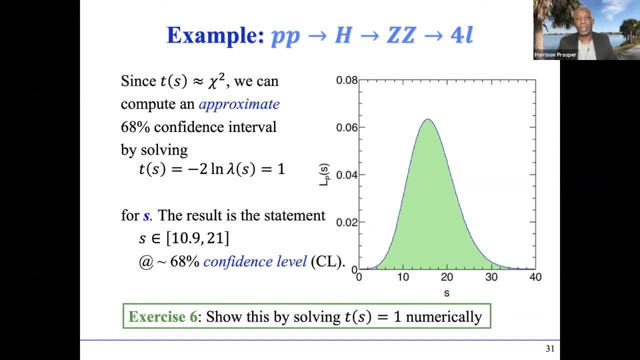 and compute a 95% limit in the one-sided interval, for example on some parameter or say the cross-section. OK, So we have, we have, so we can estimate the. we can basically estimate the signal, We can by maximum likelihood, we can put a bound on it and see what this is doing, this interval. 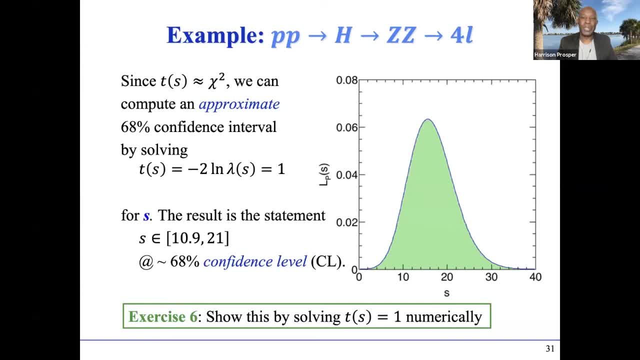 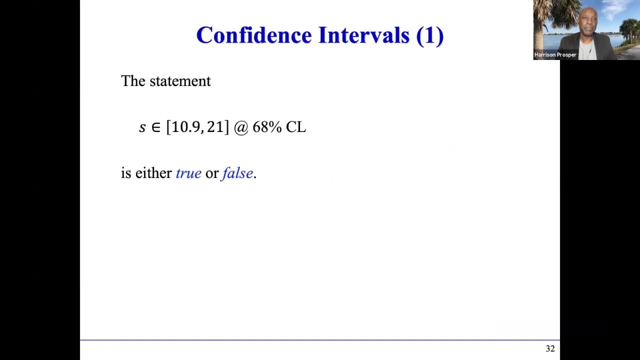 And so now we want to ask a question, which, of course, is obviously answered by just looking at this curve: How significant is the signal? Now notice this: this statement is either true or false. Right, And what we're, what we're arguing, is that if I were to repeat this many, many times, 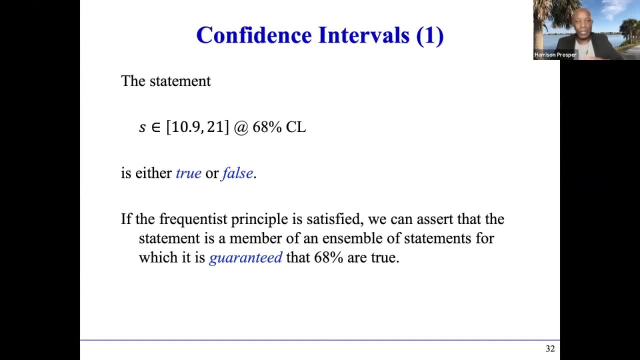 different experiments. there'd be true statements, there'd be false statements, but the fraction of true statements would be at least 68%. right, That's the idea, But, but remember, the frequency principle is not likely to be satisfied, exactly because we've made an approximation. 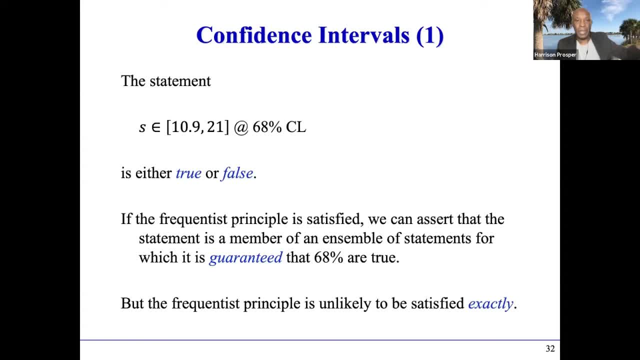 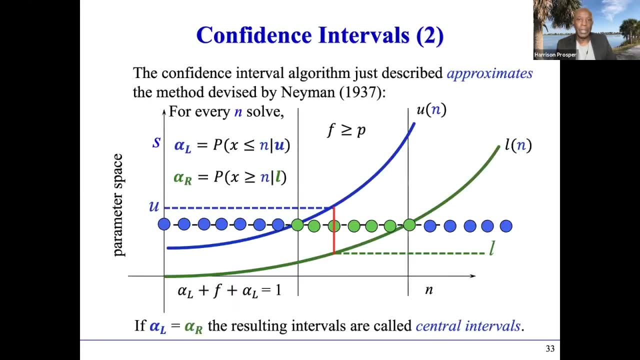 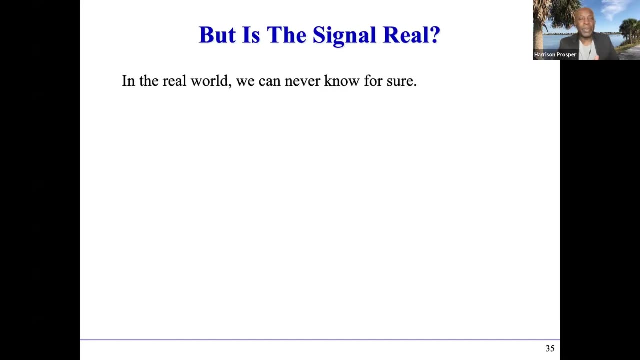 We replace all the things which are unknown by estimates thereof, And so that may lead to some so-called under-coverage. Let me just skip this. And so we're coming to the end of the first half, And so the question of course now is- and this will be- this, of course, would be an exciting thing. 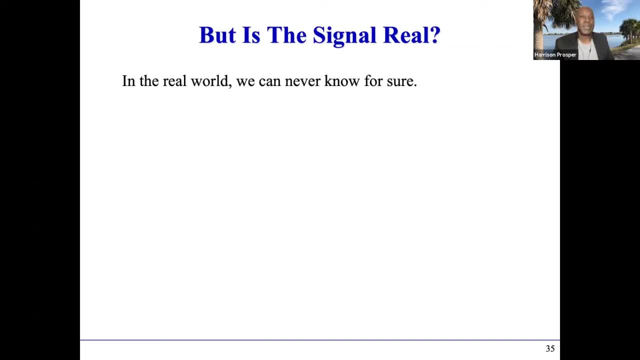 Let's say, 10 years from now. we are, we are getting a hint of something new, something really exciting. Then of course, we would like to know: is is? is this signal a real thing? Obviously, we could never know. 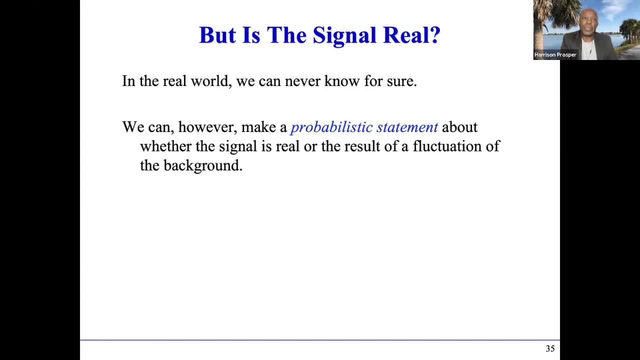 We never know for sure. right, We never know for sure. So what we have to do is make a probabilistic statement about whether the signal is real or whether what we're seeing is a fluctuation of the background. And this is as you know. we particle physicists are really, really careful about making bold statements such as: there's a Higgs boson that exists, right? 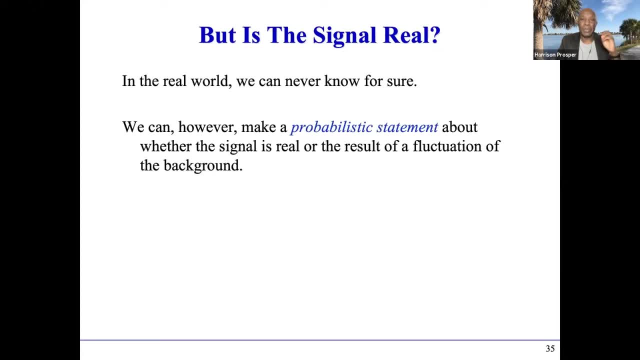 We have very strict criteria for arriving at this, Arriving at such a conclusion, But they're still probabilistic, right? There's still a chance that our bold statement is actually wrong, And of course, we all know our field has had this history of bold statements that proved to be wrong. 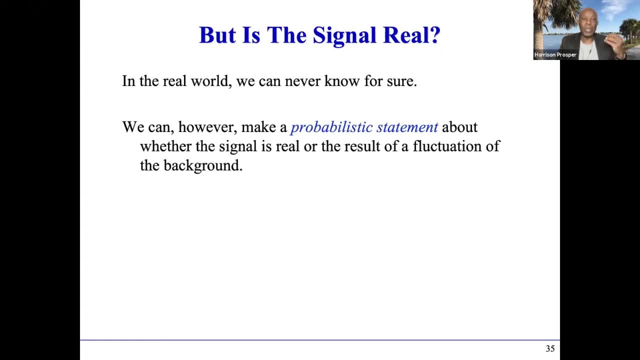 That's fine, That happens. You know, science is a thing made by human beings And we can sometimes be wrong, And so, in order to decide whether or not a signal, you know something. you may have evidence that there's a signal. 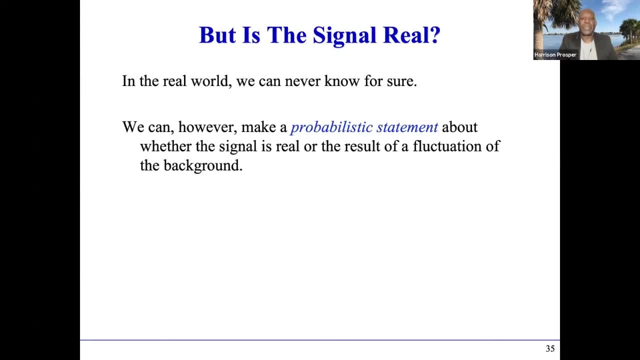 You know something, you may have evidence that there's a signal, But in order to really say whether this is real in a probabilistic sense, of course, we usually consider the background-only hypothesis right. If that hypothesis is extremely unlikely, how do we argue? 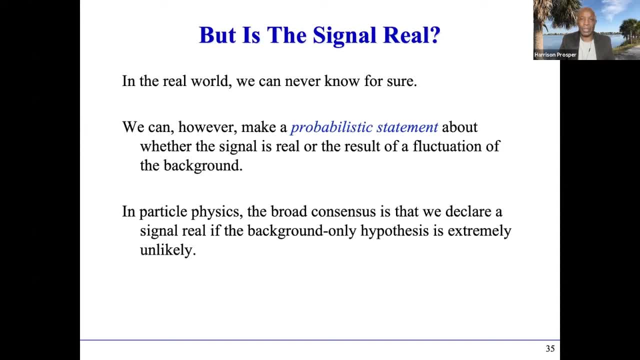 We argue: let's suppose that the background-only hypothesis is correct, right? For example, in the case of the Higgs boson discovery, we said: okay, let's suppose that the standard model is real. The standard model without the Higgs boson is the true hypothesis, which, of course, is a model that is completely unsound. 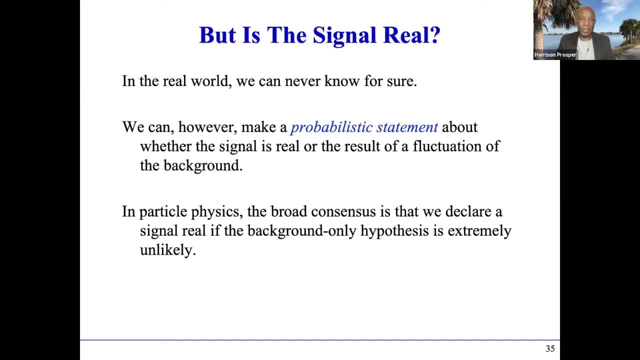 But that's essentially what we did, right? We said: here's this model. We're going to assume that the Higgs boson does not exist, And then we do the experiment, And then we construct some measure, And if that measure indicates that that hypothesis is extremely unlikely, 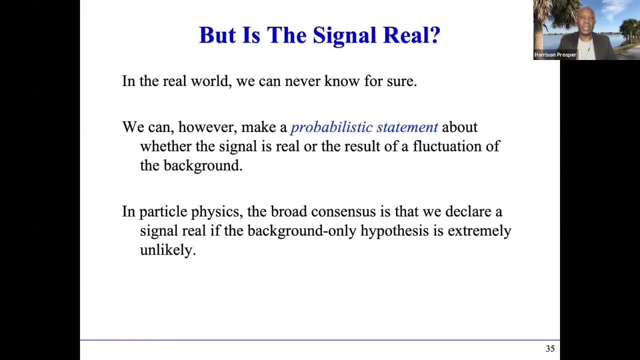 then we conclude that the Higgs boson does not exist And then we conclude- as we did in 2012,- that the no-Higgs hypothesis is false, And that's kind of the reasoning. But I want to make that a bit more precise in the next half when we talk about hypothesis testing. 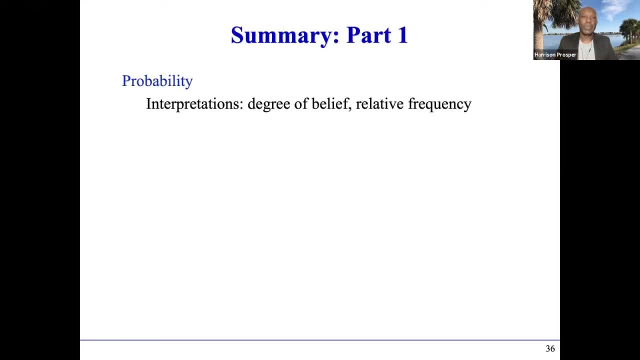 So let me just summarize this part, Then we'll take a break And then we shall continue with that. So probability: Everyone agrees that If we wanted to make inferences about models or whatever they might be, probability is the underlying thing everyone agrees upon. 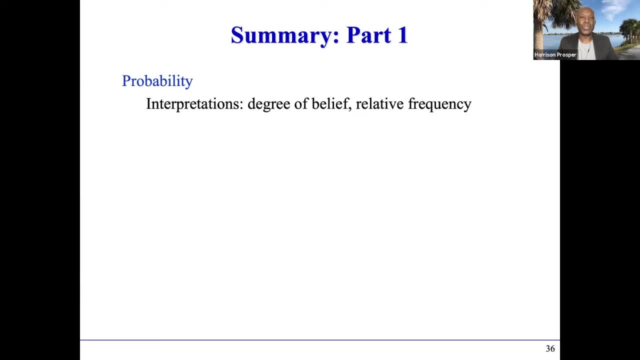 However, people disagree about which of these two interpretations is preferred. In my view, both of them are useful and both of them should be used. Degree of belief which does not depend on an ensemble right. It's a statement about a particular singular statement. 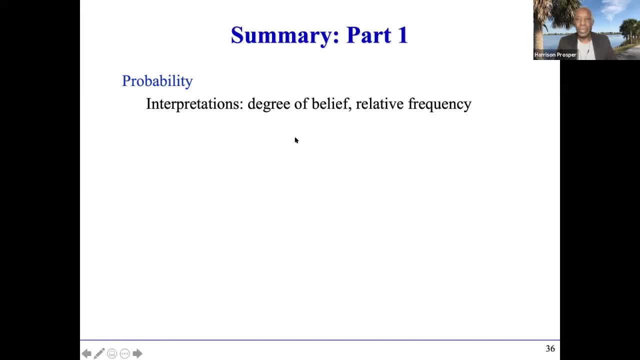 And that's it, Nothing more. Or relative frequency, which relies upon the idea that there are repetitions of things, And when you repeat these things and you count how often a particular outcome is realized, then you can compute the relative frequency of those outcomes. 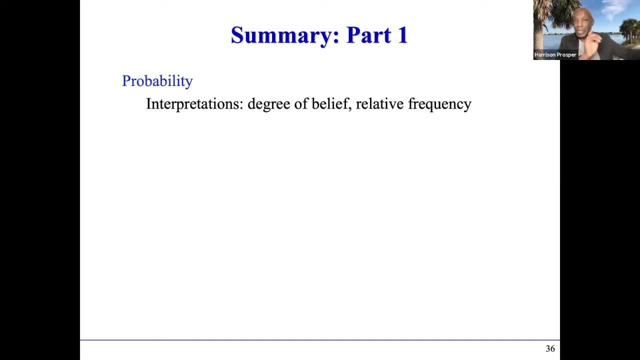 And one presumes that, as you repeat this to the degree that your repetitions are in fact constant in some sense, that this relative frequency will settle down to some number called the probability. So both of these interpretations are important and ones that are used. Then you build a model of the mechanism that generates the data. 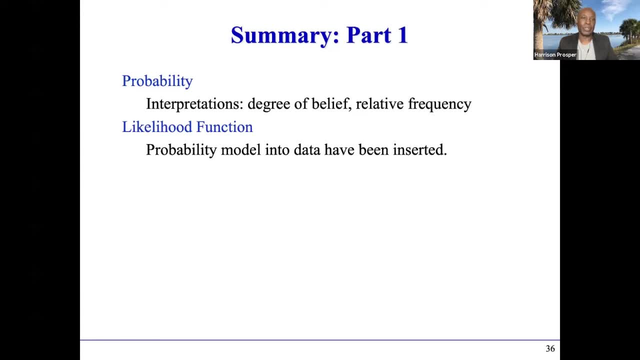 And invariably, if we're doing a counting experiment, we basically use a Poisson distribution And I give sort of an argument as to why that is reasonable And then you plug it in, And then you plug into your model the data that you've observed. right? 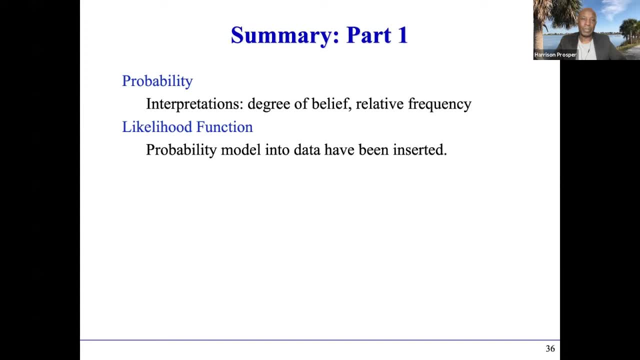 And once you've done that, the data, of course, are just constants. The model now becomes just a function of the parameters, Let's say the signal strength of the Higgs or the cross-section, things like that. And once you have that likelihood function, you can then continue to do inferences. 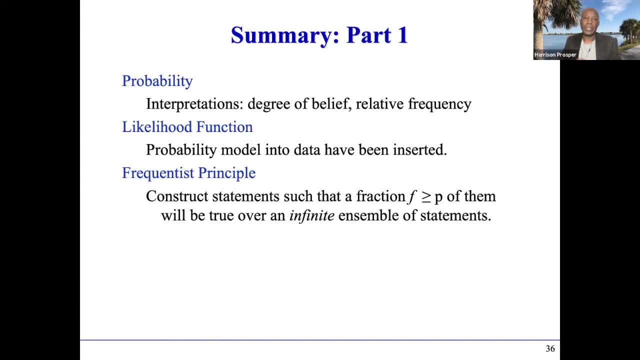 And the basic idea is that you want to. you want to construct a statement. For example, the signal strength lies within some bound. That statement is either true or false. We never know whether it's true or false, But you construct those statements in such a way that if over a huge ensemble of such statements that have been made, 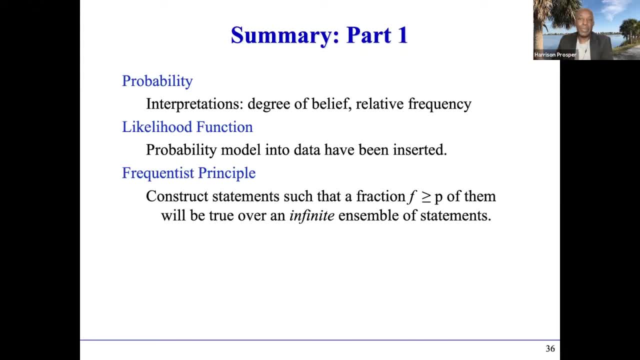 none of the statements you know are true or false. You can never determine whether a statement is true or false, But because of the manner in which those statements have been constructed, you can then guarantee that a fraction f of them are going to be true. 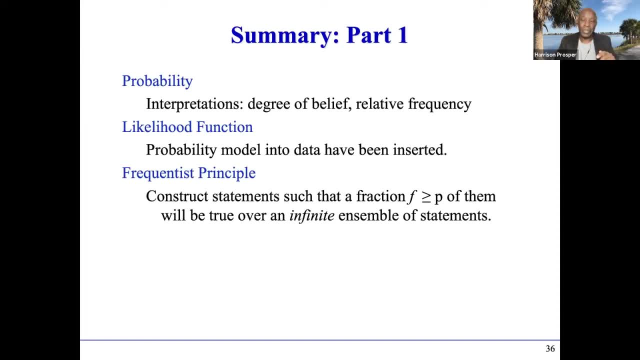 That's sort of the idea Now, of course in principle. that's in principle, But of course in practice, because we have to get rid of nuisance parameters and we replace them by their estimates, then it's not completely clear that this is going to be true. 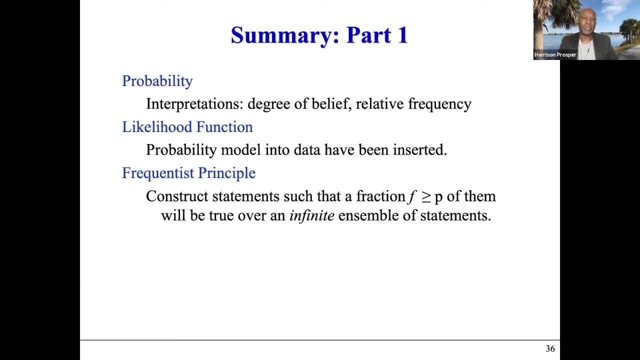 But in fact, it turns out that, in practice, we do a very reasonable job, And this is what this is saying, is that we have to get rid of these nuisance parameters one way or another, And the technique for doing so is to profile the likelihood. 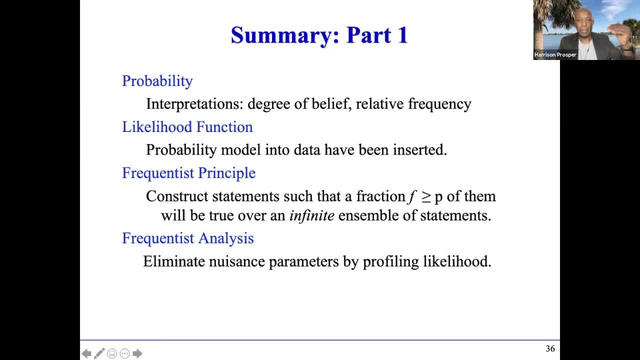 basically to replace all the nuisance parameters by their maximum likelihood estimates for given choices of the parameter of interest. That's sort of the basic idea And even though I've gone over a very simple example which we're going to continue in part two. 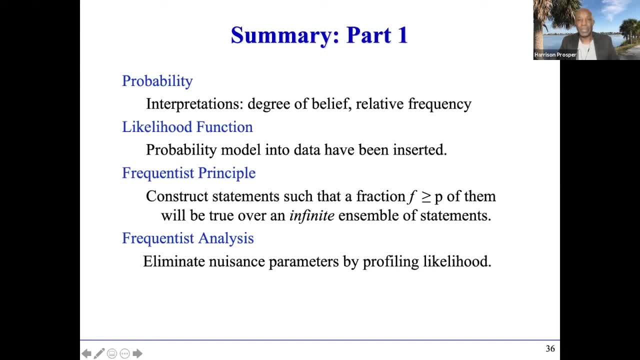 it's really the prototype of of all the analyses at the LHC, which, of course, can become extremely complicated because of all the details that one takes into consideration. OK, so let's stop at this point And maybe we can take a few questions now, or take a break, as you wish. 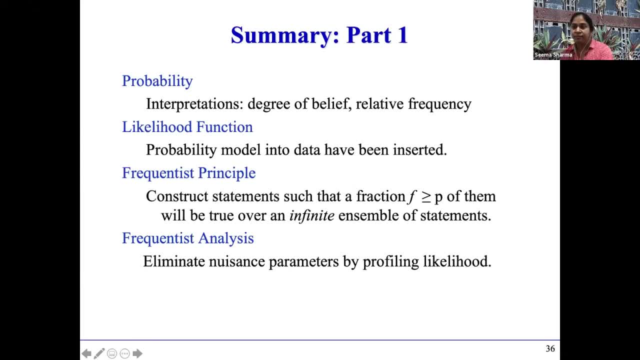 We have some questions. OK, fantastic, Please go ahead. Camelia, do you want to go first? Yeah, Hi, Could you please repeat that? why did we need to compute the Poisson? I mean the Poisson probability for m. 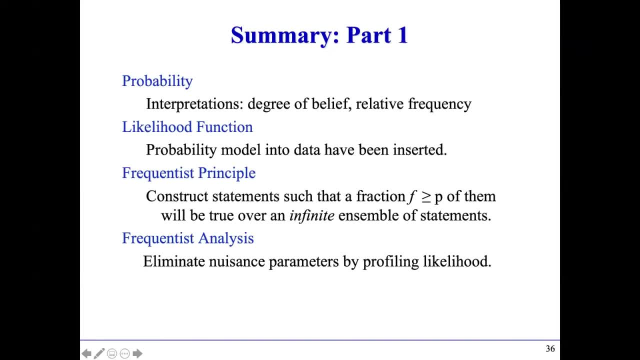 I mean the count m, the likelihood for the count m. Yes, OK, thank you. Thank you for the question. So the one of the goals in building these, these model, is to try to be as precise as you can. 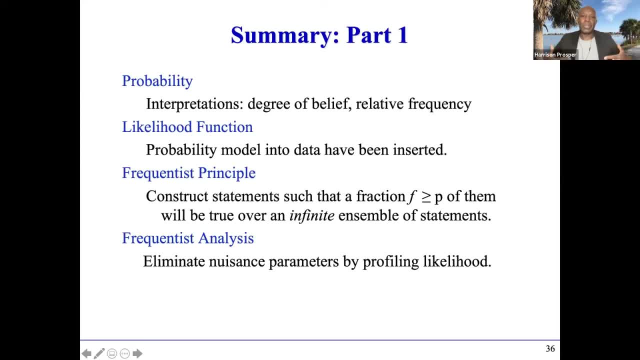 as get as close as you can to to the manner in which the data have been manipulated. Right, So I? I could have. I could have said: you know why not, Since we have a background estimate. background is: what was it? 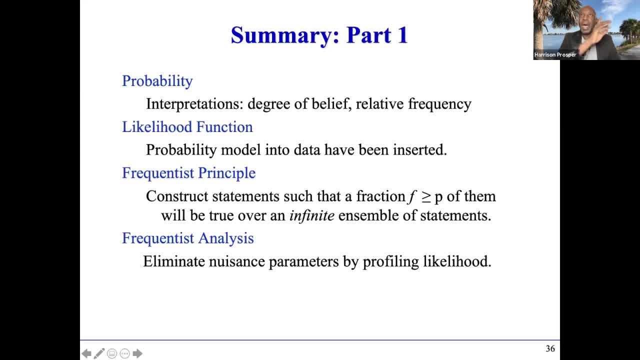 Nine plus minus 0.5 events. I could have chosen to say: let me assume that this is a Gaussian. Let me assume that that I can represent this particular result as a Gaussian, where 9.9 would be sort of the. 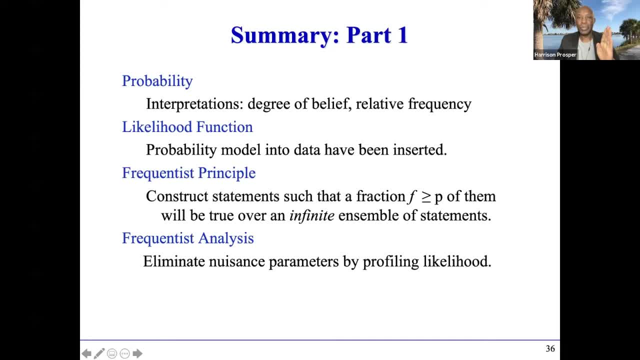 you know would be the measured and 0.5 would be the standard deviation. And I could have used a Gaussian instead. I could have had a Poisson right: Probability of getting n equals 25, given s plus b times a Gaussian. 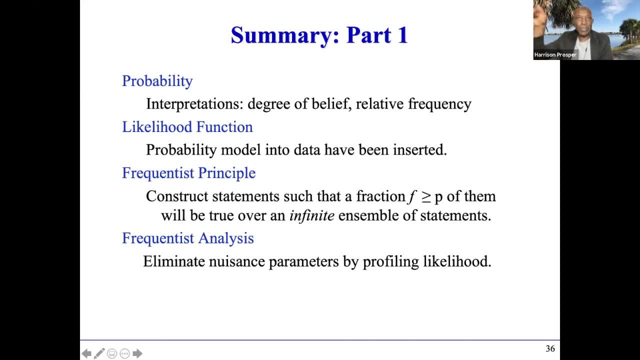 where I plug in nine events minus b, divided by 0.5 for the standard deviations, all squared Right. I could have used, I could have used a Gaussian. Now it turns out that for this particular set of results, because there is a, 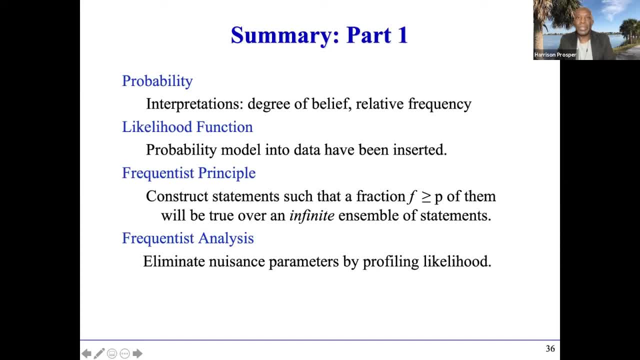 there is a substantial signal, as we shall see in the second half. the Gaussian would have been reasonable Why? Because the uncertainty is 0.5 compared with nine, nine events. But the reason I went through this little exercise was to show what you could do if you were not in this happy situation. 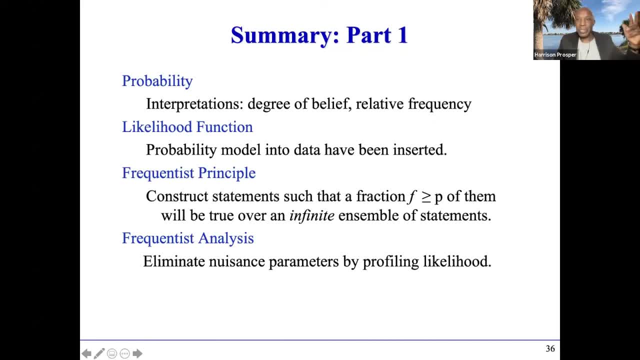 Suppose you had nine plus or minus, I don't know, three events or a larger uncertainty where there's a possibility that the Gaussian could have a long tail towards negative, towards negative values for the background, Then what people used to do at the Tevatron. 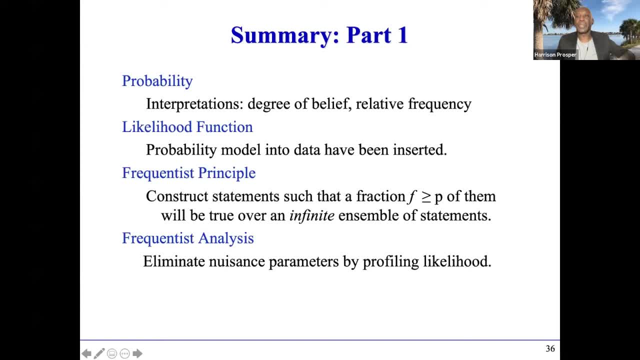 for example, is that they used to truncate, truncate the Gaussian at zero. Well, that's not a very good thing to do. You would like to have a function that goes to zero at zero, And so, by going through this exercise, you arrive at a function that looks very 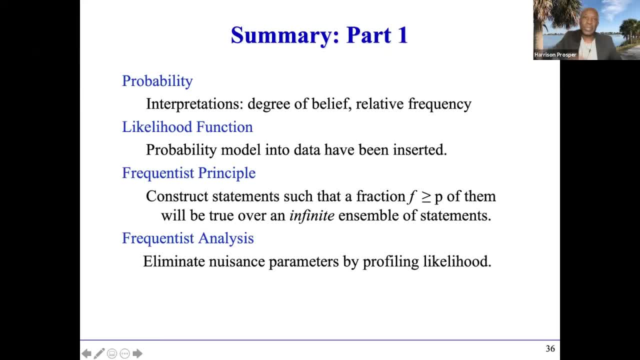 very Gaussian around where the background is, but actually goes to zero at zero, which is a much more sensible behavior. So that's why I did I did this. Okay, Thank you. So I'm sorry I missed that, But I did not understand how come the maximum likelihood estimate of a 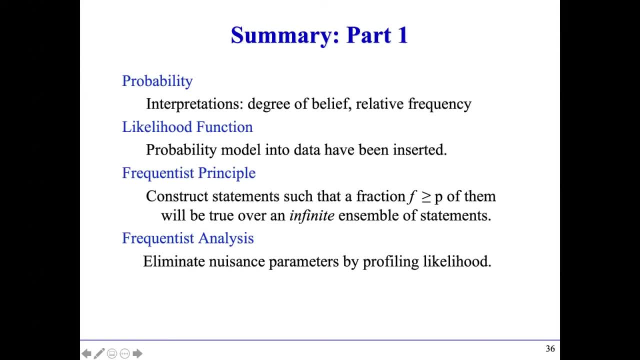 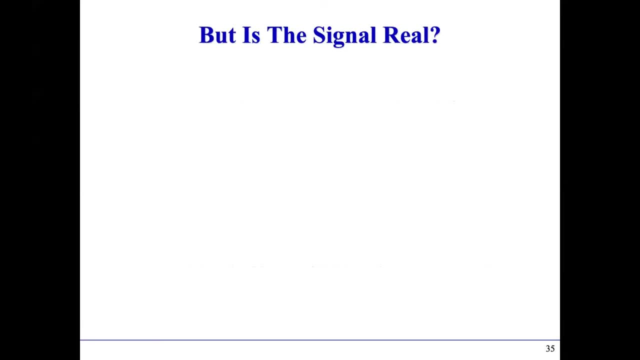 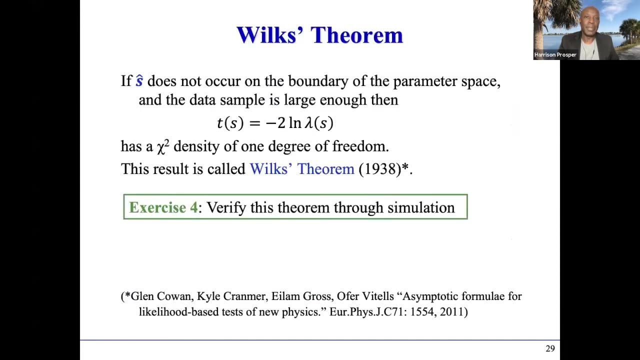 nuisance parameter is a function of signal, because you've not looked at data at that point, right, Okay, So so, let me, okay. Thank you for the questions. Let me go back to. yeah, let me go back to. 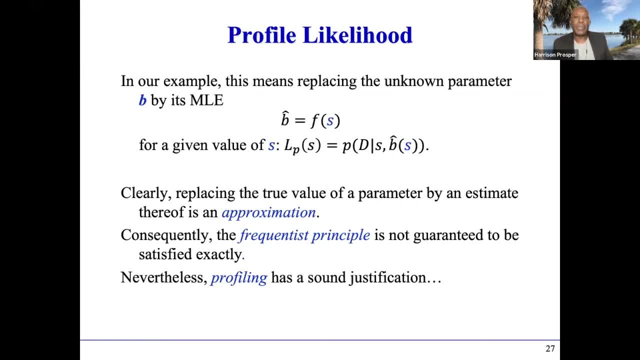 to here. Okay, So What I mean by this is this: So this is a function of two parameters: the signal s and the background b. Okay, There's two parameters. So what I'm saying here is this is that I fix s. I said s equal to 0.5 event. 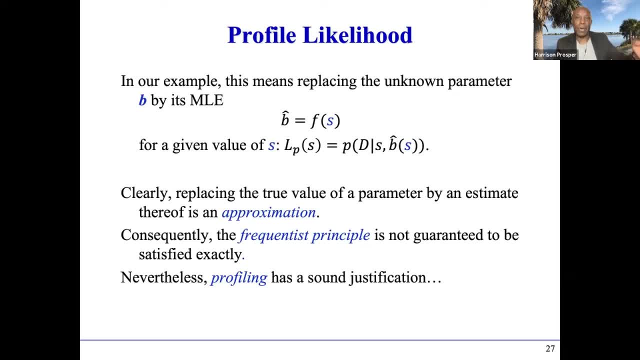 And then I run my favorite maximizer, minui, to find the best estimate, maximum, the best estimate of the background, for s equal to 0.5. So I get some. I get a value b hat at s equal to 0.5. Then I go to s equal to 1.. And I repeat this: 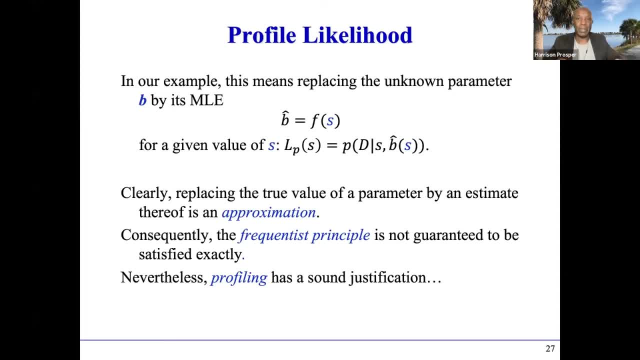 I find the best estimate of the background, assuming S is equal to 1.. I then go to s equal to 1.5. And I repeat this, And as I do so, I will map out a function of s only. 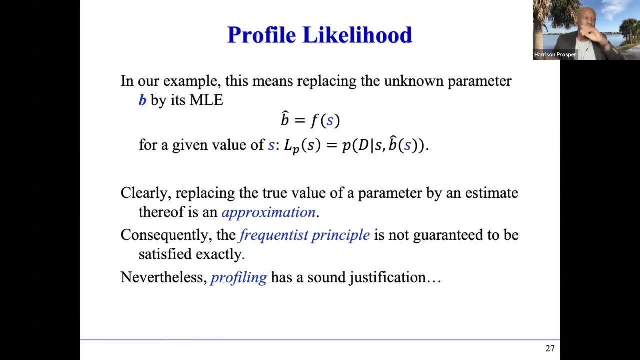 And that is literally what is done. What is literally done? for example, I'll give you a more realistic example. In the Higgs discovery work there were two quantities that were of interest to us. right, There was the signal strength of the Higgs signal. 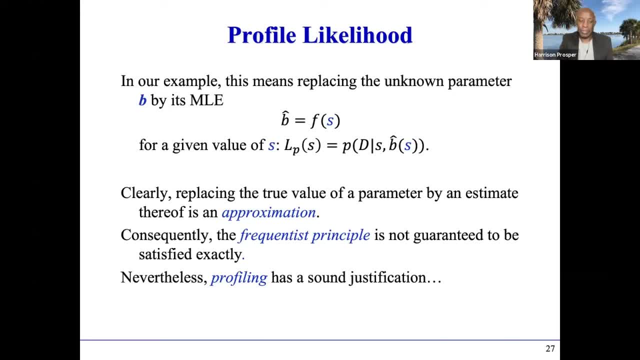 And there was the signal strength of the Higgs signal, And there was the signal strength of the Higgs signal, And then the Higgs boson, or this resonance mass, And what was literally done was for every point in that parameter space for a given Higgs boson mass. 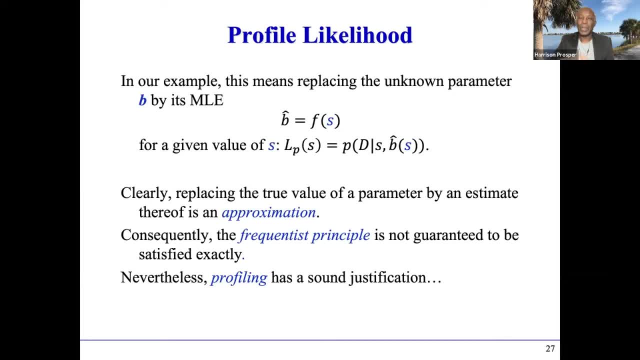 and a given signal strength, all the nuisance parameters in the problem were maximized for that particular point, And this was done for every single point in that parameter space until we actually mapped out a function that depends only on the signal strength and the Higgs mass. 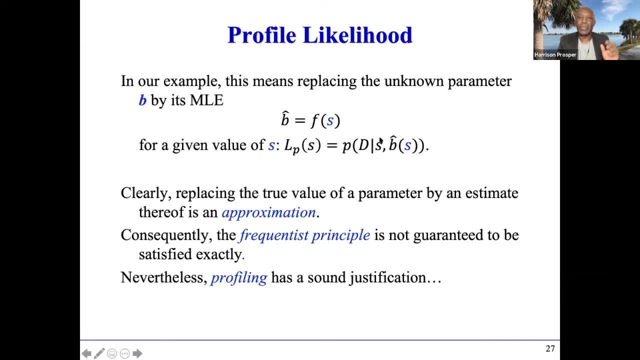 And so here we're just doing a simple example of that, where instead we have only a single parameter s, And you're quite right, We don't know what it is, We have no idea, We'll never know. But what we do is that we say let's just have different hypotheses for the signal, starting from zero up to a very large value. 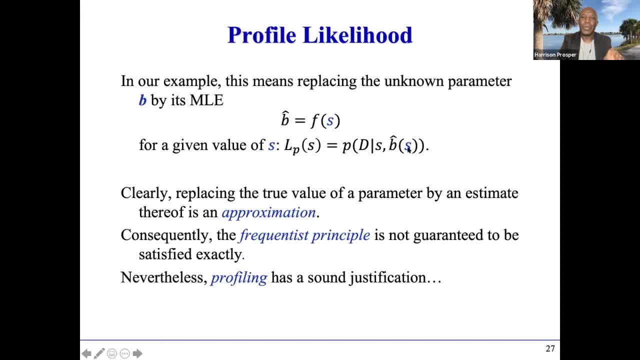 And for every particular value of the signal, we find the best value of the background. And then, having found the best value of the background, we find the best value of the signal. And then, having found the best value of the signal, we find the best value of the background. 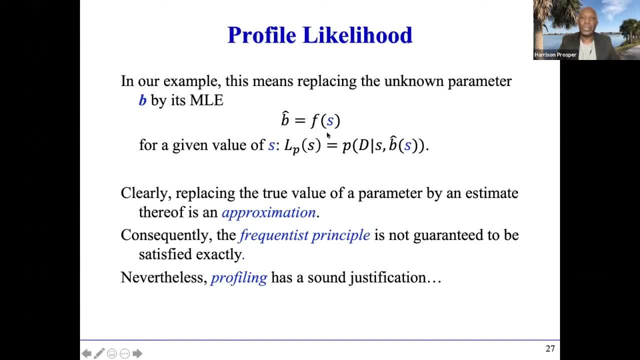 We plug it back into this function And, as a consequence, this function just maps out a curve that looks like a function only of the signal. Okay, So when we are finding this best fit value of B hat, then we are also simultaneously looking at data. 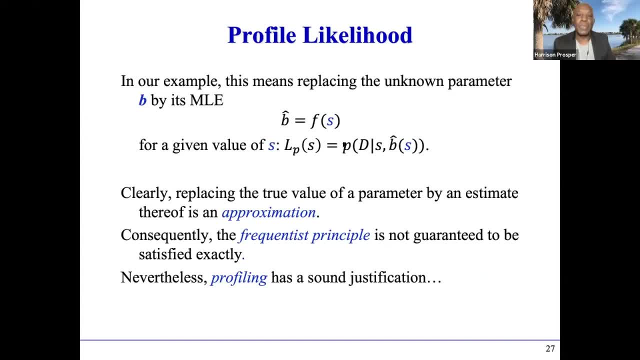 Like that's how we are deciding: Yes, yes, yes, yes, That's right, Because, see, this is the point We have now plugged in. So there are two steps. The first step is building your probability model. right, 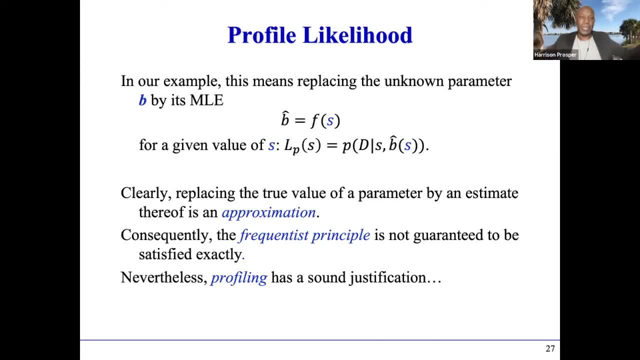 Right, And then you say, okay, I do the experiment, I plug into my probability model the data. In this case I have 25 events that were found And I have, you know, I have information about the background. So now, because the data are constants, this function necessarily is now a function only of the parameter. 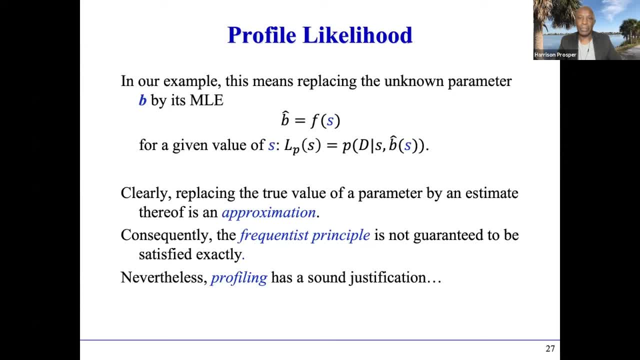 In this case, the signal mean and the background mean, And so, but I want to get rid of the background somehow and that's the technique that is used. Right, Okay, Okay, thank you. Thank you for the question. Thank you, Angira. 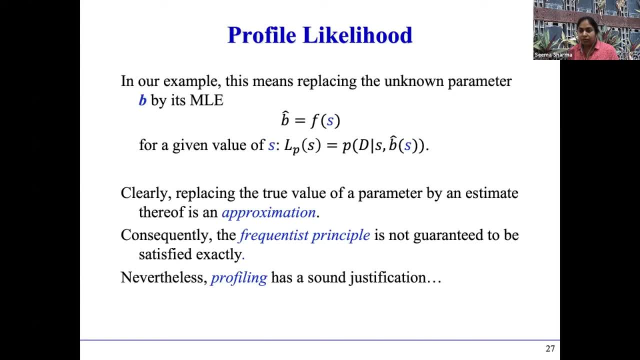 You can lower down your hand, please. Any other question? I think, Sanjay, you changed your mind. I'm just trying to send it to a pen. I'm just asking for a second. Okay, Harrison, so do you want to take a break now for 10 minutes? five minutes. 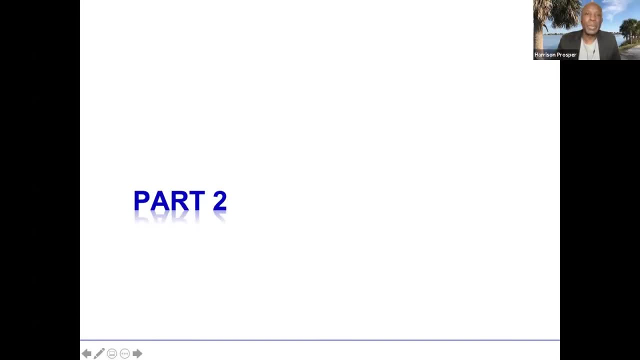 Yeah, just take five minutes. Yeah, Okay, So let's. so now we're going to part two. So so we we've, you know, found the estimate of the signal. We've, we've put a bound on the signal that quantifies its accuracy, right? 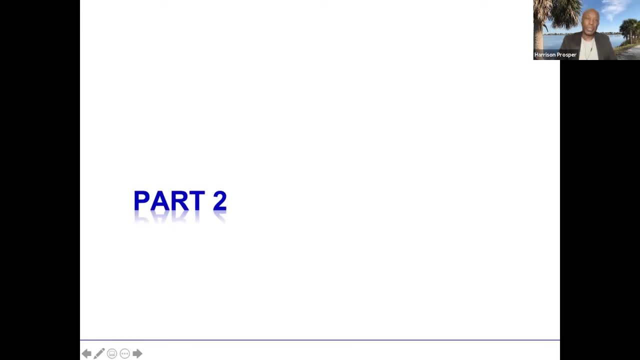 This confidence interval, And now what we want to do is to assess the degree to which the signal really is real. We want to do a hypothesis test, and that's what we're going to talk about now, and then we'll talk briefly about Bayesian methods, if we have time. 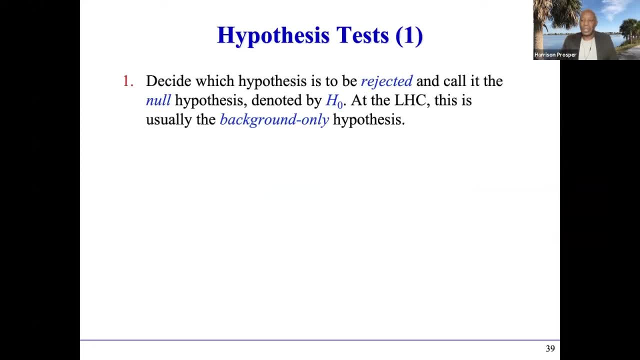 So how does one test an hypothesis in this approach? Well, the first thing we want to do is decide which hypothesis we wish to reject. So we require some data and and the idea. the goal is to reject this hypothesis. The one to be rejected is called the null hypothesis. 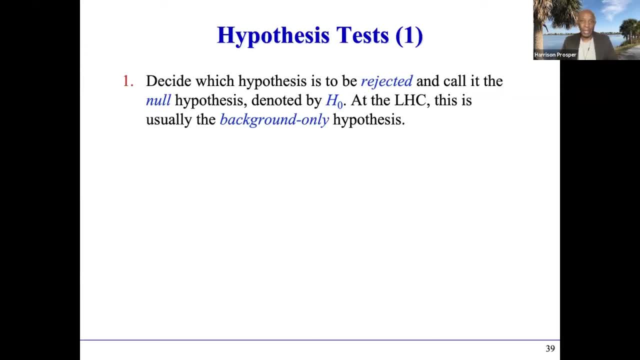 And again going back to the discovery of the resonance in 2012.. That we now believe is the Higgs boson. The idea there was that we wanted to be able to reject the hypothesis that the Tang model is a theory without the Higgs boson right. 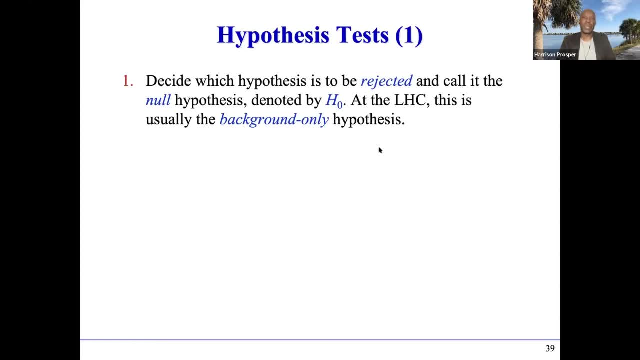 That was the model we wanted to reject. That's the null hypothesis. We'll call that H sub nought In background only is the typical hypothesis. Okay, So we've figured out what we want to get rid of, And then we construct a function. 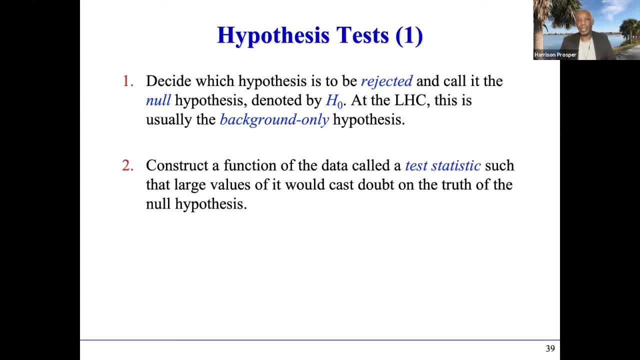 Okay, Of the data, maybe plus some other things. that's called a test statistic, And usually it's not always, but usually we- we construct it so that large values, and ever larger values, cast ever more doubt on the truth of the null hypothesis. 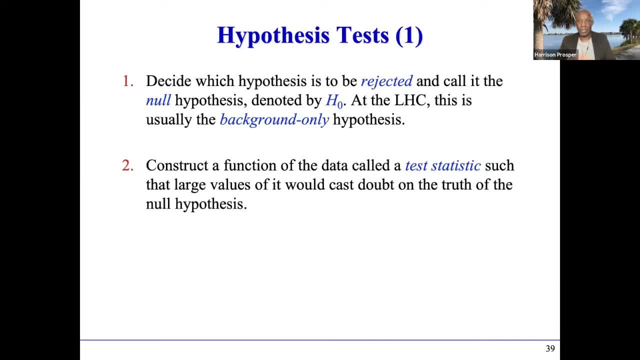 Okay, So you construct a statistic, and if this, this quantity, is very big, we will say, well, maybe our null hypothesis Isn't true after all and therefore can be rejected. And then, having built this test statistic, you choose a threshold above which you are. 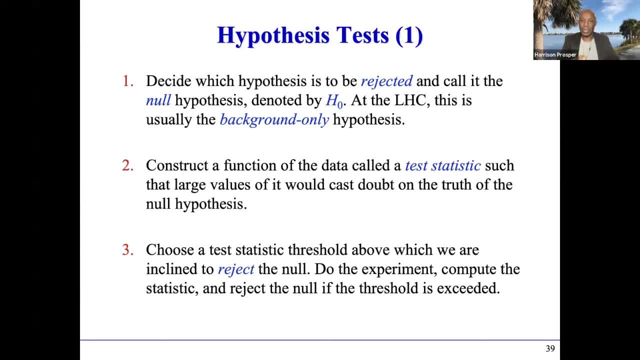 prepared to reject the null hypothesis. So you say, okay, let's choose this threshold, And if we get result that's above this threshold, then we shall declare that the null hypothesis- I this case, a background only or the model- without a null hypothesis. 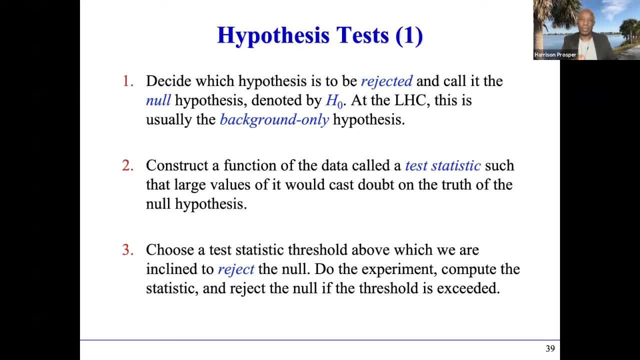 The Higgs boson should be thrown away. It should be discarded. So so those are the steps. you decide which hypothesis you are planning to reject. You construct a test statistic in such a way that big values and bigger values indicate ever more doubt on the truth of the null hypothesis. 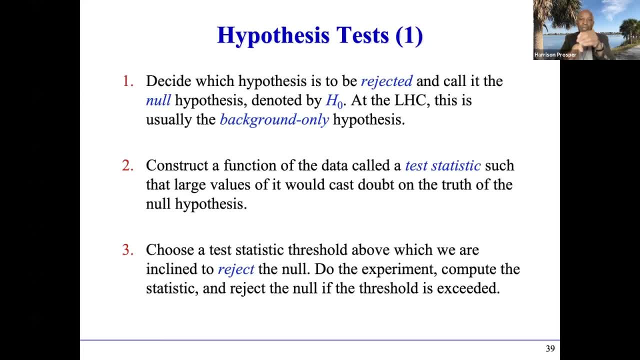 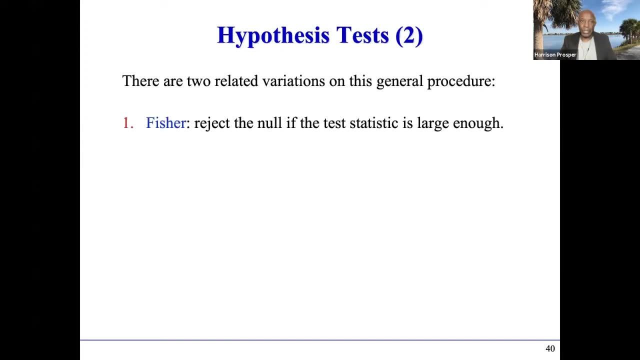 You choose a threshold, you do the experiment, and if you should get a result that exceeds that threshold, then You agree to reject the null hypothesis. That's the idea Now. so this is the general procedure, but there's there are at least two variations of that. 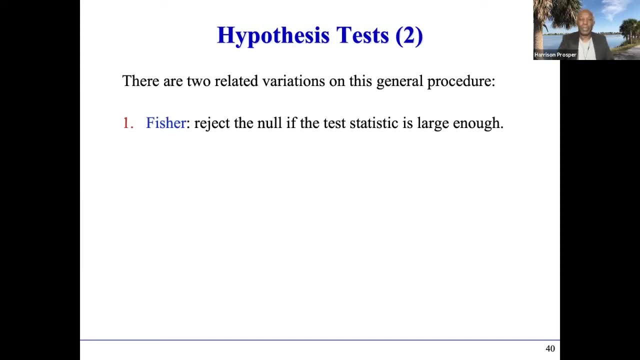 general procedure which are used in particle physics. The one of them is due to Ronald Fisher who, in the 1930s was did a lot of work in this area, and his idea was relatively simple. He says: look, if my test statistic is big enough, I should reject the null. end of story. 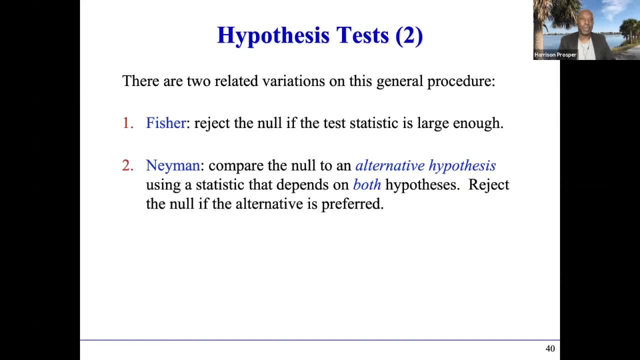 Yashick Naiman. we've met earlier with a frequentist principle. He disagreed with Fisher and he said: no, no, no, no. this doesn't make any sense. You've got to compare two hypotheses: The null hypothesis. 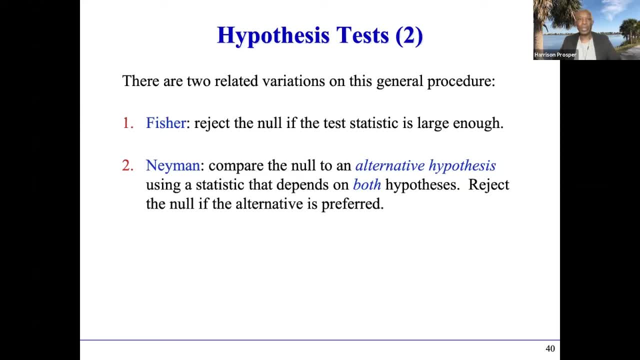 And you have to compare with an alternative hypothesis, and only a comparison of hypotheses makes any sense, and so he built a theory that required the comparison between two hypotheses. Fischer, of course, thought it was not sensible, because he said: well, you may not have an alternative hypothesis. 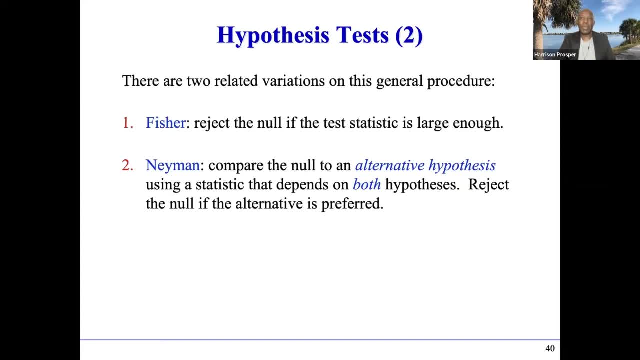 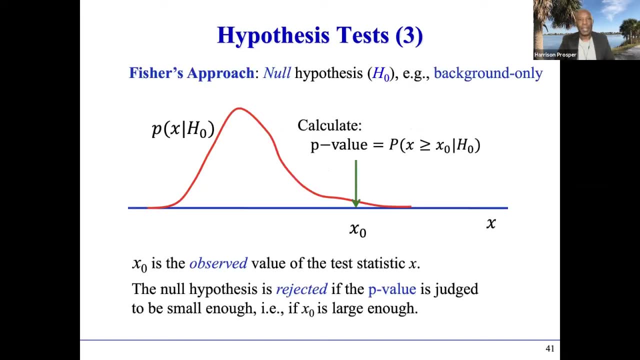 but in fact we physicists being pragmatic persons, we use both approaches, which I think is sensible. So let's start off with the Fischer approach. So here is a the probability, you know, model for the non-hypothesis. So we assume that the non-hypothesis is true. background only: 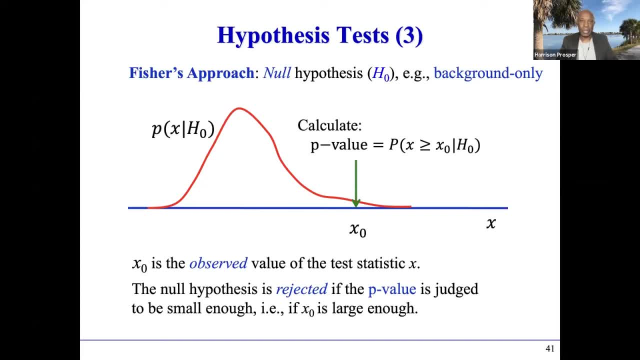 nothing interesting happening. sadly there's no Susie, it's just some model, nothing more than that. and this curve is the probability of getting some quantity x if the background only hypothesis is true. So we assume that the non-hypothesis is true. background only: nothing interesting happening. 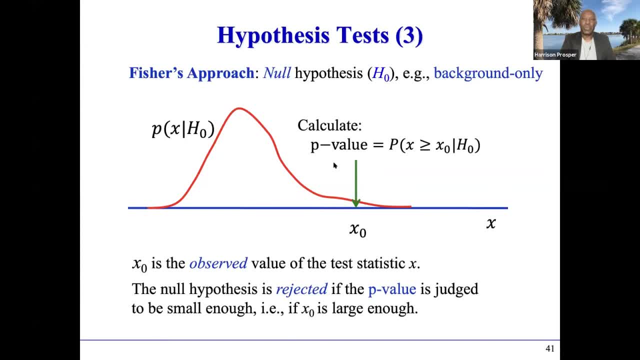 is true. So now we get a measurement that is x sub naught, and we compute the tail probability that is from here off to infinity, or the upper bound. That tail probability is called a p-value right, And so the idea is this: is that if the null hypothesis is true, 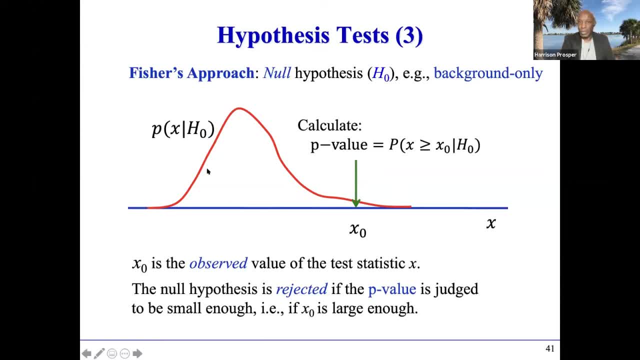 then of course you know, then of course you can map out this entire curve and you can compute these numbers. But if this number, if this probability is really really small, then you might begin to question whether the null hypothesis is true. right, Because if this p-value is very 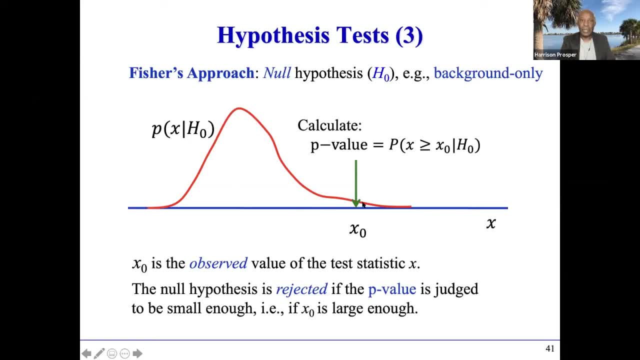 small, then there are two possibilities: Either the back-end only hypothesis is true and we just have there's just a big fluctuation that has occurred, Or the null hypothesis is false and something interesting is happening and we should therefore reject the null. And it's up to us right, There's no. 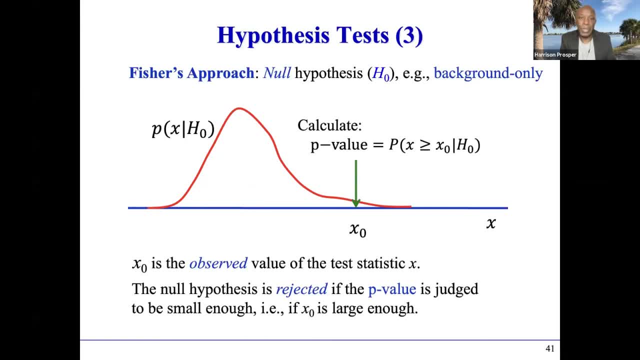 I mean, there's no law that tells you what you should do. Now, in particle physics we are very strict, And what we typically do is that we say: look, we want this number p to be 2.7 times 10. 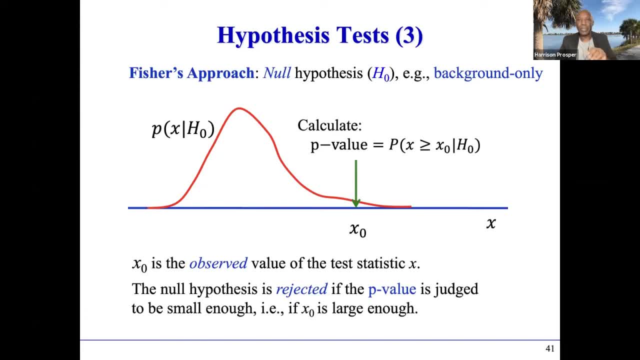 or smaller, And and if we find a p-value that's smaller than that number, which corresponds to five standard deviations in another measure, then we are prepared to declare that null hypothesis, ie back-end only or standard model only hypothesis, should be rejected and declare. 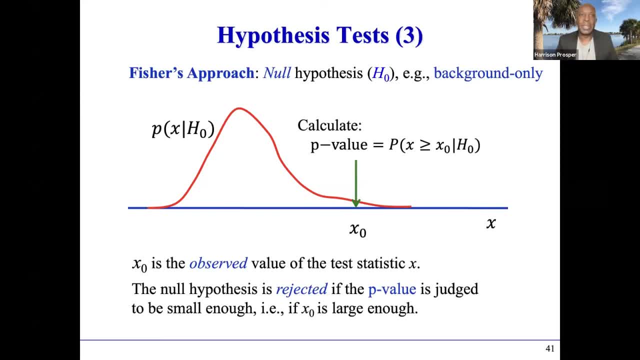 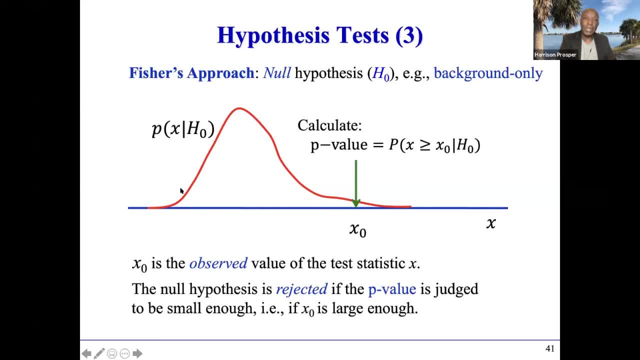 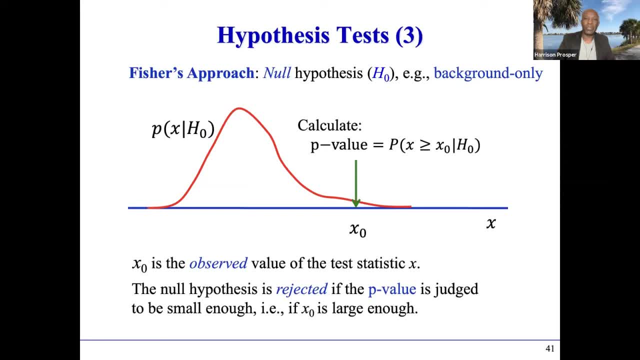 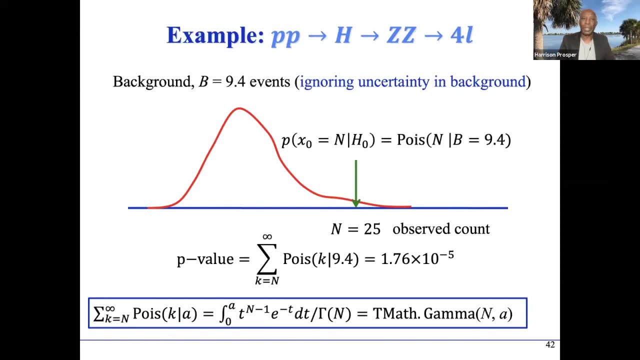 you reject the null And we, as I say, have a very strict criterion for doing so. So let's, let's apply that to the our example, for, So recall, the background count was 9.4.. For now, let's ignore the uncertainty, right, Remember. 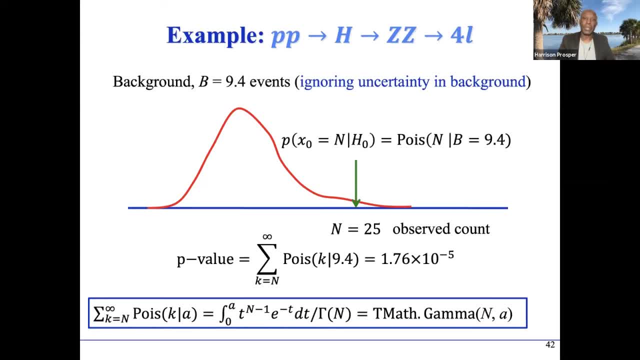 the certainty was 0.5 events. Let's ignore that for now, So let's just compute it. Well, to compute it, we simply have to integrate or, in this case, count from the observed count. in our case, n equals 25 event off to infinity. We simply compute this and what we find is that this: 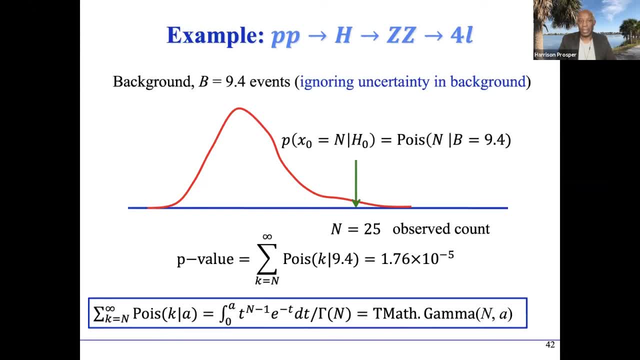 p-value is 10 to minus 5,. okay, And, by the way, you can compute this quite easily by using this thing from root. Okay, so 10 minus 5, so that tells you that it's not quite big enough. 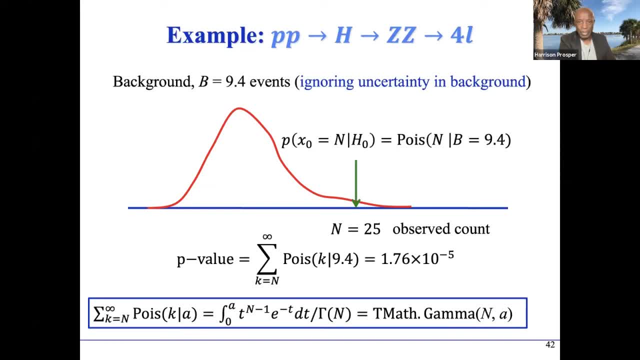 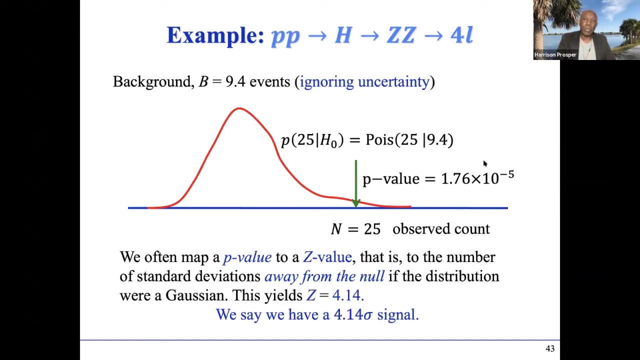 small enough, rather on its own, to declare victory and say we've made a discovery. but it's sort of you know it's getting there right. So this is the p-value, Very simple idea. Now we have a very poor intuition for these kind of small numbers, and so usually what we do, 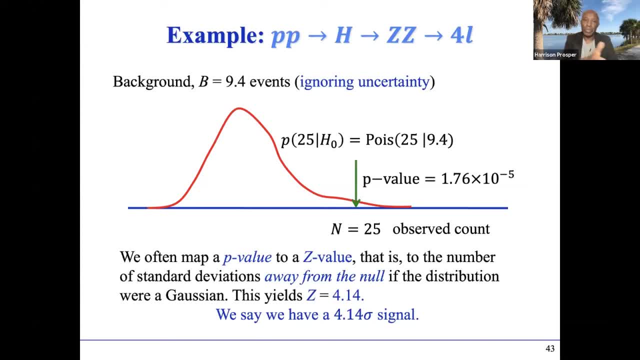 is that we convert these numbers, p-values, into some other. another measure, which is, which is to assume that we say: well, let's suppose this were a Gaussian. Let's say, if this were a Gaussian, then this point here where the green arrow lies, would correspond to some number of ton deviations. 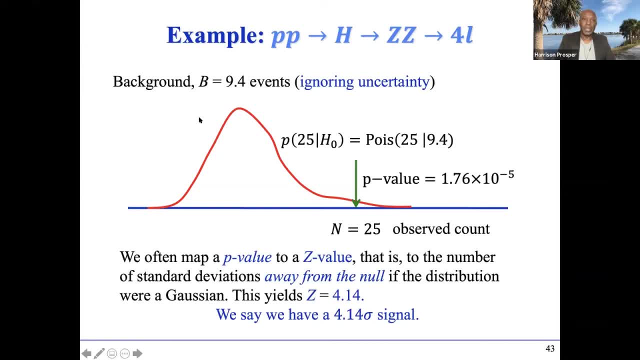 away from the p-value. Okay, so let's say the mean is here at the peak, and assuming this was like a Gaussian, then this green arrow would be some number of ton deviation away from the mean, and that's the measure that we usually find easier to wrap our heads around. 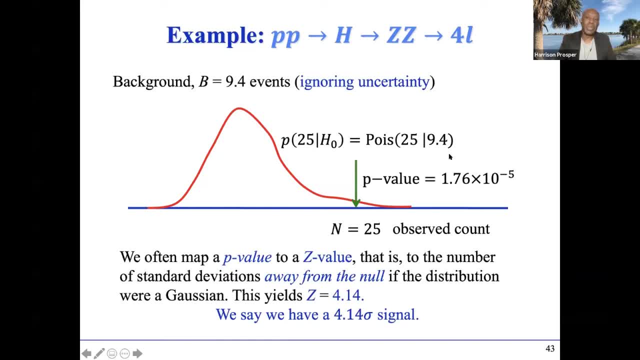 And so what we do is that we simply convert this p-value into the equivalent number of ton deviations. you know, assuming a Gaussian distribution. That's just a convention. There's nothing. there's nothing that's going on between them. Okay, so that's what we do. 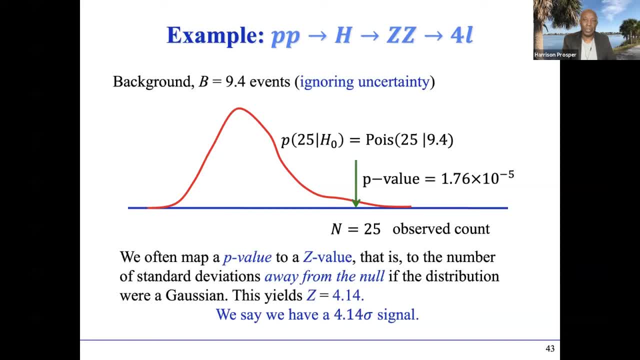 Okay, so that's what we do. There's no necessity for doing so. the p-value on its own is fine, And so if you do so, if you do that, you then find that that this is a 4.14 standard deviation. 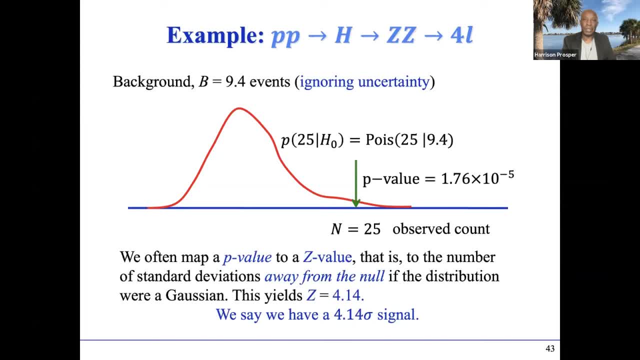 signal So strong evidence that this thing exists, but not- but not yet- the threshold that we use to declare victory. ie, a discovery has been made, But this does not account for the uncertainty in the background. Okay, That's the p-value. 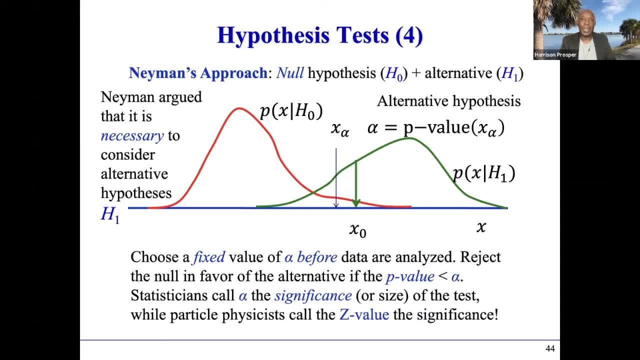 So that's, that is Fisher's approach, which we of course use, But according to Neyman that he said that does not make any sense. You have to have two hypotheses, he says You need to have a null hypothesis by this red curve. 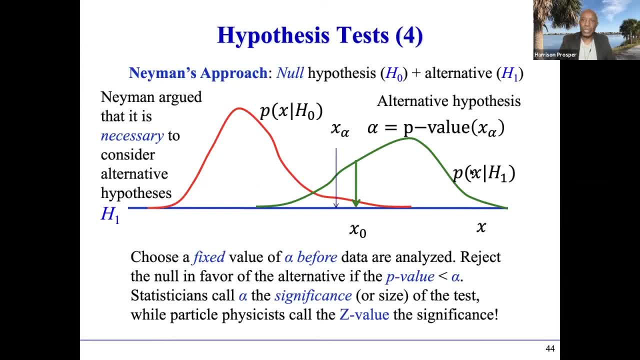 and you need to have an alternative hypothesis. So this would be this green curve, would be the hypothesis that let's say again: we're looking for supersymmetry, We, we. you know this is 20, In 2040, the MSSM is really dead, the NMSSM is dead, but there's a new variety of supersymmetry that is still alive. 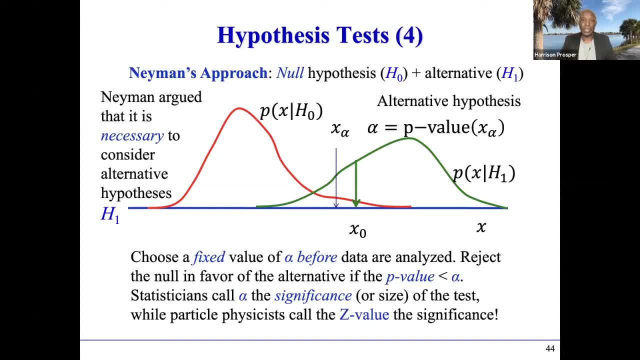 and it makes a definite prediction for some quantity, some observable, and it is this green curve here. okay, So these are two hypotheses: the no SUSY and this is the hypothesis that there is supersymmetry. okay, Okay now. so what Devin says that we should do is that we choose a threshold: x, sub alpha. 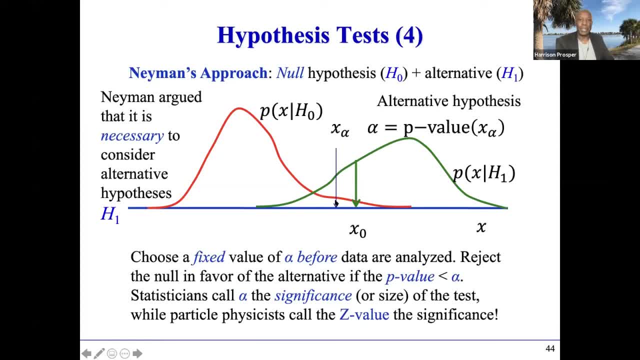 where alpha is a particular number called the significance or size of the test, and that is chosen ahead of time, before you do the experiment. Okay, now suppose, and so for us we would choose alpha if we really want to make a decision. 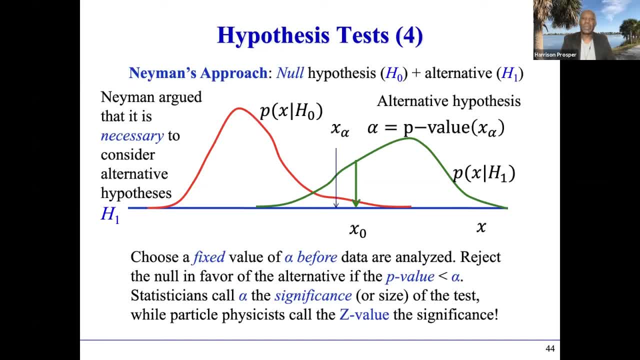 if we really want to make a discovery of supersymmetry and say yep, there really is supersymmetry, we would choose our magical threshold of 2.7 times 10 to the minus 7.. So whatever x alpha corresponds to that tail probability. from here onwards, we would find x sub alpha. 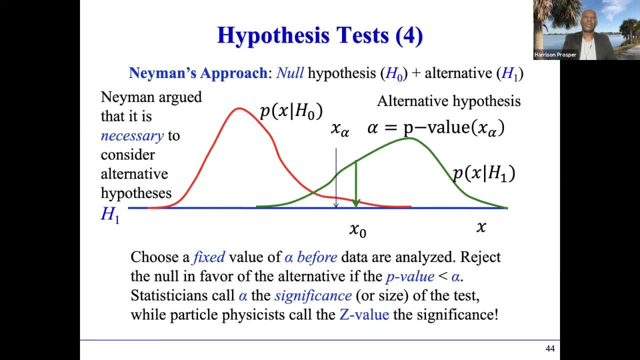 Okay, we do the experiment and lo and behold, we find that we get a result x sub naught that is actually bigger than x sub alpha. Well, according to Neyman he said: well then, you should reject the null hypothesis in favor of the alternative. 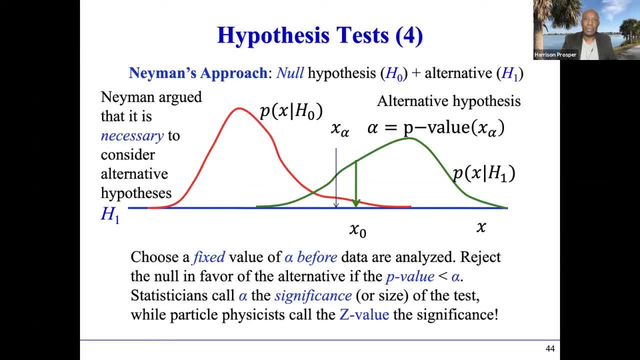 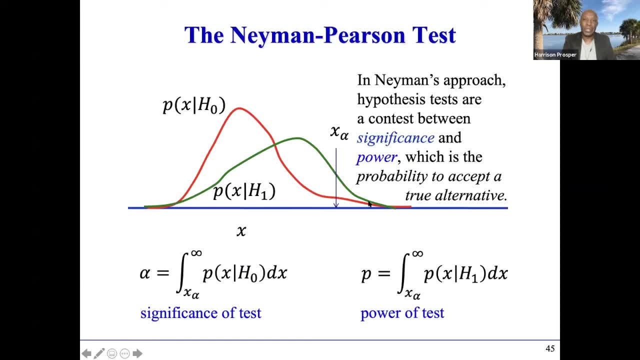 And that's it. So in Neyman's theory there's always a contest between two hypotheses- the null hypothesis and the alternative hypothesis, And what he said was important to do was to, in addition to computing this number- and, as you can see, this is basically like a p-value, except here it's called alpha. it's a fixed threshold. 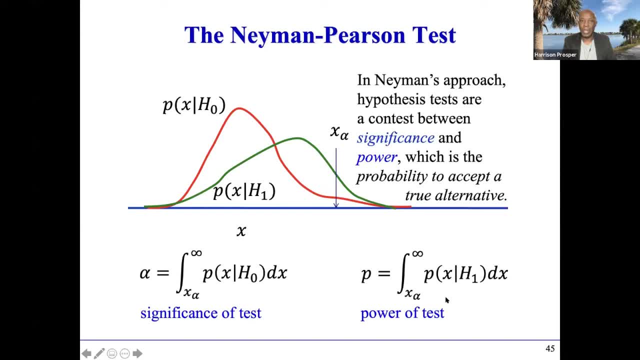 You should also calculate this number here, which is called the power, And if you think about what it's saying, this number is really the probability that you would actually accept the alternative if it were true. Now, remember, we do not know which is true. 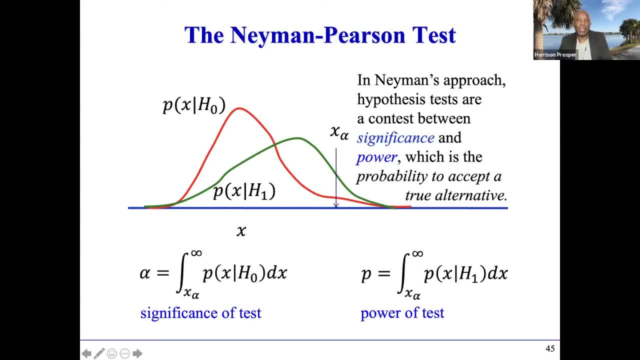 We do not know whether it's h naught, nor do we know whether it's h1. And in fact it could be. neither We don't know. But if in fact h1 is true, ie the Suzy hypothesis is true, 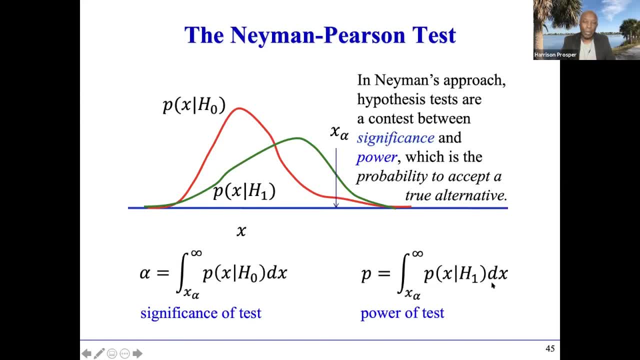 then this number would be the probability to accept it, if it were true. Okay, so this is Neyman's idea. Neyman's idea is that you compare two hypotheses and you for a fixed alpha. so you keep alpha fixed. 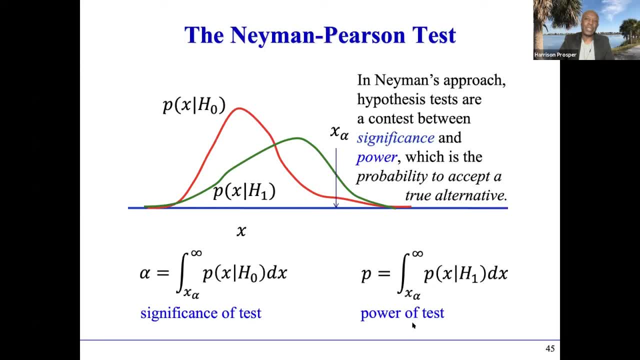 what you want to do is design your analysis to maximize the power, the power of accepting the alternative hypothesis. That's the idea, Whereas in Fisher's way of doing things, there is no alternative, There's just the null hypothesis, And if your p-value is small enough, you reject the null, and that's it, you're done. 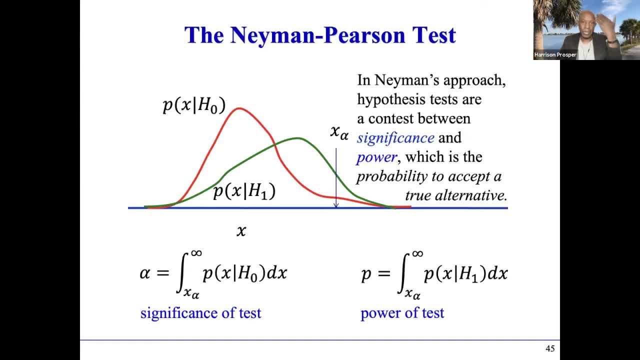 But here you really are comparing very concretely, you know, say, standard model prediction and a very well-defined model, for example supersymmetry, right? I mean, as was stated by the previous speakers, it's really necessary to test real models against data if you want to make real progress. 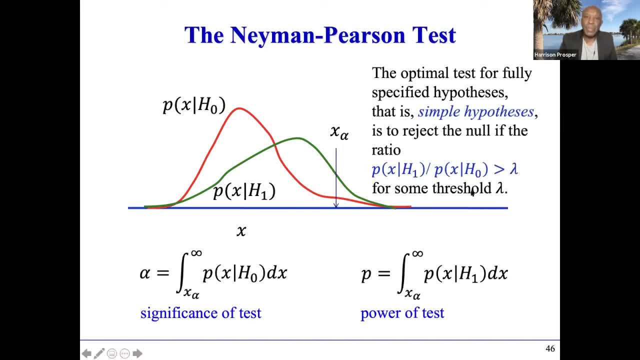 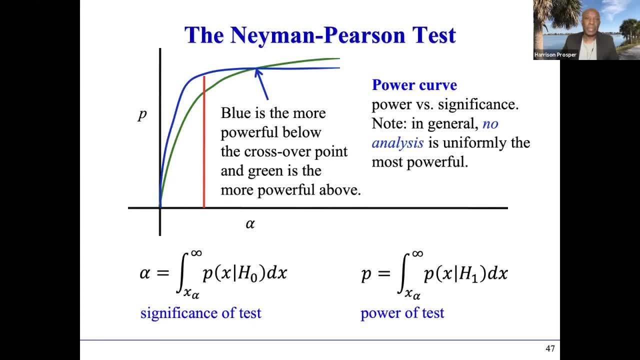 And that's what one should do. And Neyman constructed a particular way of doing this test, which I don't want to talk about right now. I just want to make a point here: This quantity, this power of the test is a very good way of comparing analyses. 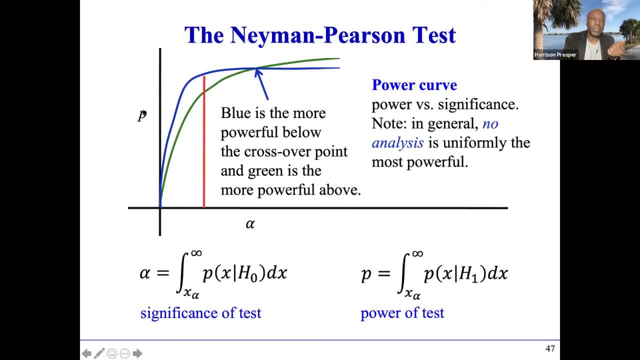 So let's compare. let's draw this curve where we have power on one axis and alpha on the other axis. Now, in principle, what everyone should do is you construct an analysis and you compute for different alphas. right, You compute the power for some alternatives. 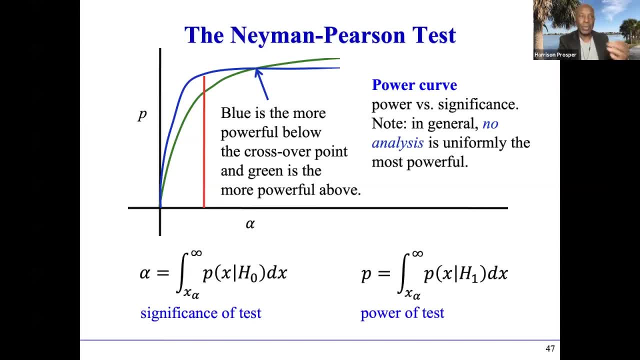 So we're all interested in looking for Suzy right, And let's suppose we want to test the N-MSSM. Then you design an analysis and you say, OK, I'm going to compute the power of my analysis for different choices of alpha. 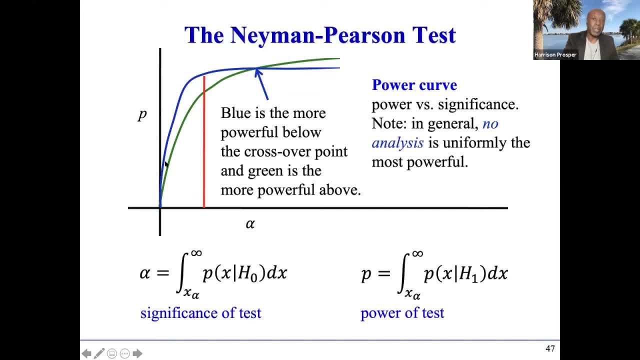 Let's suppose I end up with a blue curve. That's my analysis. OK, I've not yet decided where I'm going to set my threshold, but I've computed this so-called power curve. And let's suppose someone else decides to do their own analysis, looking for the same models, let's say the N-MSSM. 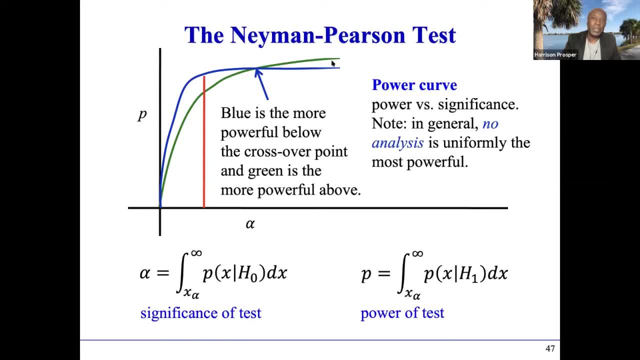 And their power curve is the green curve. Now, what you notice is this: is that if we were to agree to choose a threshold for alpha, say up here, then the green analysis is the more powerful, That is, it is the more likely to accept the true hypothesis, the alternative hypothesis, the Suzy hypothesis, if in fact the hypothesis is true. 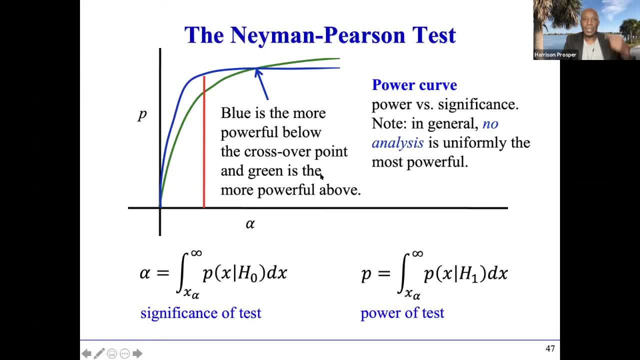 If we chose a threshold here and did the experiment, then that analysis is more likely to basically accept the true hypothesis. On the other hand, if we were to choose a more stringent criterion for alpha- let's say you know a three sigma, four sigma, whatever- then it turns out that my analysis is the more powerful if we were to choose this particular threshold. 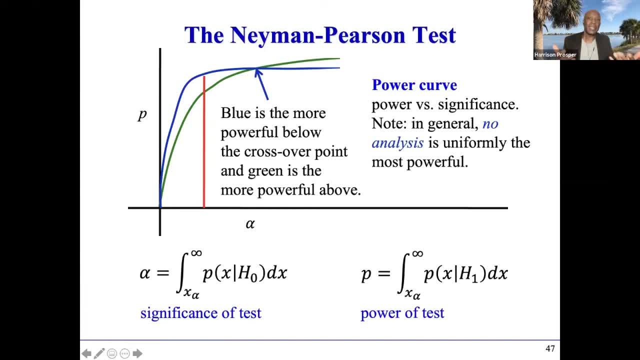 And so is it generally the case that there's no single analysis. that's going to be the most powerful everywhere, And really what one needs to do is to decide on the threshold, which of course we do. We have, you know, three times the deviations, let's say evidence of something going on. 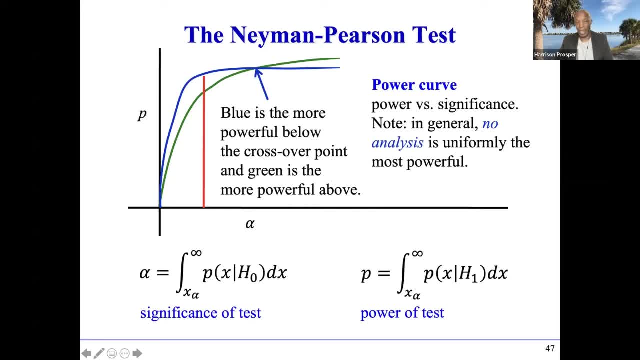 Four times the deviations- perhaps something with more evidence- and five times the deviations being a discovery. We choose our thresholds and then what we want to do is that we want to design analysis and we want to arrive at analysis that is the most sensitive. 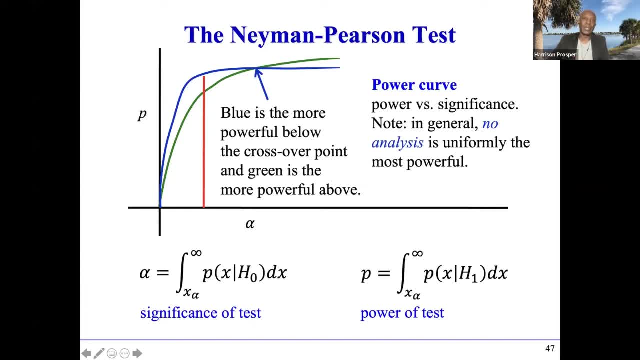 if you like. that's the way we like to state it- the most sensitive with respect to a particular hypothesis that we are trying to actually test, And so this is what's done, And essentially we do that all the time right. 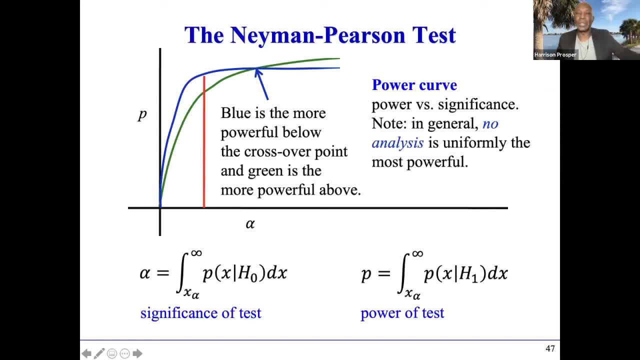 We design and we optimize it for a particular, in this case a particular SUSY model. Of course, there this is a lot more difficult in practice, because these SUSY models, as we have learned, contain lots and lots of parameters. 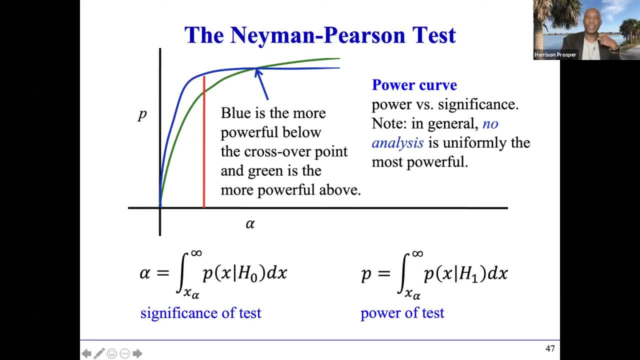 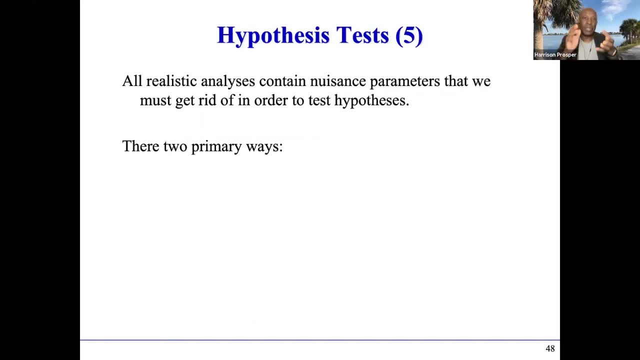 And sometimes this is very difficult to know how really to optimize analysis when you have such a situation. But the problem, of course, is that all realistic analyses contain useless parameters, sometimes hundreds of these things, And we have to get rid of them if we want to test hypotheses. 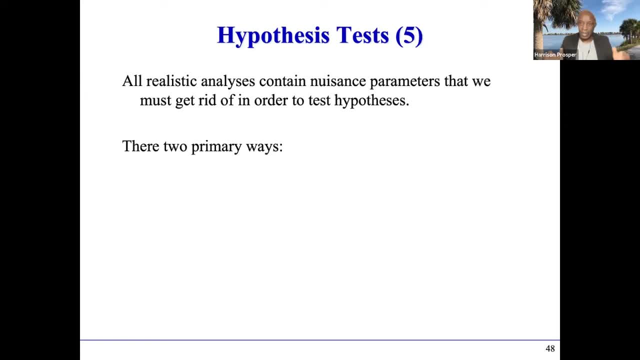 If I really want to test the NMSSM- let's suppose you know, let's think about the MSSM, right? This is this thing has? this beast has more than 100 parameters And if I wanted to do an honest test of this, I would have to look at many of these parameters. 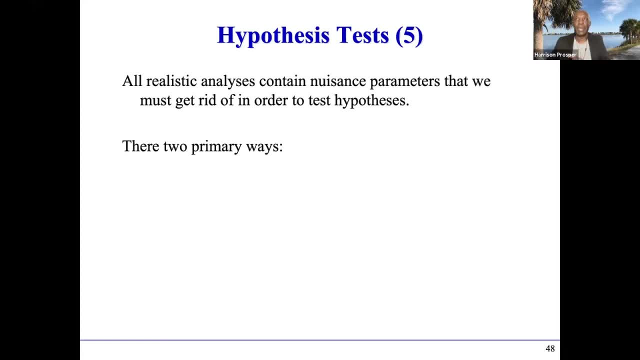 And but, but. but maybe you know, maybe I only care about a subset And that all the others in this context would be nuisance parameters, in addition to the nuisance parameters which are purely experimental. Right, I only care about tan, beta and a few other parameters, and all the others I simply don't care about for now. 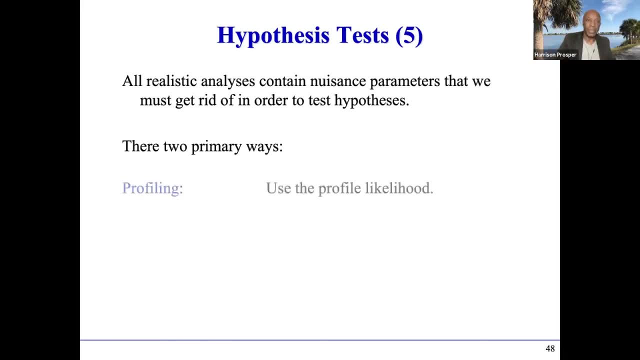 I need to get rid of them somehow, And there are two ways to do this. One is- we've already seen- profiling You, you, you fixed the particular parameters that you care about as some particular values And you maximize all the- you know- respect to all the other parameters. you go to another point in the 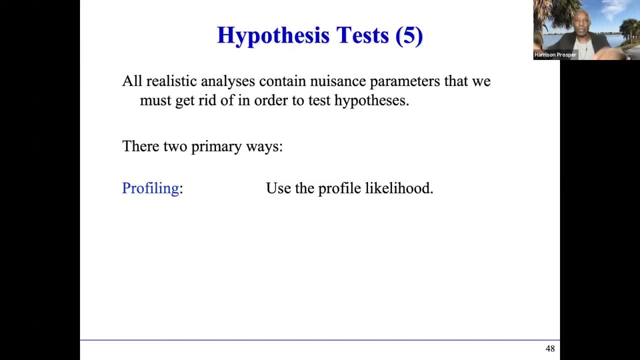 parameter space that you care about, maximize respect to all the parameters and that way you map out a function that called the profile likelihood, that depends only on the parameters that you care about And that, as I said, this is true whether the parameters are theoretical. 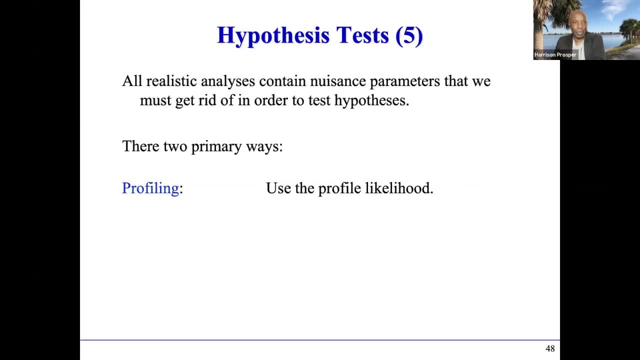 parameters in a model, or they are parameters which are purely experimental. That's the way one gets rid of those parameters in this approach. The other approach is- as we shall learn shortly- is to integrate over those parameters that you don't care about. So again suppose, let's take 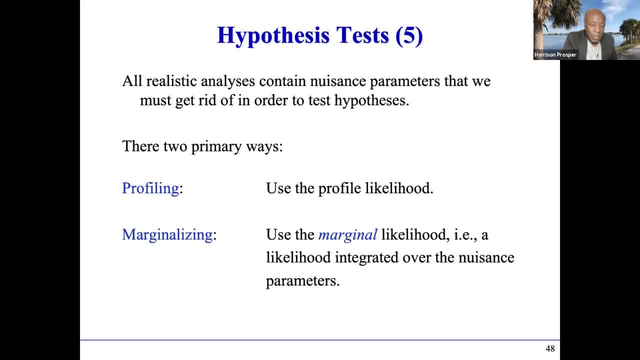 for example, something that's more realistic: the P-MSSM right. That's a proxy for the MSSM, in which the number of parameters has been reduced from whatever it is: 120 down to 19 or so. So 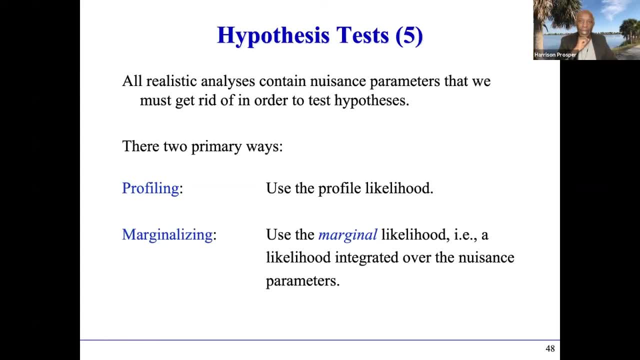 suppose, of those 19 parameters, I only care about five. I really don't care about the others. Well, the others then would be nuisance parameters that I would get rid of by integrating over those in my model, my likelihood model, or profiling them away in addition to all the other experimental 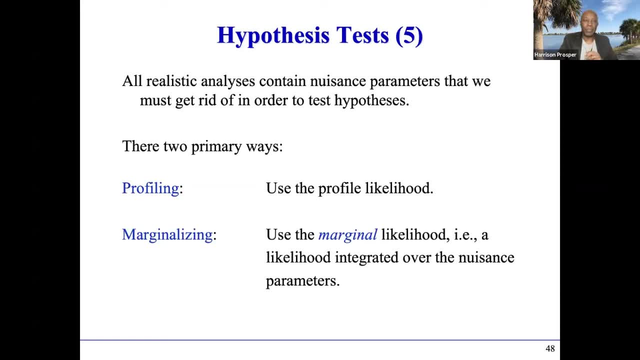 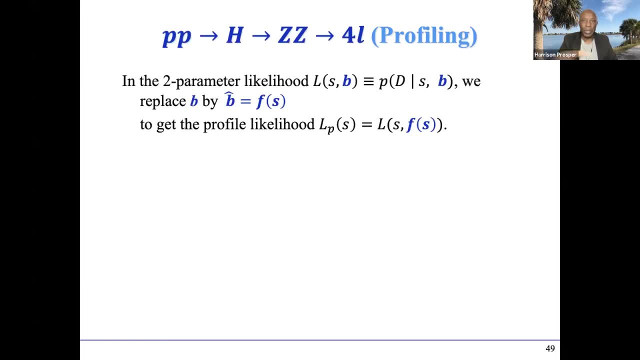 parameters. So those are the two ways of doing this. Now, in the frequentist analysis, profiling, of course, is the way things are done, And so let's do that. Let's profile, use profiling to get rid of this as before, And so that's what we're going to do, And so let's do that, And so. 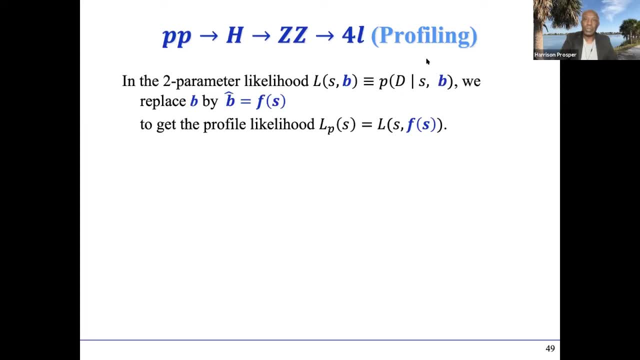 let's do that, And so let's profile, use profiling to get rid of this as before, And so that's what we did here. This is the likelihood which depends only on S and B. now, because the data are fixed numbers, We fix S and we find the best fit value for B, And we do that for different. 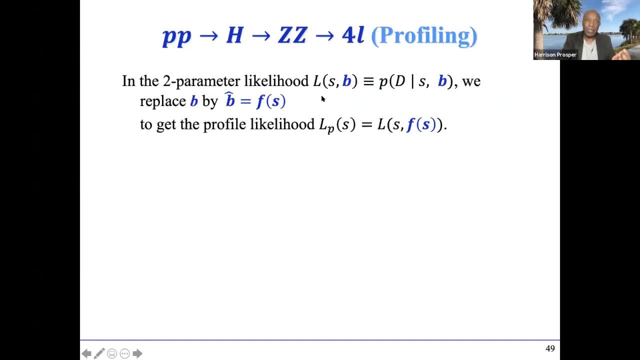 values of S, And so this maps out a function right. So B is now a function of S, B hat, And now we replace B, the true value, by this function, And so we arrive at a function as before, which 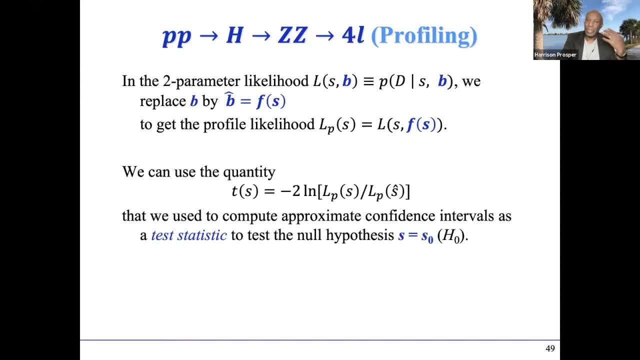 depends only on S, And what is interesting is that we can use the same statistic that I showed you before. Remember we used this statistic before to work out an interval for the signal or maybe an upper limit, if you're searching for some new physics. So we can use the same statistic as before. 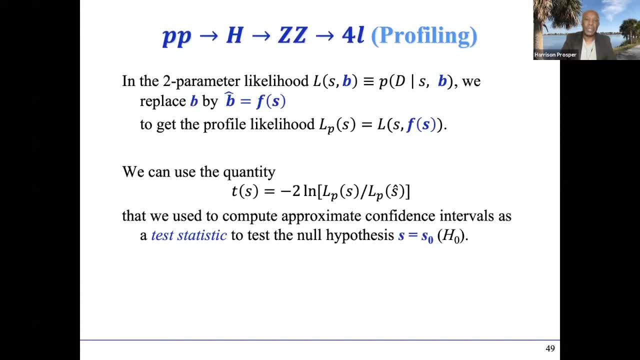 to test the null hypothesis. However, because of this, we can use the same statistic as before to test the null hypothesis, Because we've replaced the true value of the signal, of the background or the other parameters with estimates thereof. then this test is approximate. But again it turns out that the 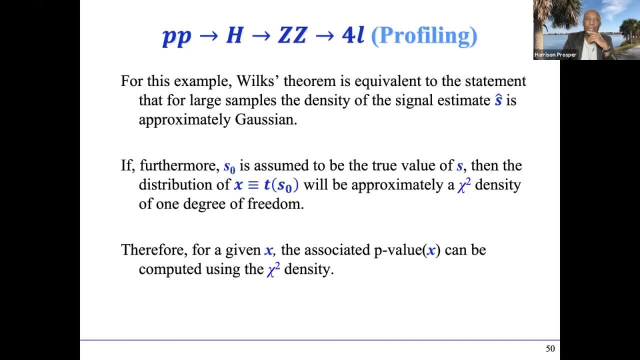 tests are still reasonably good. So how do we test this? Well, actually it's very easy, because this theorem that we talked about briefly in the first half, Wilk's theorem, says that this quantity t minus twice the profile of the likelihood ratio, is just a chi-squared. 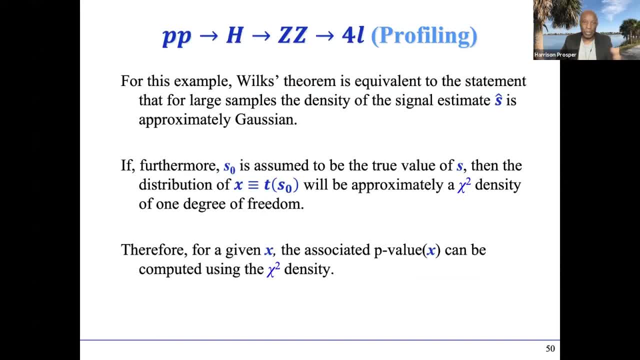 variable if certain properties are realized, And so I can test particular values of S0 by using the chi-squared density. I can compute p-values, since I know the distribution of t right. I can compute p-values, since I know the distribution of t. 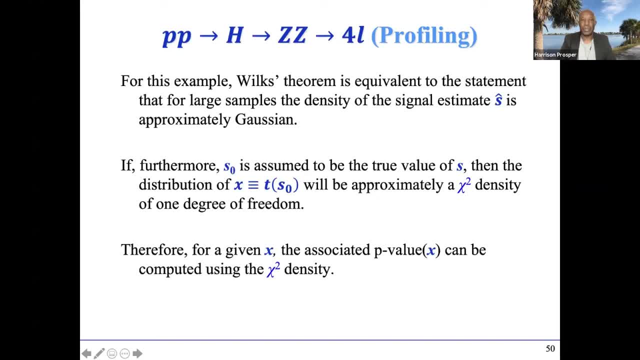 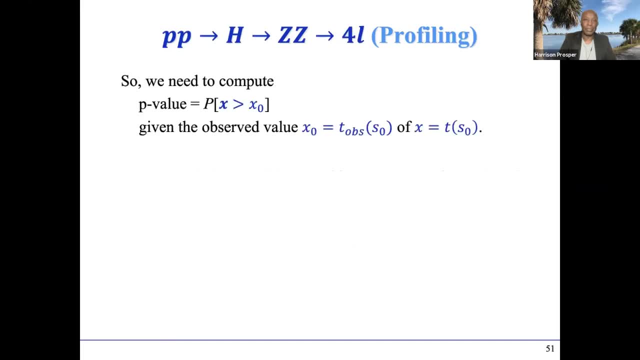 I can compute the tail distribution because I know the distribution of t. It is just a chi-squared density in this particular case, And so all we need to do is to compute the p-value. say: what's the probability that x- in this case a chi-square- is bigger than x0? And then x0 is. 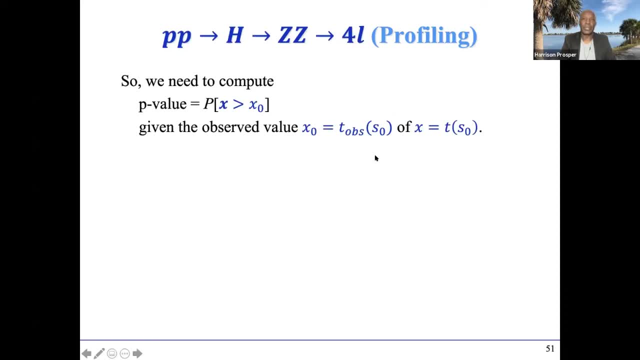 just the observed value of this quantity, Right, That's all it is. And then I simply ask: is my p-value less than alpha, the threshold that we've already agreed upon? And if it's less than alpha, then I reject the hypothesis. S equals S. 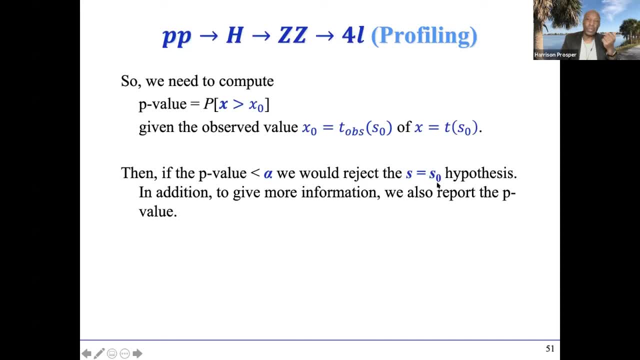 dot, In particular, if S dot is equal to zero, ie background only, I have a way to reject the background only hypothesis. Okay. So just to recap, we can use the same statistic that we use to create an interval, whether it's. 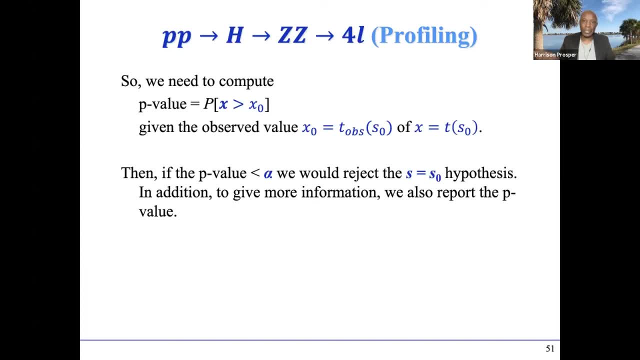 a two-sided interval or an upper limit or a lower limit. We can use the same statistic to test particular hypotheses, because we know the distribution of the statistic t. It is a chi-squared density for this particular case. Therefore, I can simply choose to compute the p-value of t. 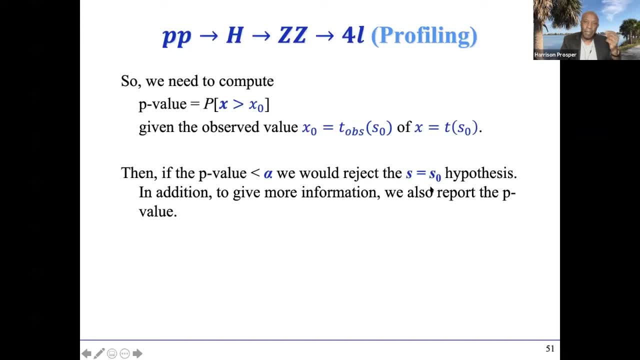 this number at a particular value of S that I want to test. I want to test, let's say, S equals zero, So I plug in zero here, I compute this number and then compute the p-value, And if this p-value is, 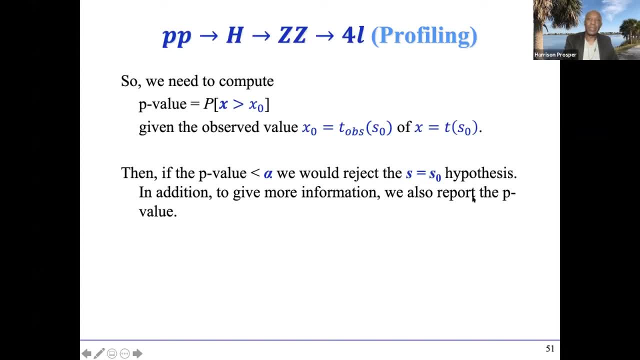 smaller than the threshold that I've agreed upon, then I can reject the. S equals zero hypothesis. And what is interesting actually is that because this is a chi-square, So remember, a chi-square is basically x minus mu over sigma, all squared right If you think about Gaussian. 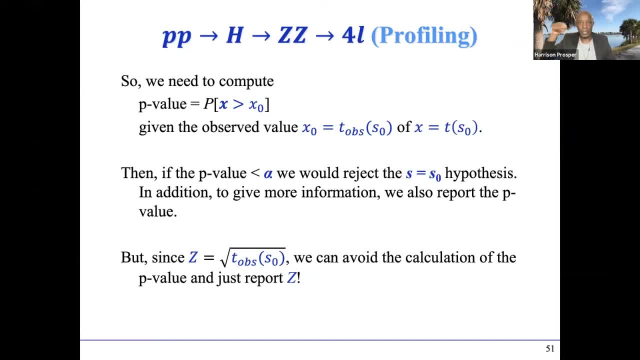 a chi-square is x minus mu, where mu is the mean over sigma, where sigma is the standard deviation, all squared. Therefore, if I take the square root of that number, then that tells me how many standard deviations z. I am away from the mean, And so all I have to do to calculate the z-value is simply: 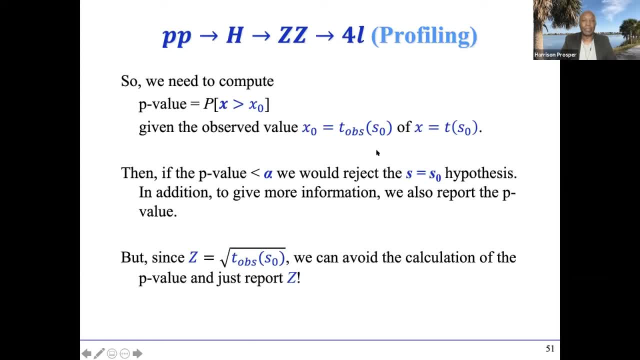 take the square root of this number And then I can take the square root of the z-value and I can just report z. Okay, so let's just again just to summarize. We use the same statistic, t. Remember t is equal to negative twice the log of the profile likelihood ratio. 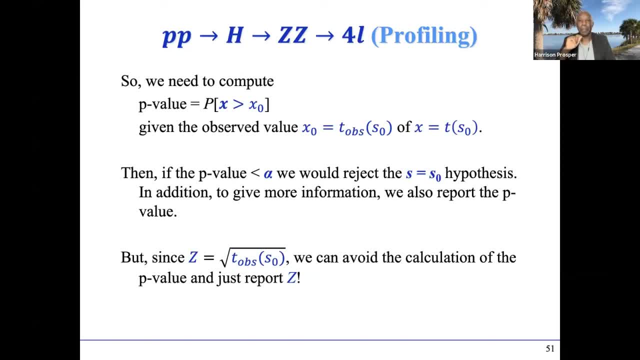 L profile S over L profile S hat. But since I know that negative twice, the log of that likelihood ratio is basically a chi-squared variable. that means I know the distribution of that quantity t. It's just the chi-squared density. So what I can do is I can plug in. 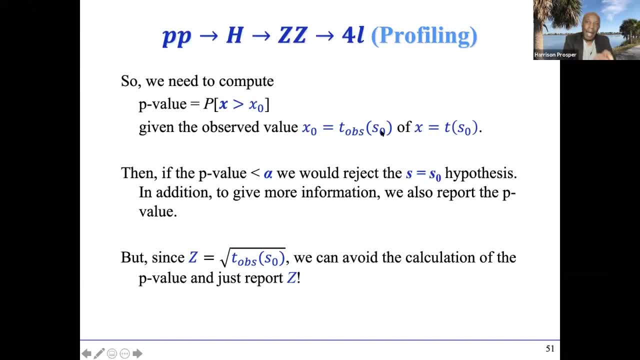 to t the particular value of the signal I want to test. ie S equals zero, ie there's nothing going on. That's interesting. And then, having computed t at S sub zero, I can then calculate the p-value, the probability that I get a value of x bigger than x naught. 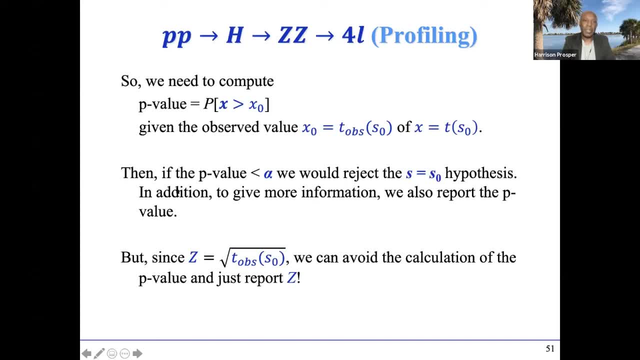 ie this thing, And if I find that my p-value is less than this threshold, ie smaller than that threshold, then I can reject the S equals S naught hypothesis. And that's essentially what was done in the discovery of the Higgs boson, except of course our alpha was very small. 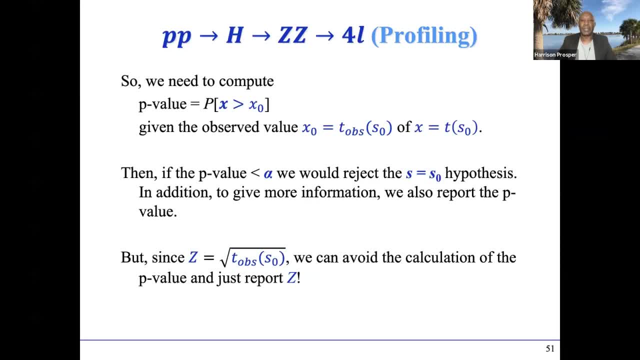 It was 2.7 times 10, to the minus 7, 7.. And that corresponds to 5 sigma. ie z would be 5, sigma would be 5.. And that's the way this is done. Now, of course, 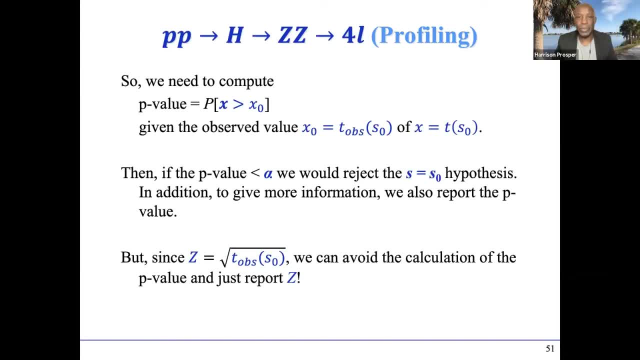 it may well be that you compute this likelihood ratio and you find that unfortunately it doesn't have the distribution of a chi-squared variant, in which case things get a bit more complicated. But to the degree that that's true, then things are very easy, since you know. 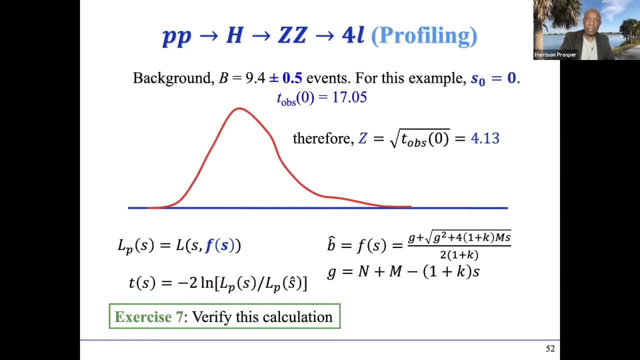 the distribution of that statistic, And so let's just do that. So now we take into account the uncertainty right And remember what we do is that we are going to replace the true mean b by the estimate of b as a function of S. Here it is. 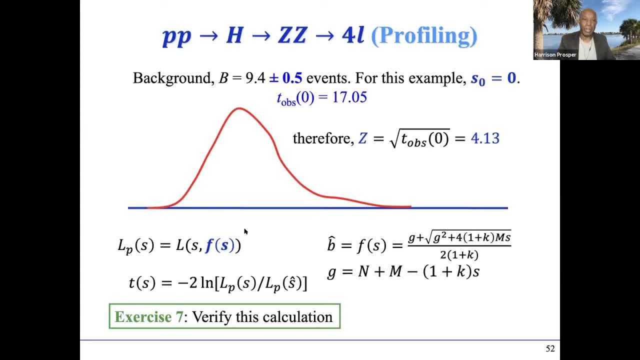 okay, right here, That's profiling things away. And here is this amazing statistic. And now I'm going to test the hypothesis that S is equal to zero, ie that the signal is zero And you can see that the signal is zero. And then I just take the square root of this. 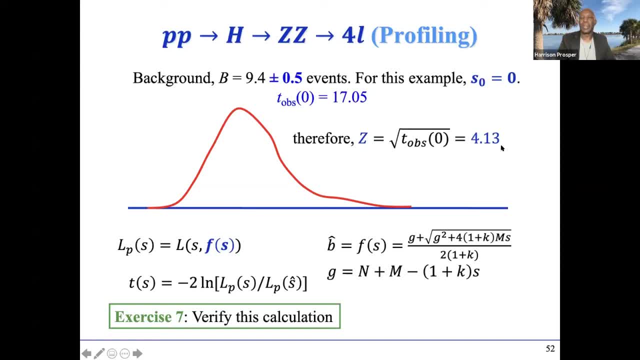 because this is basically a chi-squared variable. And then this tells me that the known standard deviation away from the background is 4.13.. And, by the way, you notice that when we did the computation in the first part, we found that this number was 4.14.. So it turns out that 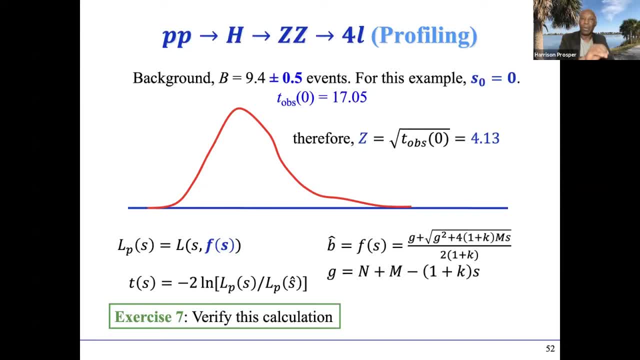 the background has very little effect actually on the Z value. There's a lot more effect on the Z value, the significance, if you scale the signal. For example, if you rewrite the signal as mu, a signal, strength times, a signal, then there's a bigger effect on the significance, ie Z if you have a bigger. 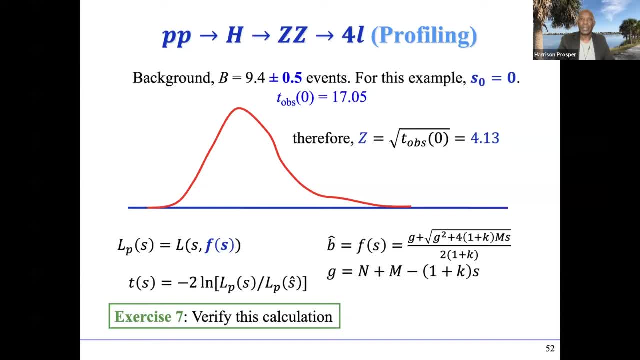 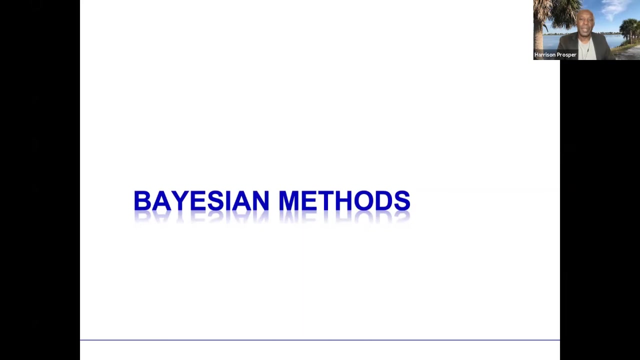 uncertainty on mu. Okay, so here we're simply using the same approach, the same sort of procedure as before, except now we're using the same statistic to test different hypotheses for the signal mean S. Okay, I have to say that many of these ideas are really best really understood by doing little toy. 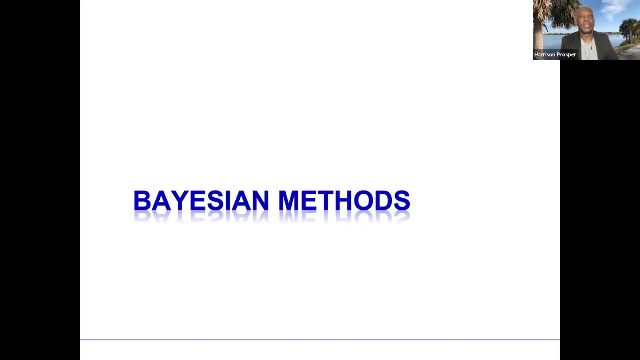 experiments, And so I will at some point write a Jupyter notebook and make it available to students, because it's very good to go through these things yourself to really understand what these things are. Okay, so now we're going to talk briefly about Bayesian methods. So so far, we've been assuming. 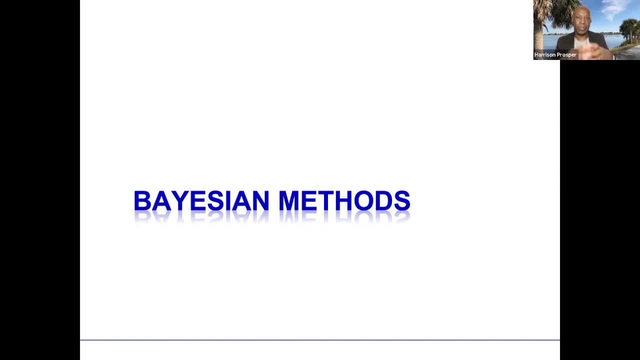 that the interpretation of probability is relative frequency, That's it, Ensembles and so on. That's what we've been assuming, But now we're going to assume that we are talking about methods in which probability is interpreted as a degree of belief. 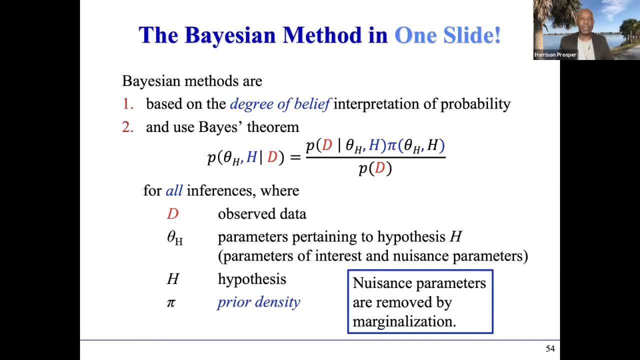 So here in one slide is the whole of a Bayesian approach. The Bayesian approach is based on Bayes' theorem. that's why it's called Bayesian approach, right? it's always used in all of the inferences, And so let's go through this bit by bit. So this term 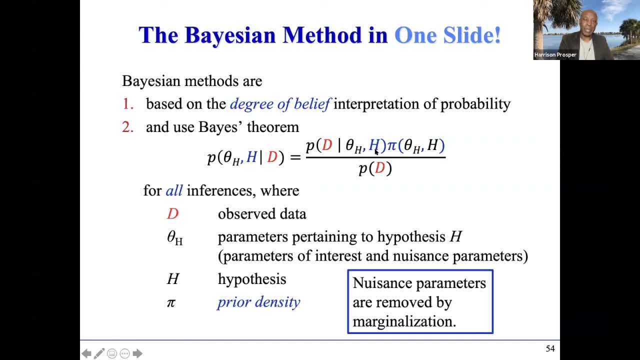 here the probability of d, given theta sub h times h. this, of course, is the thing before that we called the likelihood, since we've already plugged in data into it, And what we're assuming here is that we're assuming that we have different hypotheses or different theories, right? So h? 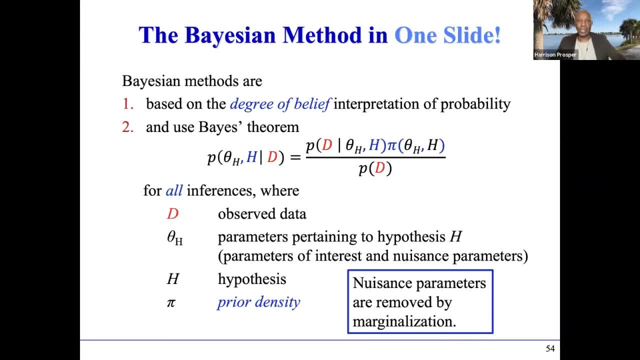 could represent, you know, one Suzy model. another value of h could represent a different Suzy model. or h could represent, say, a pattern distribution function model. you know, one could be MMHT, one could be NNPDF, whatever it is. So h is a discrete label that labels different theories. 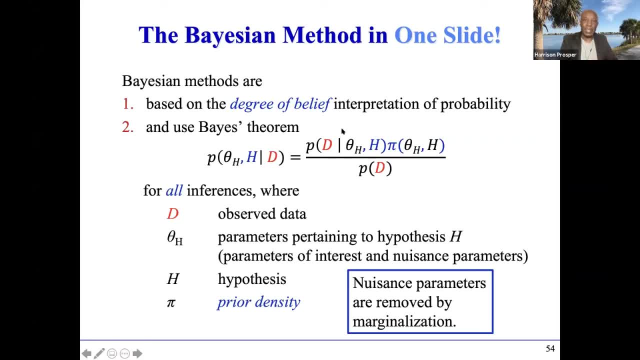 or different models, and each one of these models has its own set of parameters, which could be quite different, right? I mean, the NMSSM, you know, has different sets of parameters than the MSSM, and so on. So we presume that we have this, okay, and we know how to construct this thing. 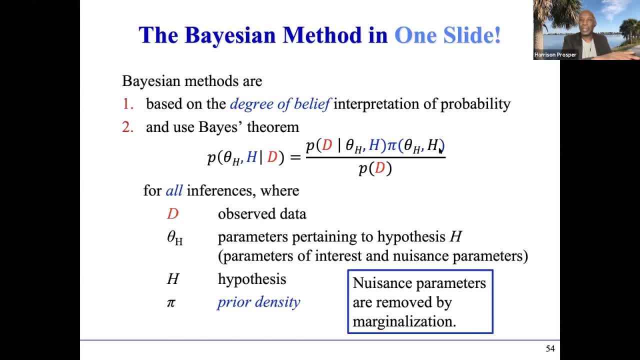 Then there is this thing that doesn't appear in the frequentist approach and that is a prior probability, a prior density, in this case, for each of the different hypotheses and different parameter sets. okay, And then we normalize this with this quantity of probability of d. 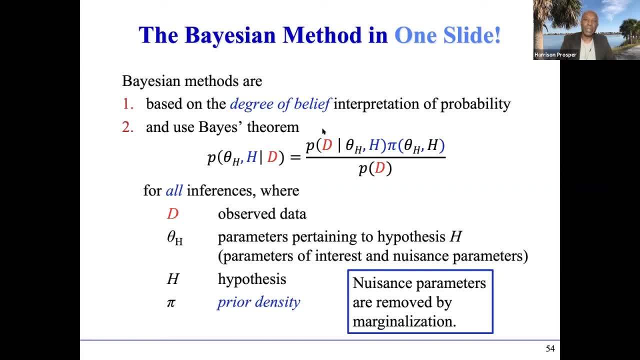 and this is nothing more. this thing in denominator is nothing more than the sum over all the possible hypotheses that we want to entertain, all theories, and integration over all of the parameter sets. So for example, let's suppose I the LAC. 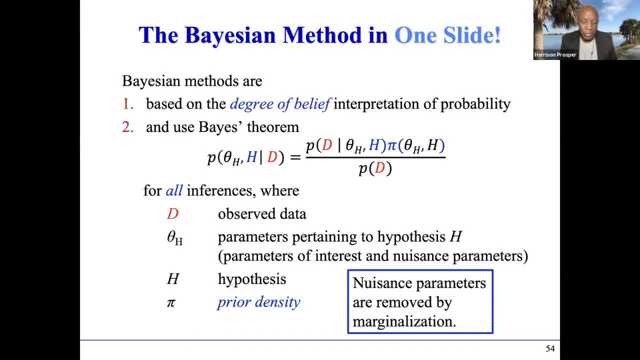 I'm not sure which part of distribution function to use. There are three. right There's CTEC, CT, you know whatever it is now. I have MMHT, I have LNPDF. I have these three different part distribution functions. 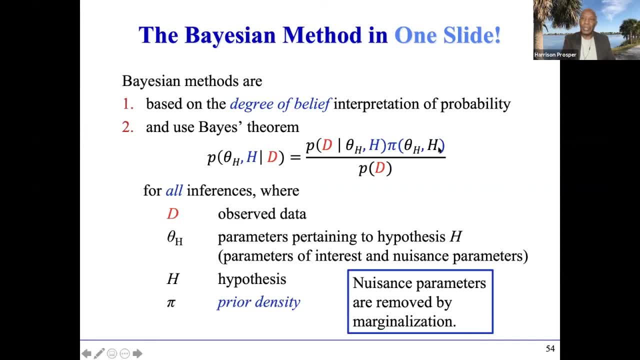 I want to use. So H would be basically have three numbers: one, two, three- one for each of these PDF sets And each of them has all set of parameters and I want to basically take those into account. So this is a very general structure here. 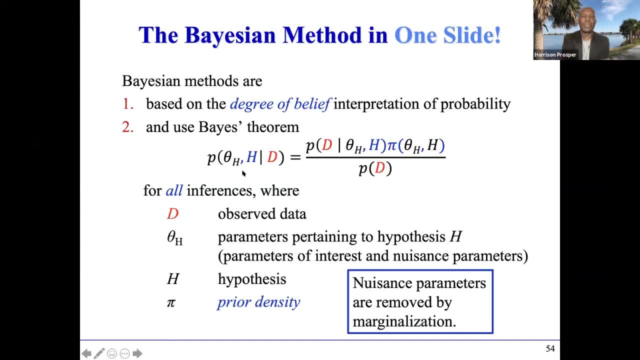 but then what happens, of course, is that Bayes' theorem allows you to invert the probability, And so you can then ask the question: what's the probability for a particular set of parameter values, for a particular theory, a particular hypothesis? H, given the data that have been acquired? 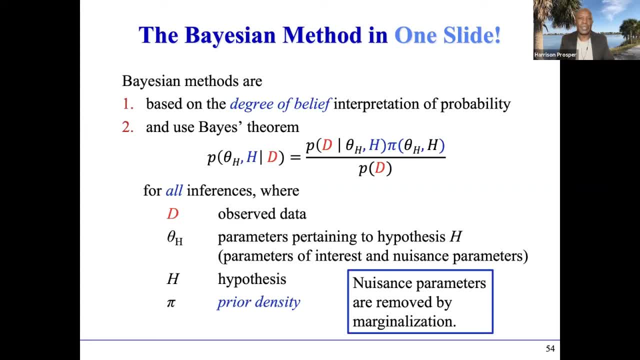 And that's it. So this is, this is the whole of Bayesian analysis in one slide, And, of course, you can marginalize, you can integrate over the parameters and theories that you don't care about for now, And we'll see how that works with our simple example. 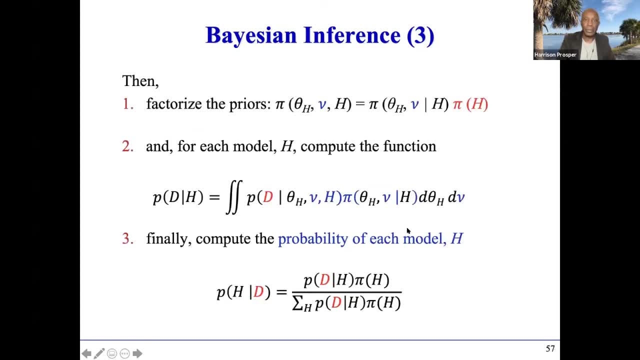 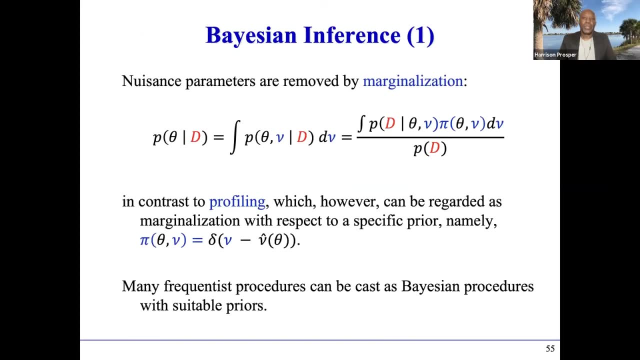 Okay, So let's suppose now one has done all this. Typically, typically, of course, these parameters split into two pieces. There are pieces theta, that are the parameters that you care about, parameters of interest, and nu are the parameters that you don't care about. 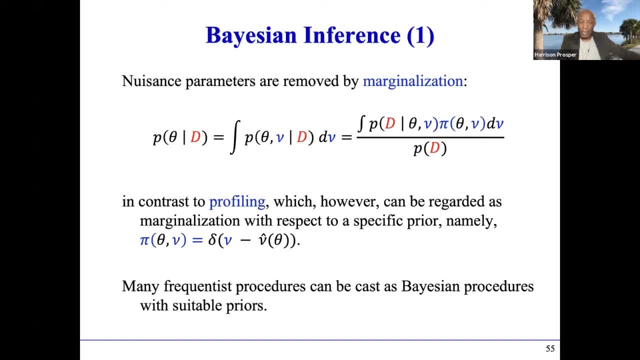 And, as I mentioned, those parameters that you don't care about right now, could include both parameters that are experimental in nature, which are energy scale, the figure efficiency, the whole bunch of things like that- scale factors of various kinds, And it could also include theoretical model parameters. 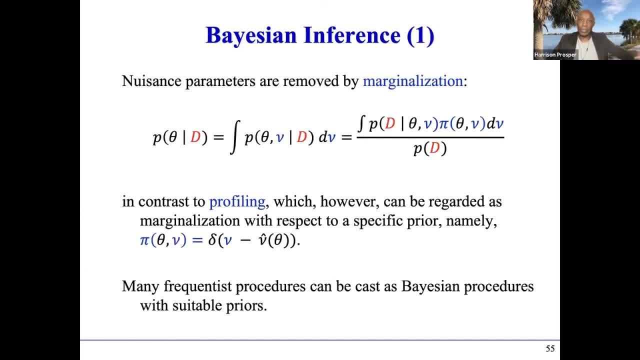 that you currently are not interested in, that you want to integrate over, And so once you have the thing, you can integrate over all the parameters that currently you do not care about, to arrive at a function that only pertains to the parameters that you do care about. 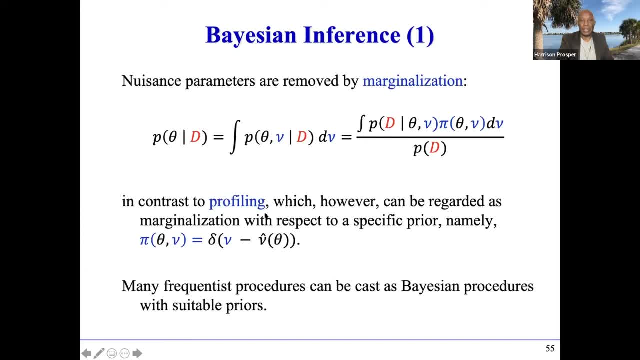 parameters of interest And in fact you can think of profiling right as just a Bayesian procedure in which you've chosen a prior density. that looks like this, where nu hat is the maximum likelihood estimate of every nuisance parameter, given a particular choice for the parameters of interest. 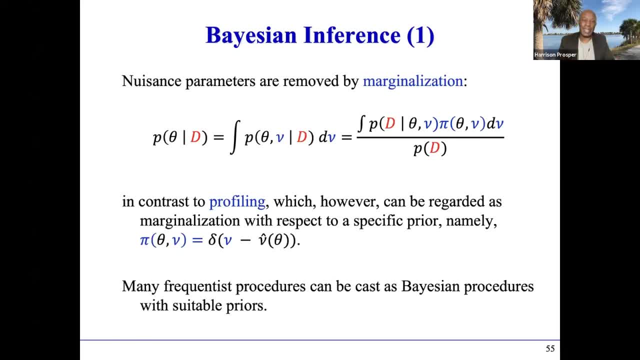 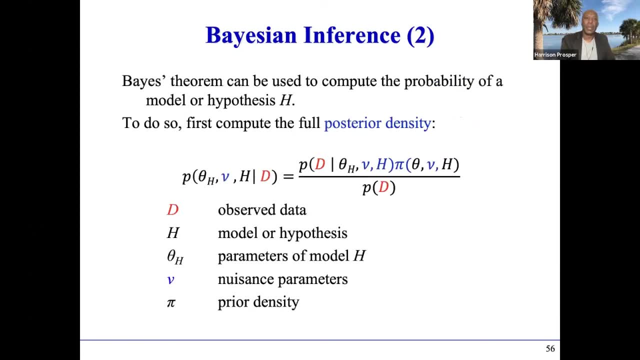 And so, in fact, it turns out that many frequency procedures can be recast as Bayesian procedures with suitable prior probabilities. Now, one of the things which I find particularly amusing is that Bayes' theorem can be used to compute the probability of a particular model or hypothesis. 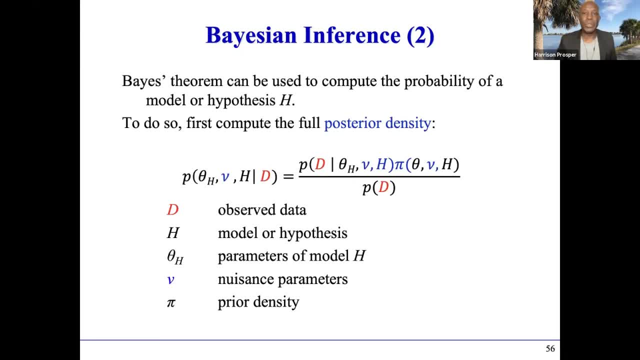 So let's suppose you wanted to be really courageous and use the data at the LHC to decide which of the different PDF models- pattern distribution models- is preferred by the data that we've acquired so far, the LHC. So in this case I would write down the Bayes' theorem. 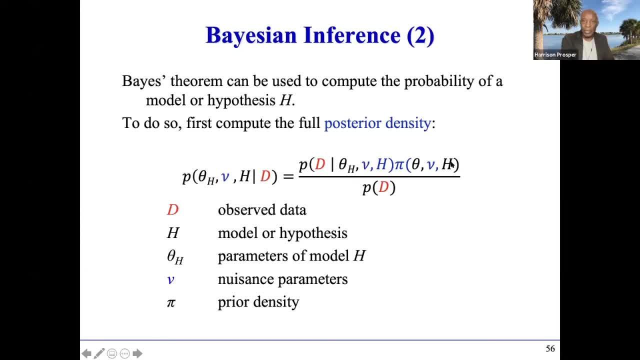 this way where H would label different pattern, distribution, function models from different groups And then PDF, MMHT, CTAC, and each one would have its own set of parameters. So there should be a subscript H here corresponding to the parameters for that particular PDF set. 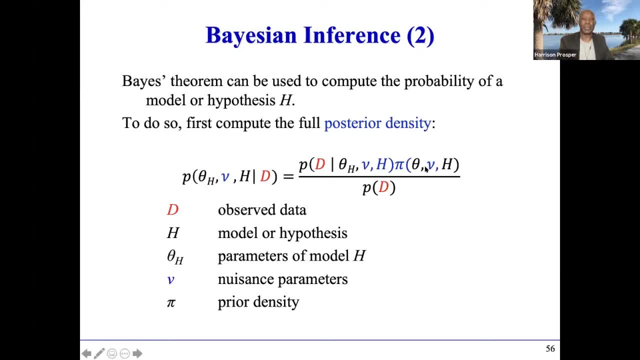 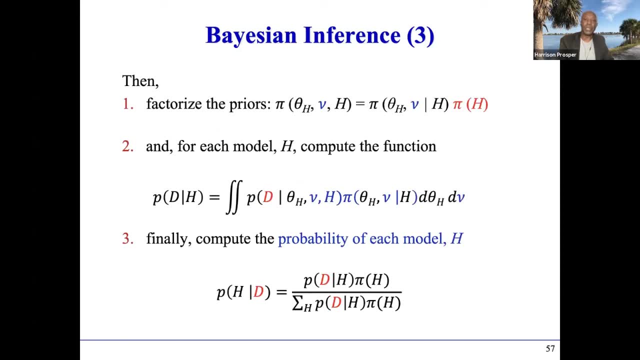 and nuisance parameters. Okay, So let's suppose how could we do that? All right, Well, we could proceed in this manner. We could say: okay, let us first of all factorize this prior, this probability, in this manner: 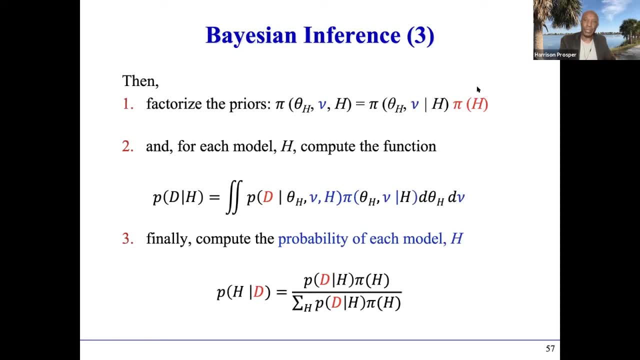 So probability of theta sub H, nu, given H times the prior probability for H, right? So I'm just using probability theory to factorize this thing in some way, Okay, And then, having done so, I could then do the following. I could say: okay, why don't I? 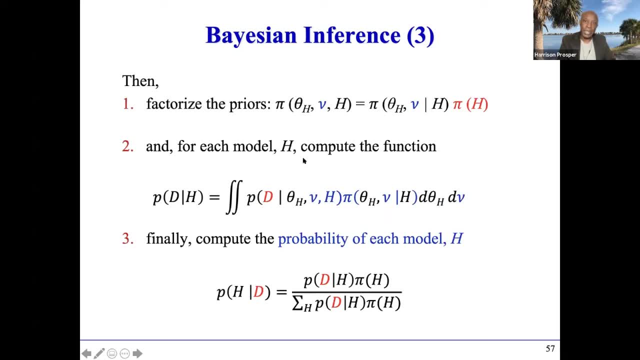 now that I've factorized this prior, let me just integrate my likelihood here. it is with respect to the parameters of the particular hypothesis that I'm going to test, So this could be the parameters. for example, let's say, this is the parameters of the NNPDF. 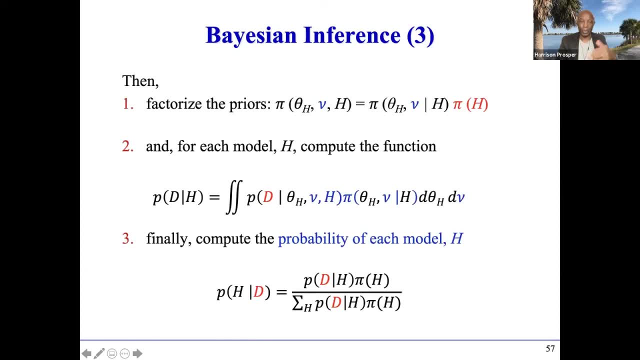 Okay, This is the NNPDF parameterization or the MMHT parameterization, And so now I've arrived at a function that's the probability of the data that I've acquired given a particular hypothesis, a particular theory, particular model, whatever it is. 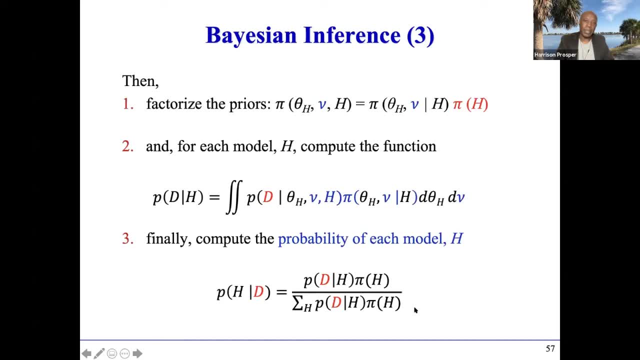 And now I can use Bayes' theorem again. And here it is in its full glory, where I've now integrated over all these parameters of these different theories. And now what I have is a parameter: the probability of a particular hypothesis given the data. 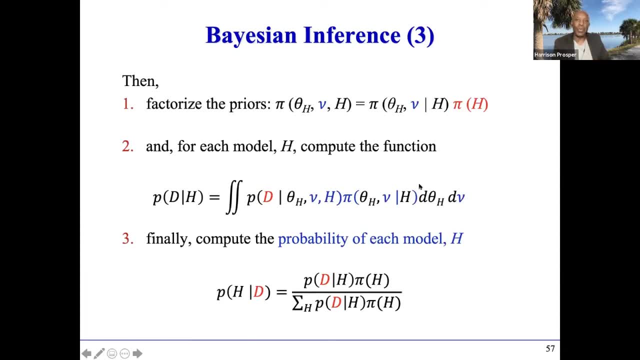 Now, why is this controversial? Well, for several reasons, one of which is that, in order to get arrive at this, in order to arrive at your PhD, you need to specify the prior probabilities that you are going to assign to different theories. 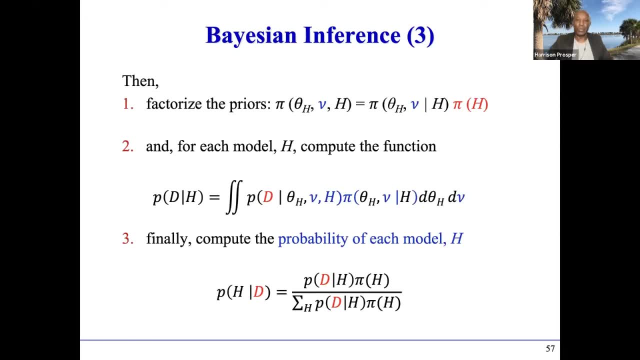 And, of course, depending on who you are, you will have different ideas about what Numbers should be applied for those. For example, you may decide that you are completely agnostic with respect to whether you're going to be using the NNPDF parameterization. 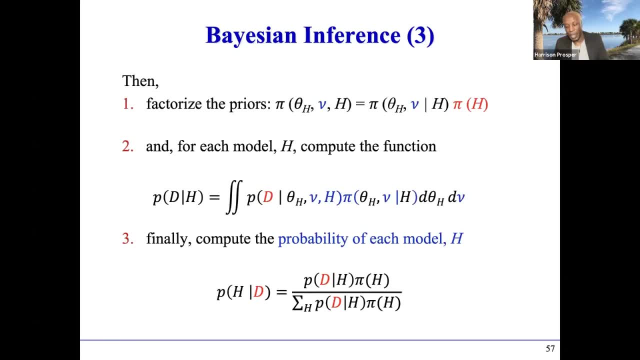 for the partial distribution functions, or MMHT or et cetera, Or you may. there may be two SUSY models that you are trying to compare And you know, in addition to some model perhaps, and you say, okay, so I have these two SUSY models. 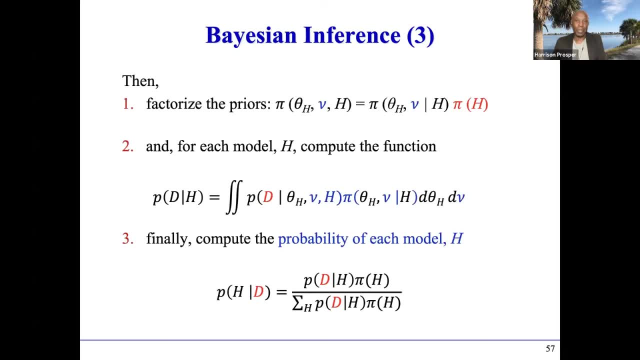 I really have no idea which one is preferred. So I'm going to give equal probabilities, but I'm going to make those properties far less than the probability of the model, because you know the model has been very well tested. So this is where it becomes controversial. 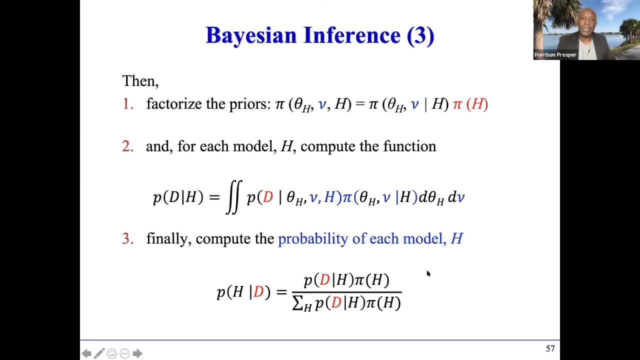 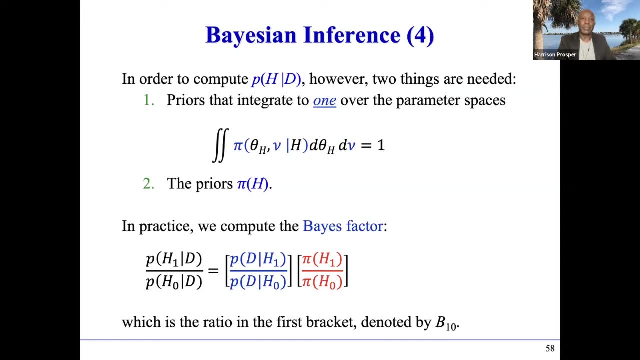 because you obviously will get different answers depending on what numbers you put in for these prior probabilities. But in principle this is the approach. Now there's another. so that's one controversial thing and I'm not saying the complicated case matters. 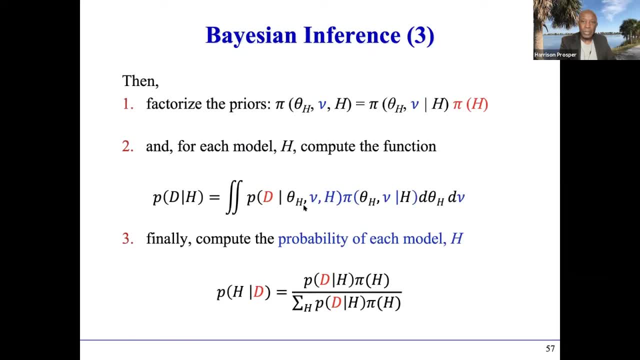 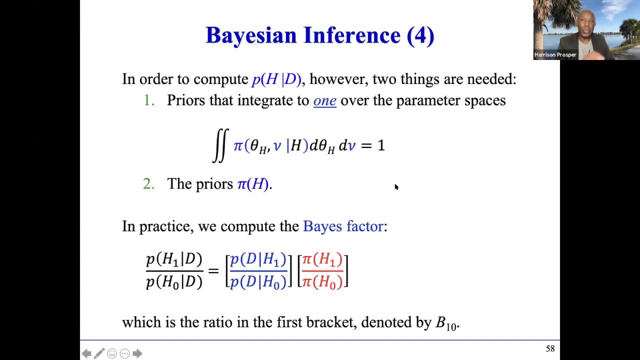 The other thing is this: is that, in order to do this integral, in order to perform this integral- remember, here there's this function, here this prior density that I'm integrating over- In order to do this integral, then two things are needed: 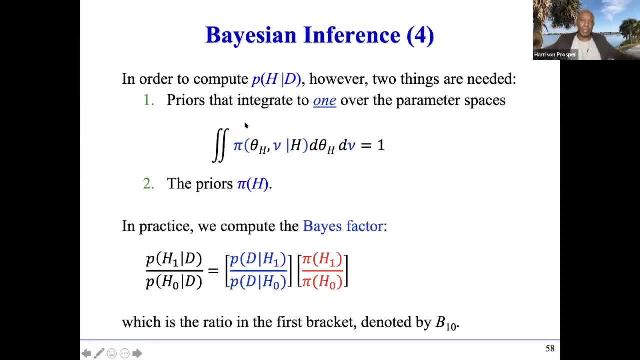 One. if you integrate this function over the full parameter space, it should be equal to one, because that's what probabilities are supposed to do. right, Integrate to one. So that's one requirement And of course, you need the priors, as I've mentioned. 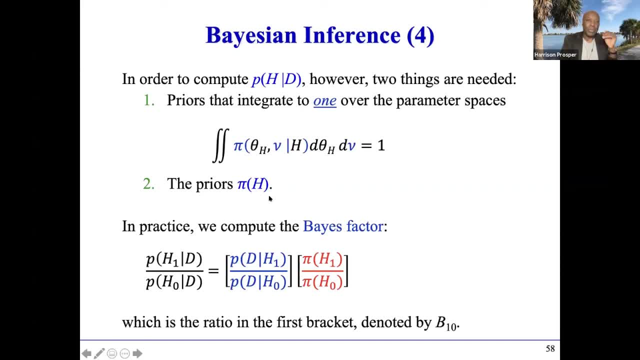 Now. so, because of the controversy about choosing priors for different theories or hypotheses, what people typically do is that they look at ratios of these probabilities. What's the probability of theory number one, H1,? given the data over the probability of theory number H0,? 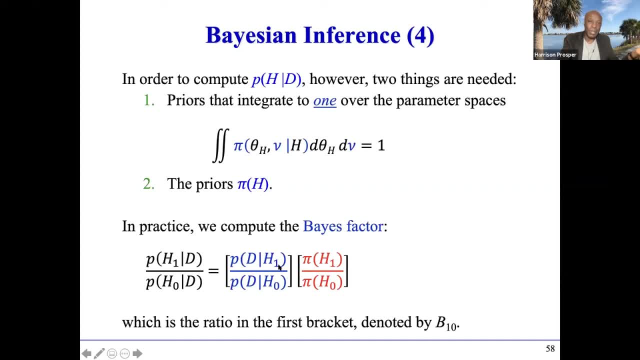 given the data, And this is simply equal to these two ratios. It's the ratio of these things and this is called a Bayes factor. And remember, probability of D, given H1, you've already done the integration over the parameters of the hypothesis H1. 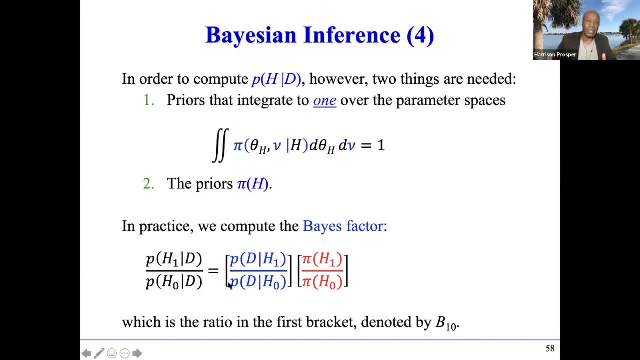 Likewise, here you've done the integration of the hypothesis, of hypothesis H0. And for this ratio to be meaningful it is necessary that this integral integrates to one, which means of course you cannot have probabilities here that integrate to infinity. That would not be, that would not work. 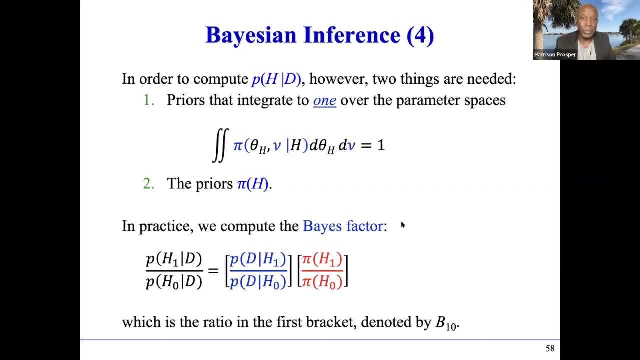 So that's one of the things that's important and that's difficult to achieve. And finally, there's this ratio here which is ratio of the priors that you specify for the different hypotheses or different theories. right? So maybe pi of H1 is the priors of H0,. 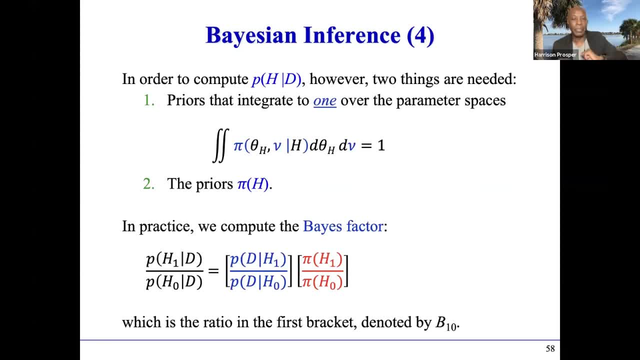 which is the priors of H1, right, And maybe you have a number of priors that you'd like to assign to the NMSSM and perhaps priors of H0 is what you want to assign to the Thurman model. okay, 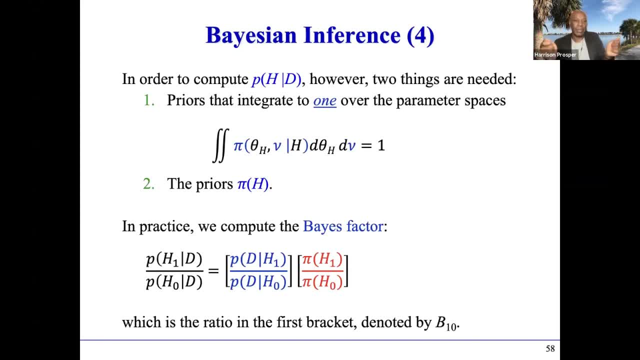 And different people will have different numbers for these, And so what people do is that they ignore this because it's controversial, the red part here, and they only consider the Bayes factor, And the reason is the following: is that the Bayes factor, this ratio here, tells you: 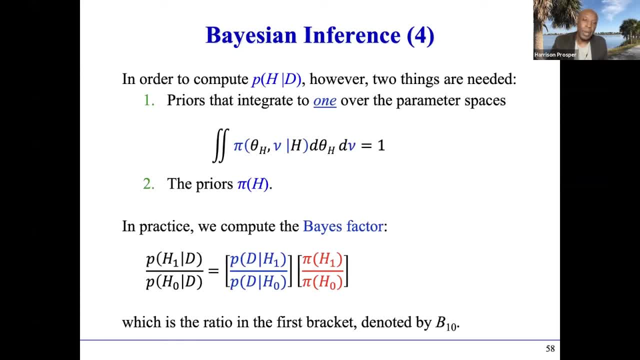 by how much the, The prior odds. so this ratio here in red is called the prior odds. you know, 10 to one like betting And I bet that the you know the NMSSM is, you know is preferred relative to something, some other theory. 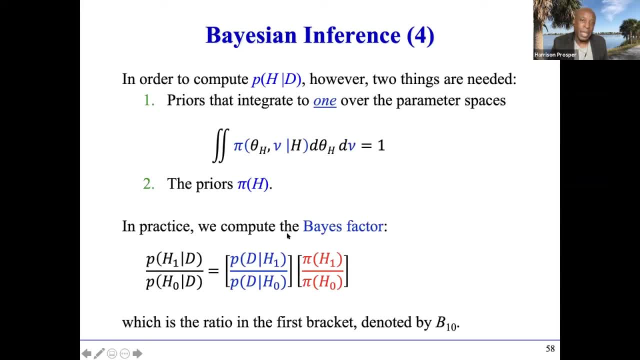 and this is called the prior odds that you specify, And so this Bayes factor tells you by how much the data changes the prior odds to the posterior odds. right, That's what this thing does, Okay, so in the last five minutes, 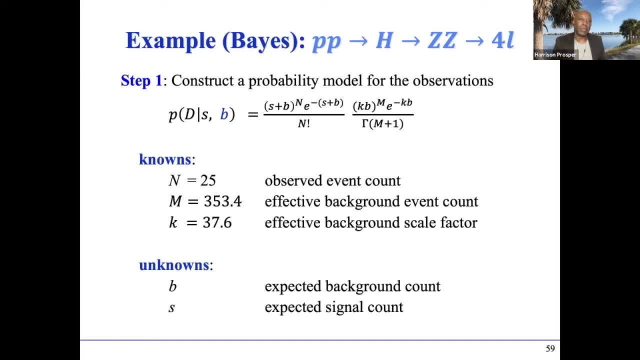 let's just apply this to our example. So remember, this is the likelihood. there's two pieces and these were the data We observed: 25 events, an effective background count of 53 events, and so on. So let's just plug away. 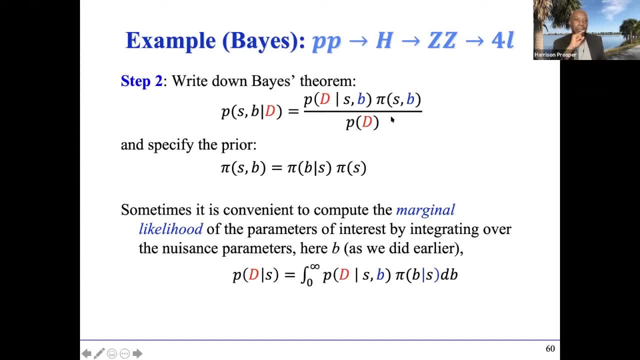 So step two: we write down Bayes' theorem And then we're going to specify the prior. So here I'm factorizing the prior into two pieces. I'm allowed to do that. I could factorize it in different ways. 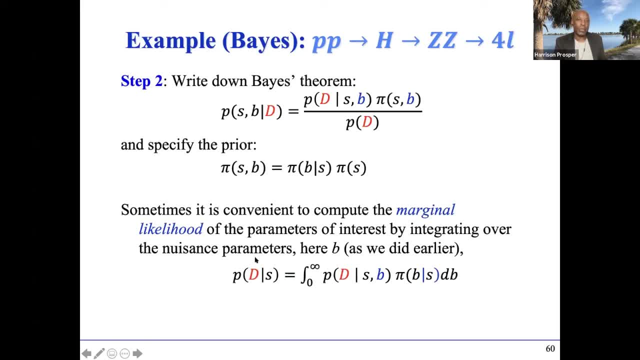 but this is perfectly okay, And what I'm going to do now is I'm going to integrate. I'm going to integrate this with respect to the background mean, just for convenience. So now I arrive at the probability of data, given the signal. 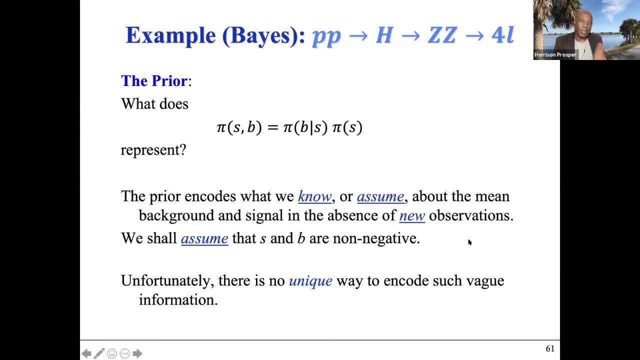 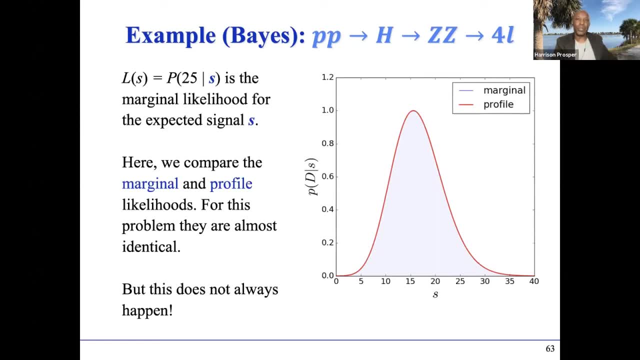 Now I'm going to- I'm not going to- dwell on the prior cause. I think this is, this is complicated. Let me just cut to the chase. So if you, if you go through this calculation right, That is you, you, you, you simply compute the integration. 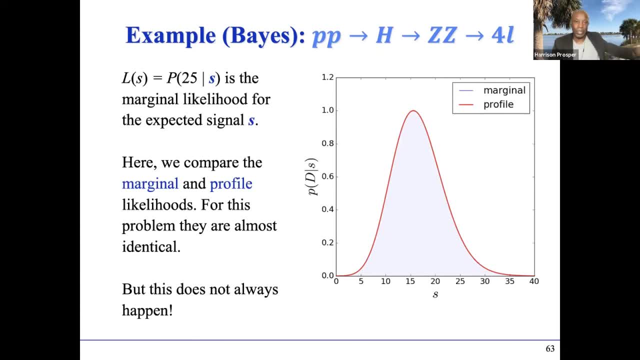 with respect to background, with some choosing some prior, which I've chosen to be in a very, in a very sort of simple minded fashion. Then you arrive at. you arrive at something that is the analog of. you arrive at something that is the analog of. 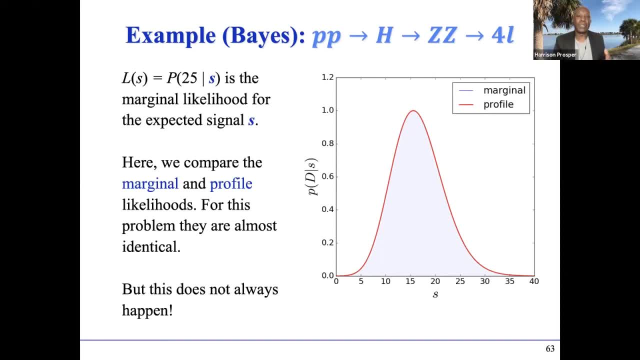 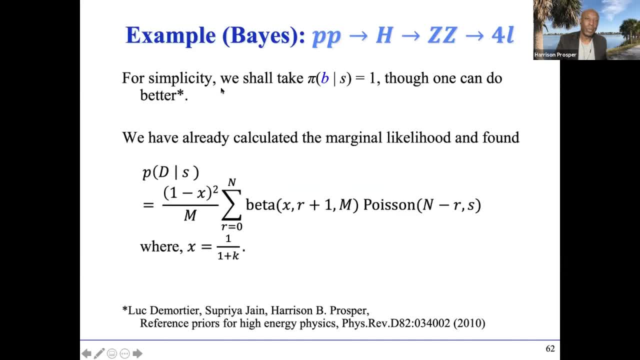 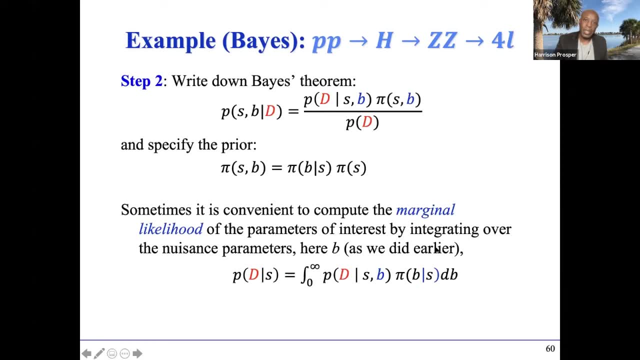 the count of 25, rather given the signal Again, just just to let you know what. what have we done? We've done this integral here. Okay, It's this In principle. this prior should be something that's. 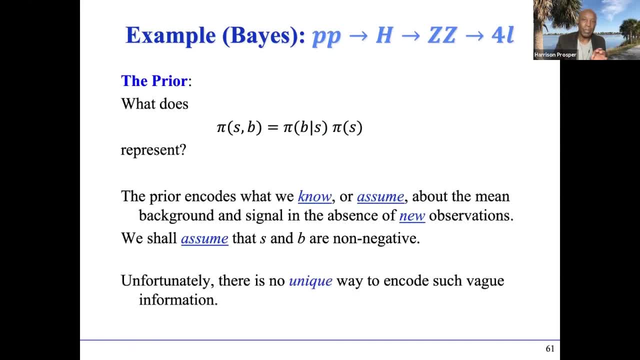 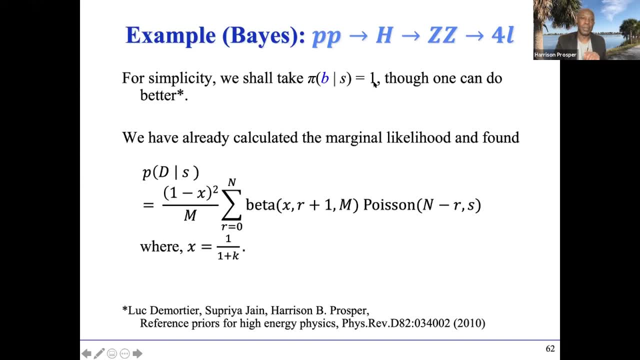 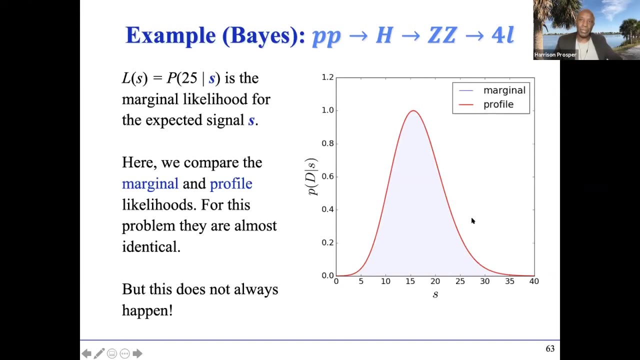 meaningful in practice for this particular problem. I'm going to put something that is not terribly meaningful, and we'll set this equal to one, But if you do so, what is remarkable is that you find that the integrated likelihood, the marginal likelihood, has exactly the same shape. 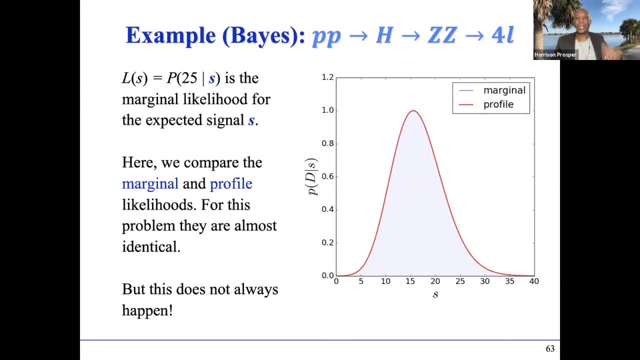 interestingly enough, as a profile. In fact, when I first saw this, I was actually surprised, And so I would love if one of the students who's listening would actually check that this is really true, Cause I expected to see some difference between the two. 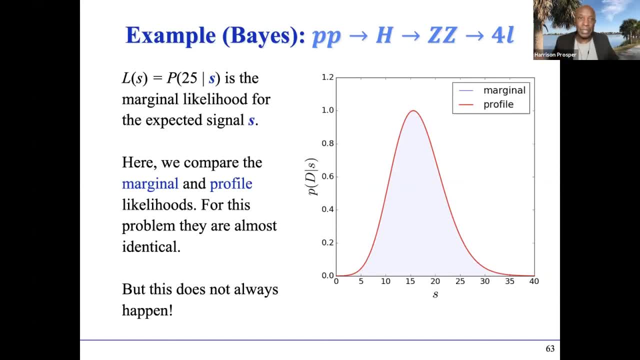 but in fact they seem to be identical, but they are different things, different beasts entirely. One, basically, is built on the frequentist interpretation of probability and the other one based on the, on the, on the degree of belief. And so, even though they identical in mathematical form, 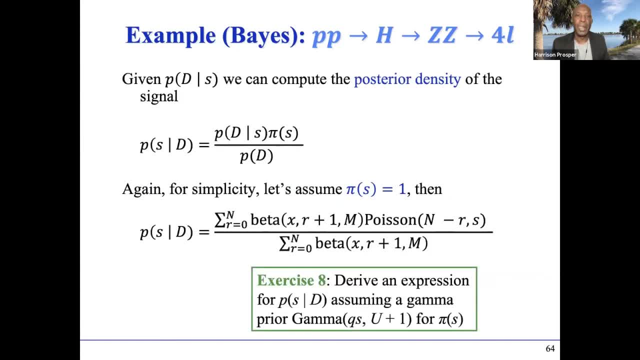 they have very different interpretations. Okay, So. so, now that we have the probability of data given the signal, I can plug in here a private signal, The private signal which again is controversial. That's difficult, And here I'm setting it equal to something again. 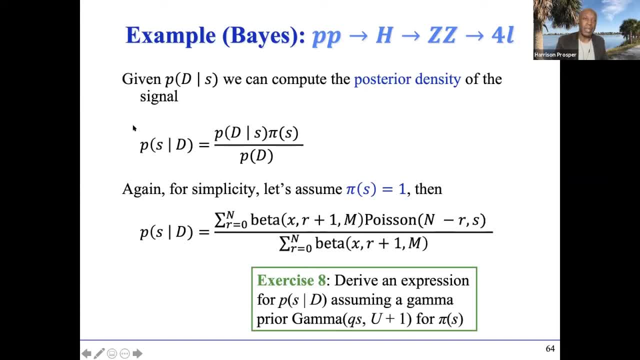 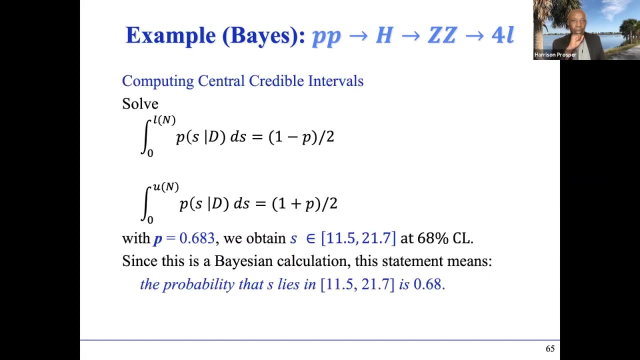 that's not terribly meaningful, but you can then in fact arrive at, finally, the probability of the signal given the data, And that's equivalent to, again, ultimately, the, the, the profile likelihood. Okay, So we now have some curve. that summarizes the inference. 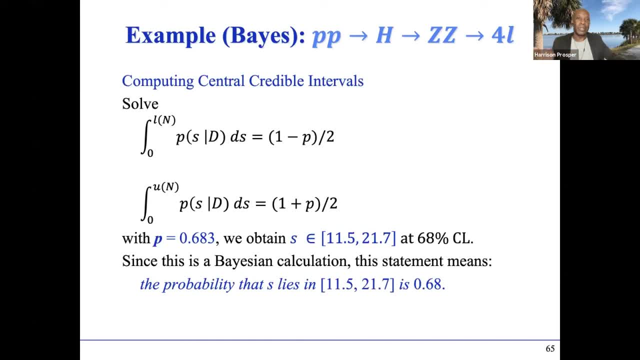 the probability of the signal. given the data, How do I, how do I quantify the accuracy of my inference? Well, here it is. One can simply construct an, a lower bound, an upper bound, by solving these equations. That's equivalent to exactly what Neyman did. 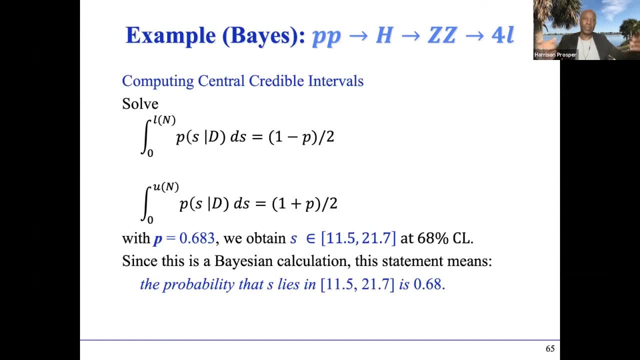 in the frequentist approach way back in 1937. That's just the Bayesian equivalent of the same. And when, if one solves these equations, one finds that the the statement now is that the mean signal is lies within 11.5 and 2.7 at 68% credible level. 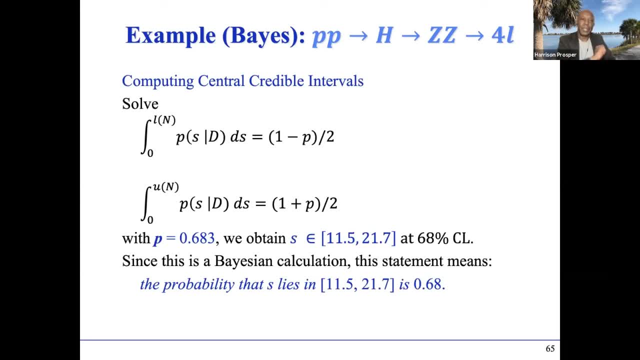 But here is the kicker: This is a Bayesian calculation. Therefore, this statement simply means directly that the degree of belief in that assertion for the signal S lives in that interval. the degree of belief in that signal is greater than the actualражion greater than the actual. 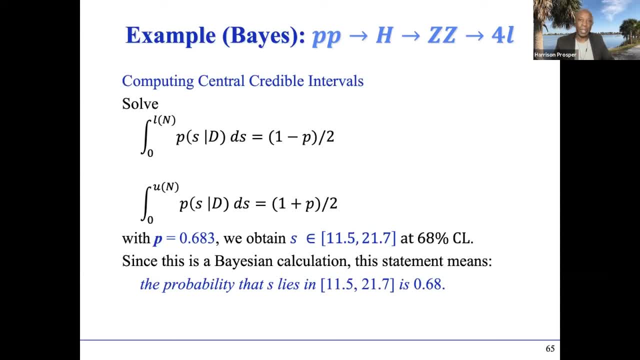 belief is 0.68.. That's it, Nothing more than that. It does not have a relative frequency interpretation, And that's the very big difference. Now, of course, nothing prevents you from doing these calculations, getting an interval, because after all, these intervals depends. 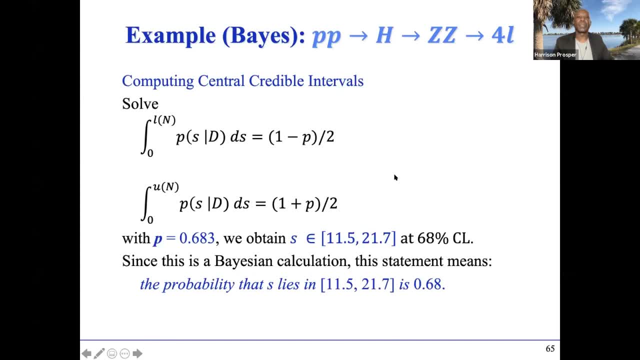 on the data: n, right The datum in this case. Nothing prevents you from using the Bayesian approach to construct intervals And then, on a computer, counting how often they contain the true value. So you run a simulation on a computer where you have a true value. you. 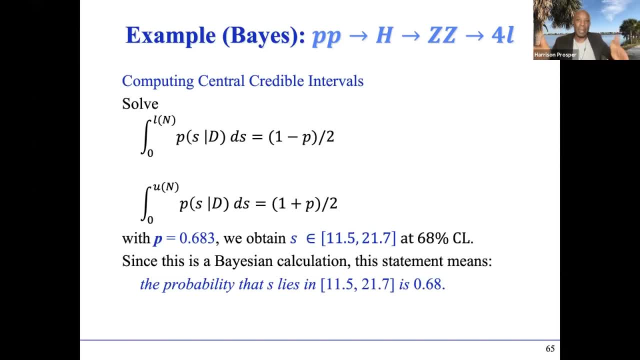 run the simulation and you can simply count. how often do the Bayesian intervals- credible intervals, as they're called- how often do they contain the true value? And, of course, what you would hope is that, roughly speaking, on the average, that probability would be roughly equal to 68%. It doesn't have to be exactly, because 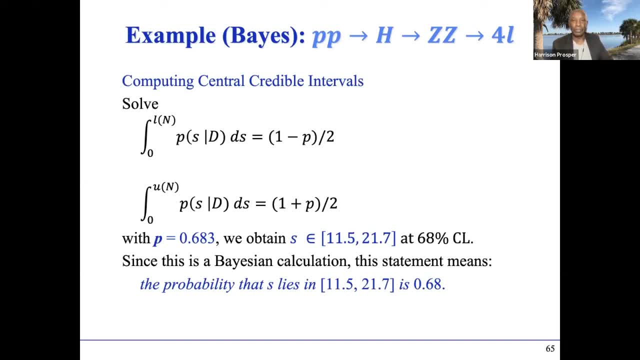 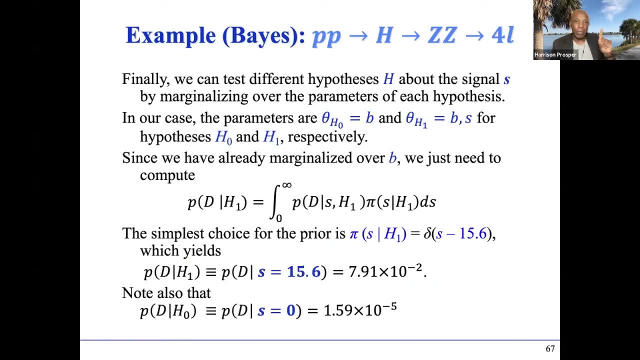 it's not designed to be exact with that, But that's what one would hope. And in the last, if I have one more minute, we can also go further, And here we can compute the probabilities, probability of H1 and so on, And these are: 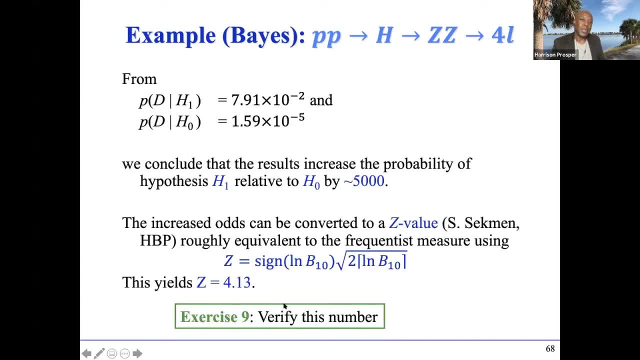 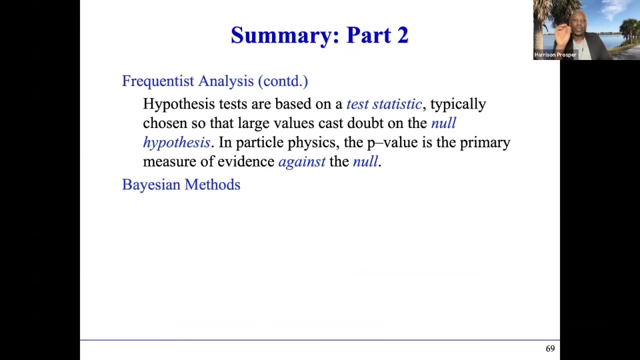 they, And when you actually go for this whole calculation, remarkably you arrive at a relative probability of those two hypotheses. that's essentially identical to the frequentist approach. But I should warn you that it is not always the case that a Bayesian approach to an analysis gives you the same answers as a frequentist approach. 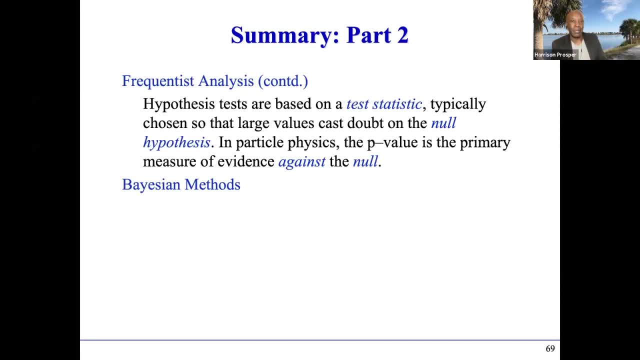 In this particular case, they turn out to be essentially the same, But in general they are different, And when they are different, that's typically a sign that your conclusions are not robust, And that's an important point to bear in mind. 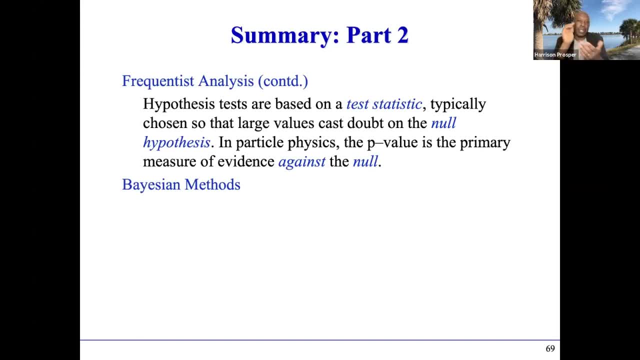 OK, so let's just summarize. So to test a hypothesis, you have to construct a test statistic, And we've noted that you can use the same one, The likelihood ratio, or rather negative twice Log of the likelihood ratio, as was used to obtain an interval on upper limit. 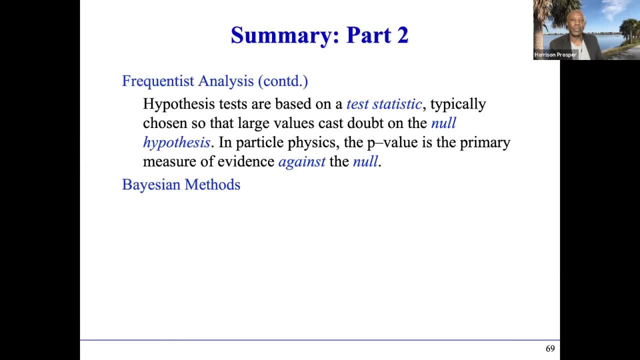 And that can be used to test different hypotheses for the signal. In Bayesian approach, Bayesian theorem is the primary tool that's used for inference for everything. Unlike the case in the frequentist approach, you can get rid of nuisance parameters by integrating them. 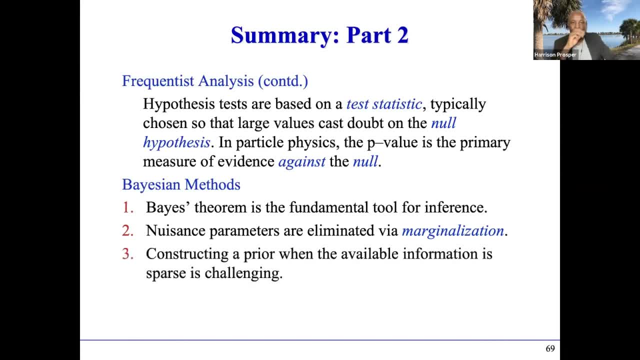 And you can get rid of the problem marginalization. But as we've seen, as I've hinted at building a prior when the magnification you have is rather sparse, a prior that people would find non-controversial is quite challenging. 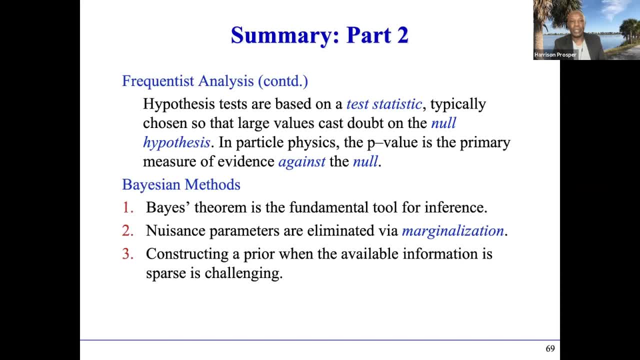 And that is, of course, one of the reasons why I think that in our field we tend to prefer the frequentist approach, because it completely bypasses the need to construct a problem. So we need to be more careful about the use of the prior. 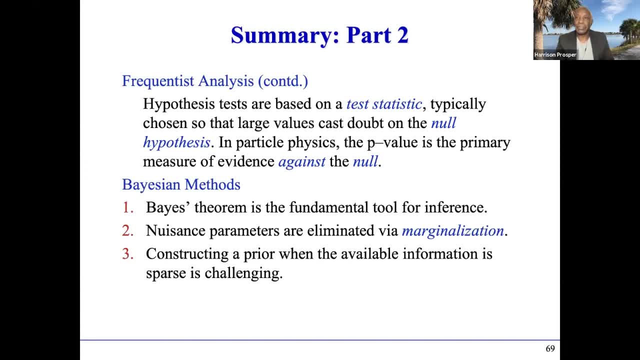 Okay, and that brings me to the end, So questions. Thank you very much, Harrison, for this wonderful set of lectures, Very, very useful. We have some questions. I think I will read from chat first. So Artna is asking: how does one decide which approach to be used, frequentist or Bayesian? 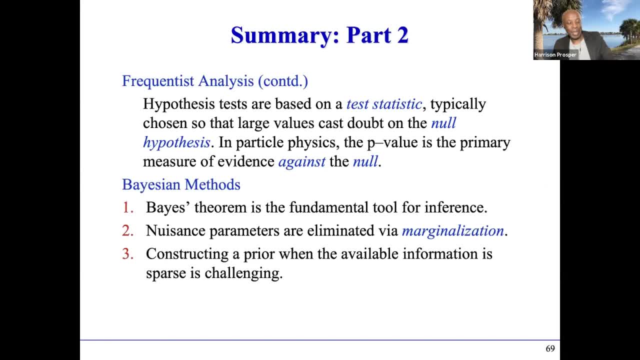 Yeah. so that's an excellent question And, as you can imagine, the one I get asked quite often. So here's my answer. My answer is this: is that I think that when you arrive, when you try to understand how to do an analysis, 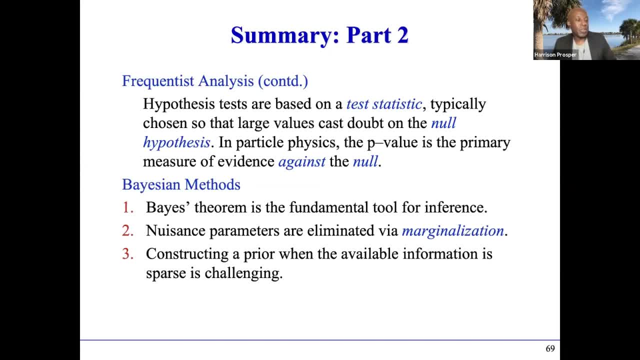 analyze some data. what I usually find is that thinking about a problem in a Bayesian way is a good way to clarify your thoughts. right, It's a good way to frame the problem and clarify your thoughts. I'll give you a few examples. 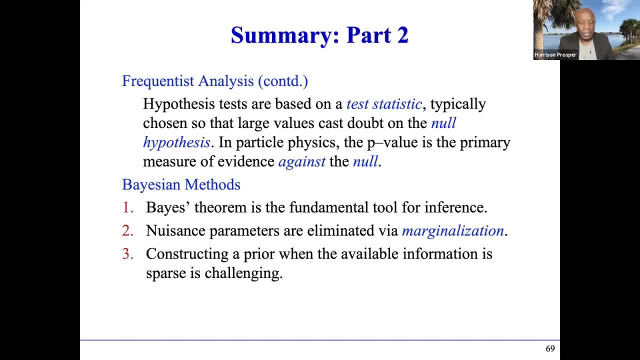 I'll give you a few examples. I'll give you I hinted at an example of this. So you may all know that for many, many years there was this not very good an ad hoc way to account for the uncertainty in positive distribution functions right. 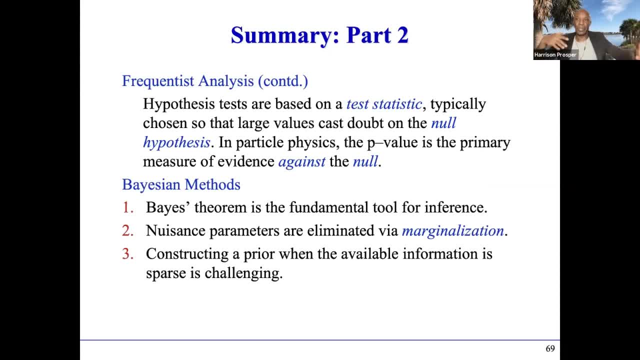 We were told: try lots of different groups, different PDFs and make an envelope of the results. That was the procedure that we were told to follow, Of course completely ad hoc, not based on any principle whatsoever and essentially having no statistical foundation. 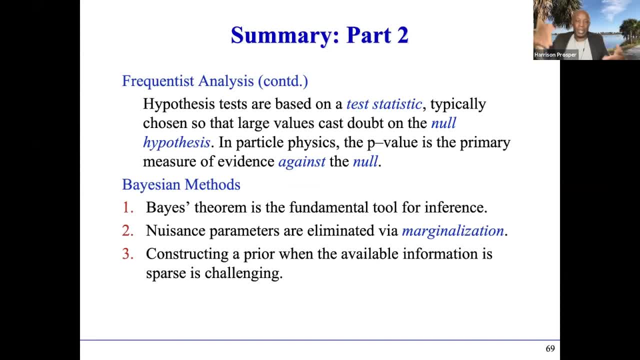 And why? Because we were thinking about this in the frequentist way, and so we're just using the seat of our pants to arrive at that particular procedure. But if we had thought about the problem in a Bayesian way, then the answer is obvious. 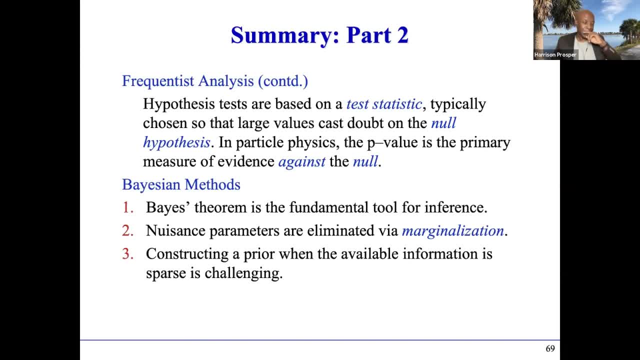 The answer is that you build a model In which not only do you have continuous parameters, either parameters of each PDF first set- but you also have the discrete parameters: NNPDF, CTEC, MMHT, etc. These are discrete parameters. 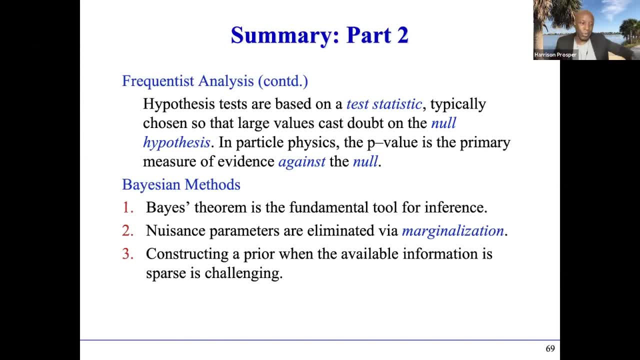 And then you integrate over the Bayesian prototypes, you integrate over all the parameters of the different PDF sets And then you arrive at something that only depends now on the discrete parameters NNPDF, CTEC versus MMHT. And when you go for the reasoning, it becomes obvious what one has to do. 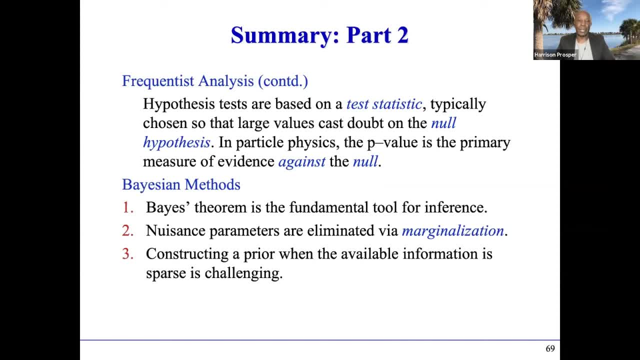 And indeed subsequent to you know, later the LHC PDF groups retooled their recommendation And in part inspired by the Bayesian sort of reasoning. So what I would say is that when you're stuck, think Bayesian The problem in the Bayesian way. when you've come unstuck, you can then go back to doing a frequencies calculation. 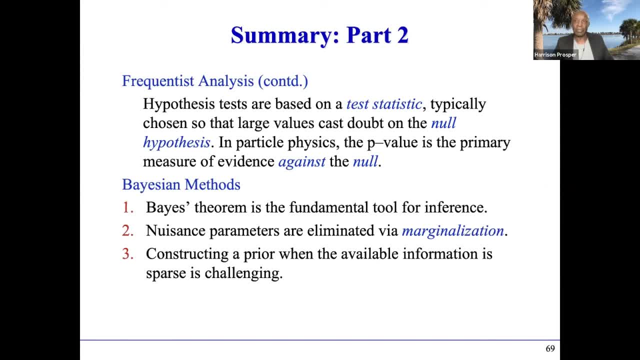 That's what I would suggest. Okay, so one should think about it like really problem-based and go step by step. So on this similar topic, Sanjay had a question that: is there any place where one should absolutely use the Bayesian approach? 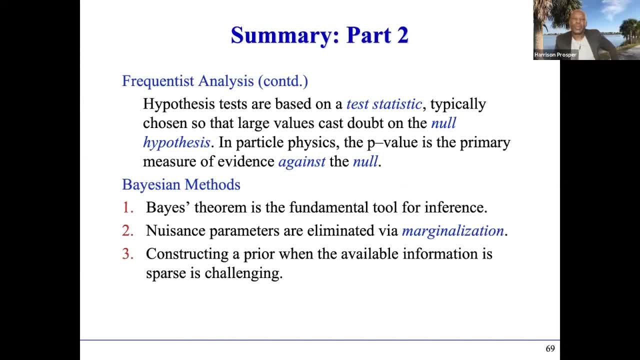 Or one should have used not the frequent dispersion Sure. So our theory colleagues, of which there are many at this wonderful workshop, they do calculations in which there are artifacts. in those calculations, right, There are things such as the binarization scale, the factorization scale. 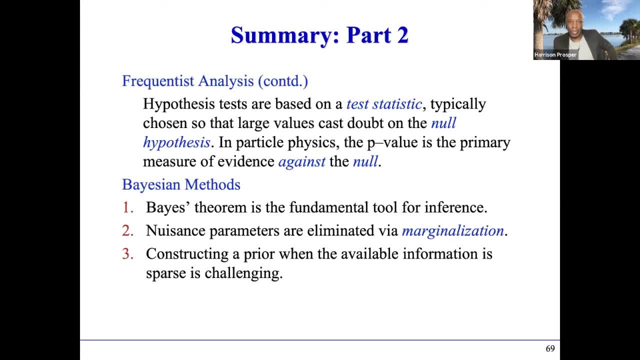 These are all artifacts of the calculation, because these are approximate computations, Suppose I wanted to take, Take into account in a formal way, take into account the uncertainty arising from the factorization scale and the regularization scales in the calculation. You could do it in a frequentist way, but only in a way that's sort of artificial. 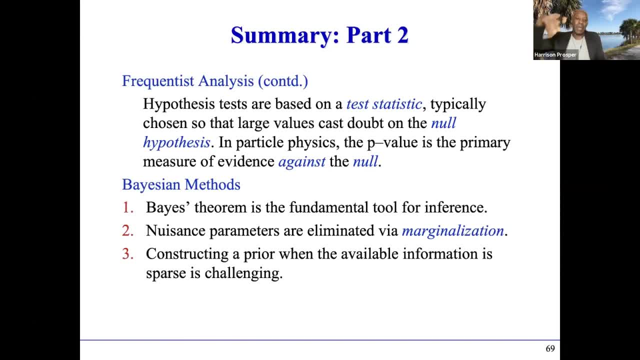 You could say: let me pretend that I embed my calculation in a universe in which I imagine that I can, I have, I can Multi-frequencies for different choices of the scales and then do frequency calculation. But that's stretching the frequentist principle to an absurdity. 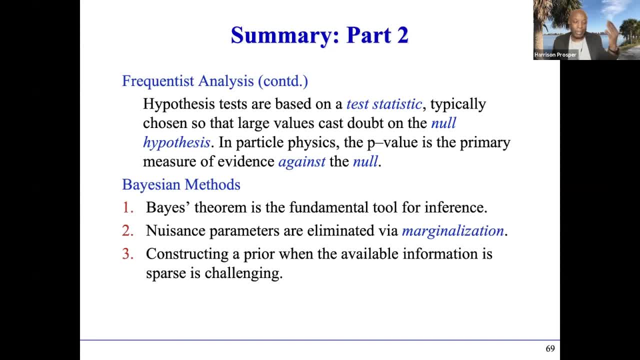 Whereas if I think about it in a Bayesian way, well, I can just simply lock my theory colleagues into a room and tell them: you are not allowed to leave this room until you tell me what your prior distribution is for these parameters. I don't care what it is. 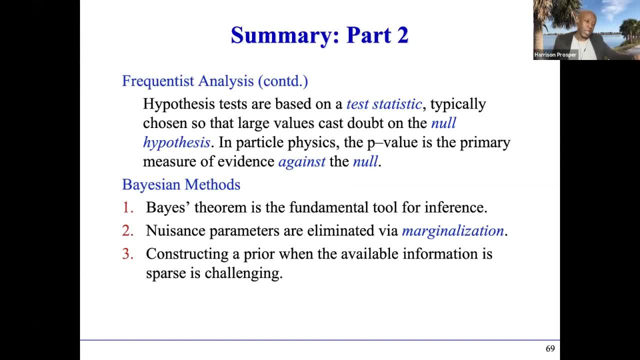 I don't. All I want is I want your honest opinion, You know. should I increase the scale to a factor of 10 times larger than the nominal scale? Should I decrease it by a factor of 10?? Is there a preferred value? 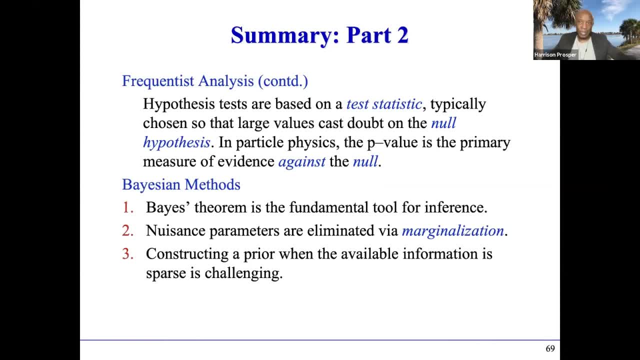 I don't care what it is that you tell me, but I want you to sit down and think hard about your problem and come back and say: this is the shape of my prior probability for these artifacts of my calculation. Once I have that, 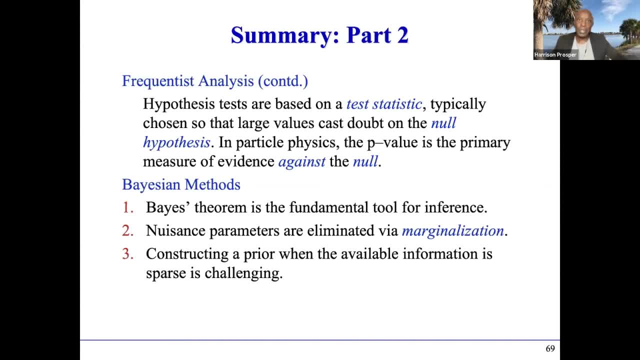 Once I have that, the Bayesian approach tells you exactly how to use it Right. And so here's a case where we could do it: if we could chain our theoretical colleagues into a room and give them no water, no food until they tell us what they think this parameter. 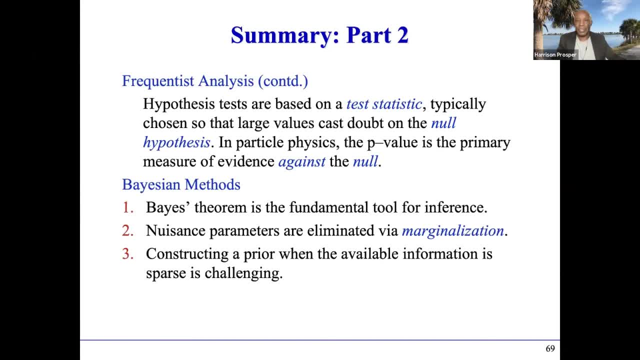 What's the spread of those parameters? Once they give us this function, it can be used formally. So here's one very concrete place where that could be done And in fact, in one of my analyses I essentially just did something like that, except, of course, the usual sort of thing where you increase things by a factor of two, decrease things by a factor of two, or you know, the usual sort of thing that we all do. 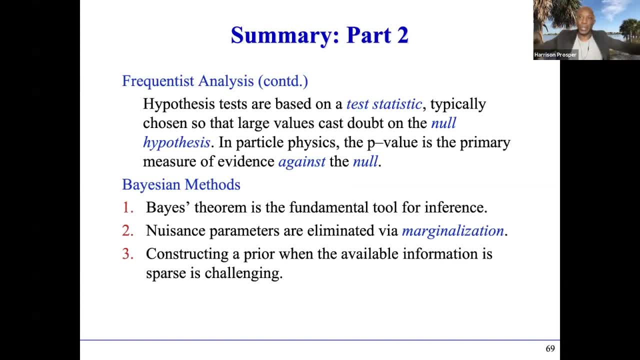 But instead what I did was I simply summed over the different likelihoods with all the different combinations, which is kind of a rough marginalization over those parameters. Dhrubanshu, can you unmute and ask Yes, Okay, Can you ask your question? 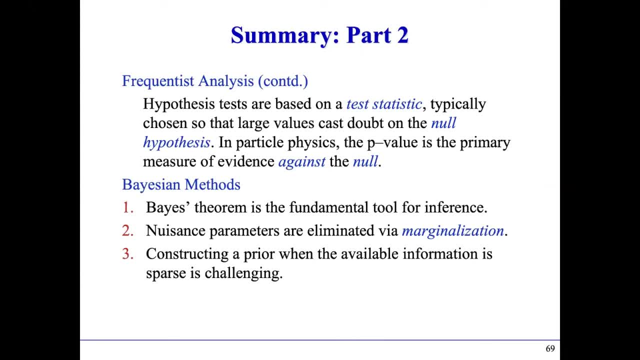 I see your hand raised So I probably would have missed this thing. So this is related to the prior probabilities. So is there a particular algorithm or a strategy by which we can choose a particular prior distribution to continue with the Bayesian approach? Yes, 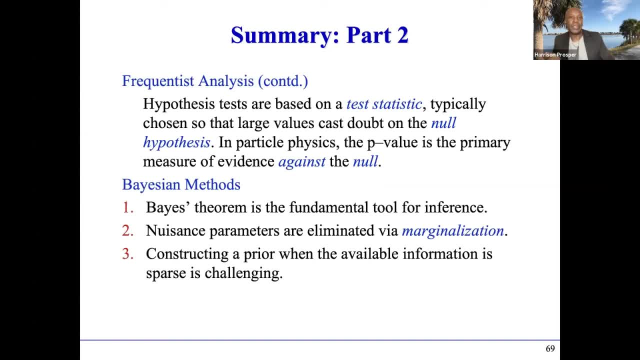 Yes, So I mean, as you can imagine, there's been a huge amount of work by statisticians over the decades, right on prior. Because this is you know, because you can't proceed unless this problem, Because this is you know, because you can't proceed unless this problem is solved. 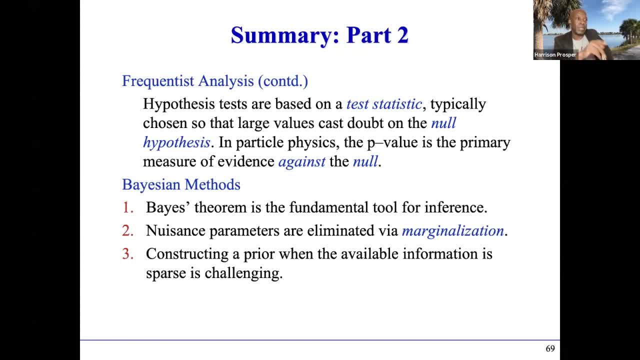 And the problem of simply setting everything equal to one is that it's essentially inconsistent, right? I mean, you get reasonable results most of the time, but still, strictly speaking, it's inconsistent. So there are techniques. One of the requirements is that you know a probability is like a probability distribution function is a bit like a vector in that it is an invariant object. 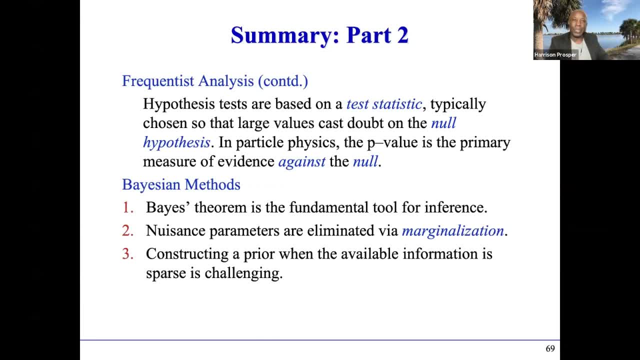 And it should not And depend on how it is parameterized. So, for example, if I build a probability distribution to describe some Suzy model, right, and in that probability distribution there's a tan beta, it shouldn't matter if I simply change my mind one day and say, oh, you know what, I prefer to write it as log tan beta. 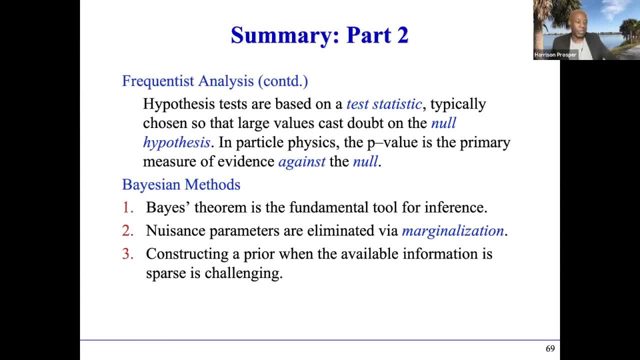 That should be completely relevant to the probability distribution And so, given that mathematical requirement for probability distribution, You can actually prove that there's a certain prior that arises that is invariant. that would actually respect this requirement that probability should not depend on how it is parameterized. 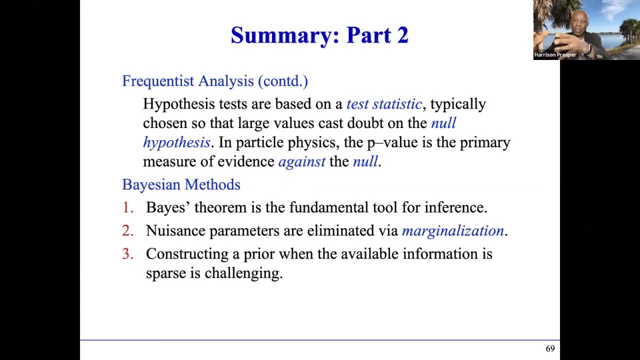 Many different arguments lead to the same conclusion, And that prior is called the Jeffreys prior. Okay, that's the good news. The good news is that you arrive at that prior. The bad news is that when that prior is used for problems in multiple devices, 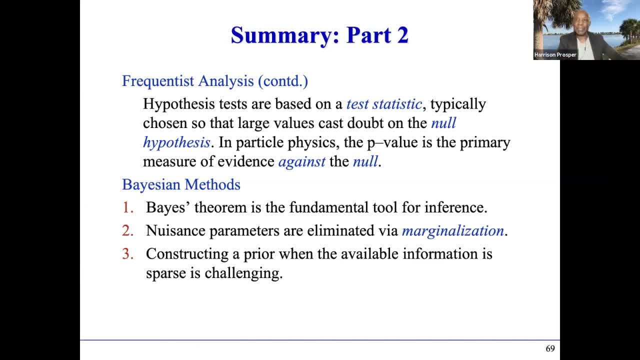 Dimensions, you often get horrible results. And so what people have done? they've sort of stepped back and said, okay, well, this is not good, And then they use all kinds of different arguments to arrive at priors that give reasonable results. 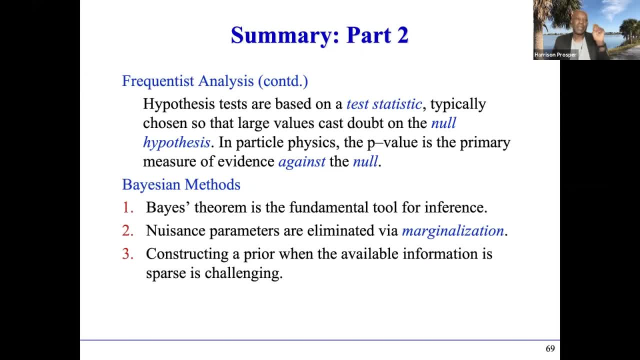 But I have a different take. My take is that the arguments that lead to the Jeffreys prior are sound, mathematically sound, And since there are several different arguments That lead to the same conclusion, there's some truth to that. 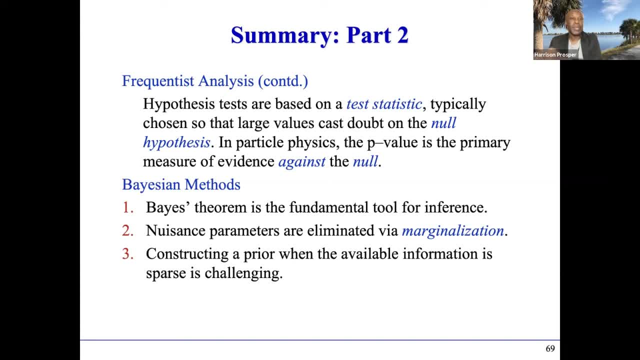 There's something about that prior that is actually sound. The fact that it needs two horrible results tells you there's something missing, Right? There's an extra thing that one has to put in to make the result sensible, And I don't have time to go into that. 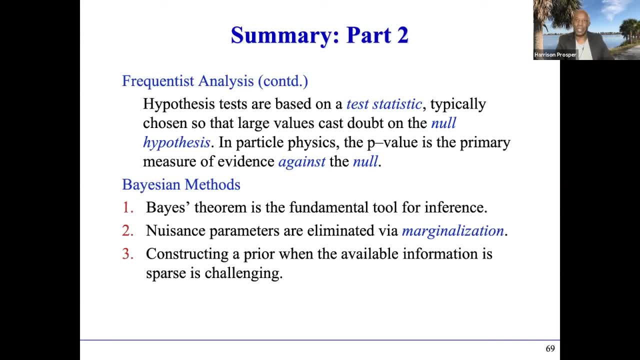 But the point is that you can actually put extra things into it to make it sensible. In fact, the most beautiful reasoning for the Jeffreys prior Is that Is that it is the prior that assigns equal weight to every probability in the space of probabilities. 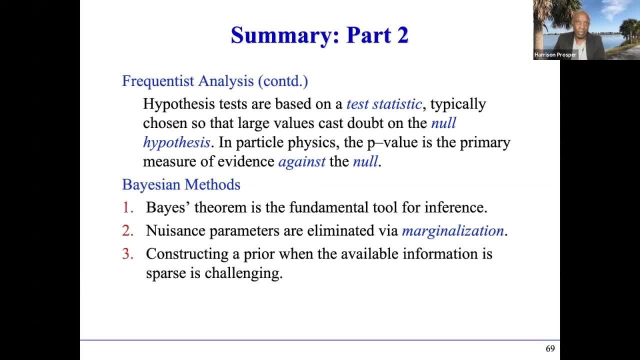 rather than equal weight in the space of parameters, which is not invariant. But that will take me too far afield, So we have a couple of more questions, if you are okay, to take them. Absolutely yes, Arun. Yeah, I had a question related to the frequentist method. 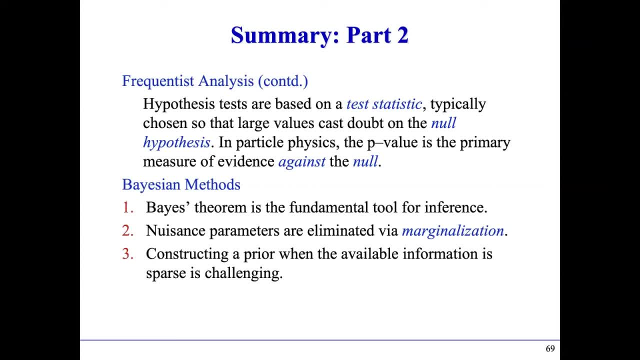 So we take this profile likelihood ratio by the test statistics And we take the In the denominator. we are using the likelihood of S hat. So why do we use that instead of say like a likelihood of S equal to zero? 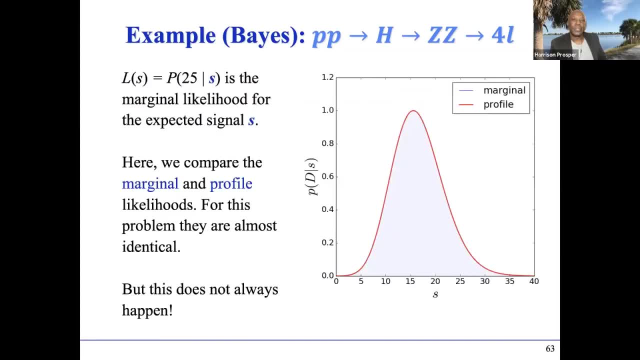 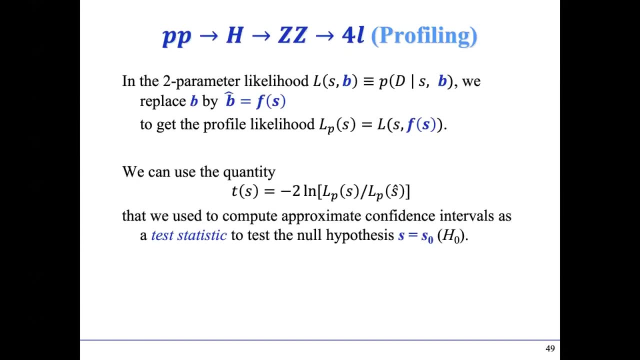 Is there any advantage in that? Okay, So let me go back to that. I think it's easier to show it. Yeah, So here The point is that One way to think about this. Okay, So let's think about this a little bit more. 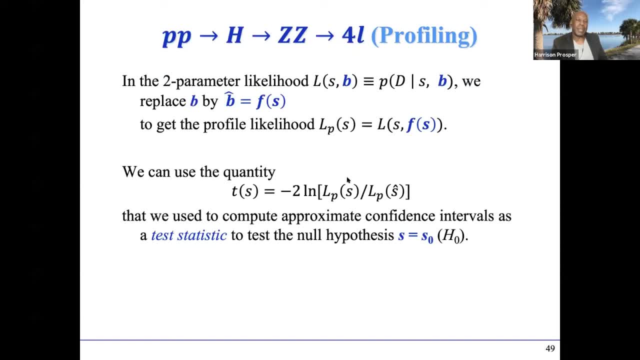 One way to think about this ratio is that you're comparing. Again, this is very, very loose. I'm speaking very loosely here because you know we're physicists, so that's okay. One way to think about it is that this is comparing the best fit hypothesis to the signal. 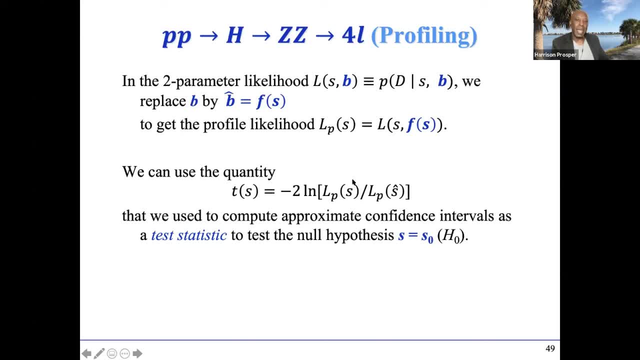 that's S hat, with the hypothesis for S equal to some other number, right? So you? You're in some sense comparing the likelihoods of two hypotheses, S and S hat. So S hat is the best fit hypothesis. 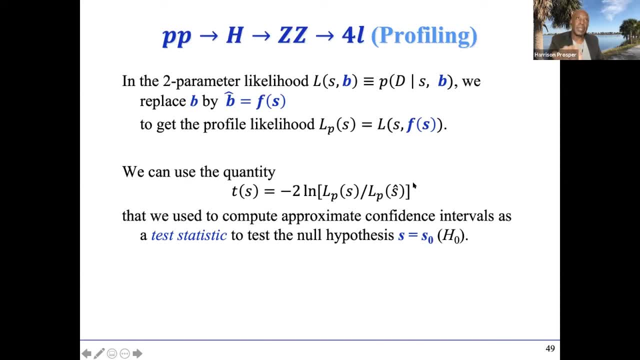 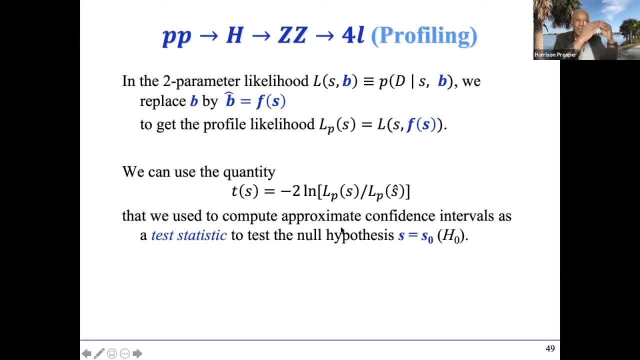 that if you- And you should really do it- You should really write a little program and convince yourself that's true, that if you, If you generate random numbers, you know, if you literally start off with this likelihood, I showed you and you choose values of S and B, right, true signal, true background, you. 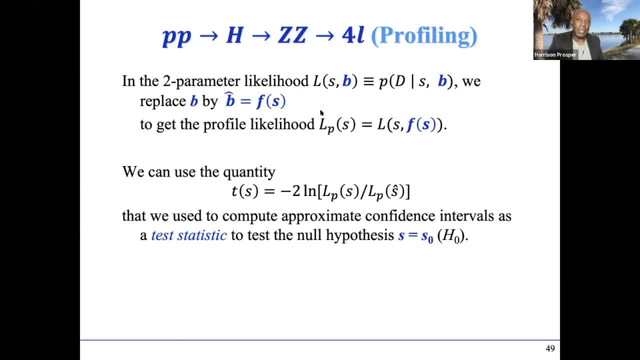 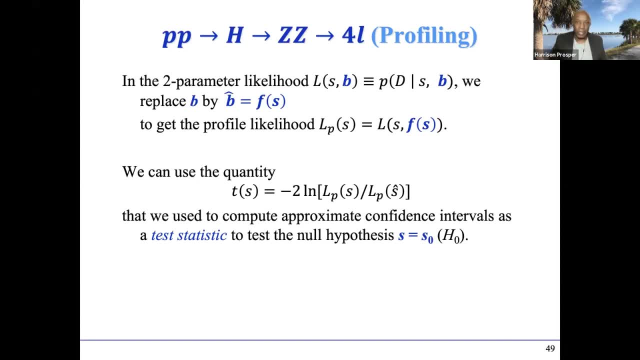 T holds that of a chi-squared distribution, which means that that distribution of T does not depend on S and does not depend on B, right Neither of these quantities, And so that is why this is done. You can choose different things. 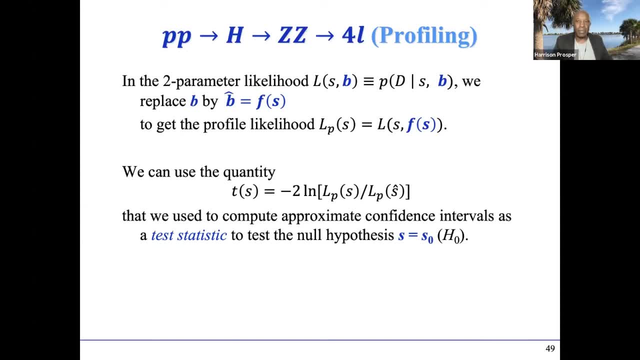 And in fact I recommend that you read this paper by Kyle Kranmer and company, because they make different choices and what they show is that different choices lead to different probability distributions other than a chi-square. but in this simple case where, if you really follow the recipe, you find the profile likelihood you find the best fit, 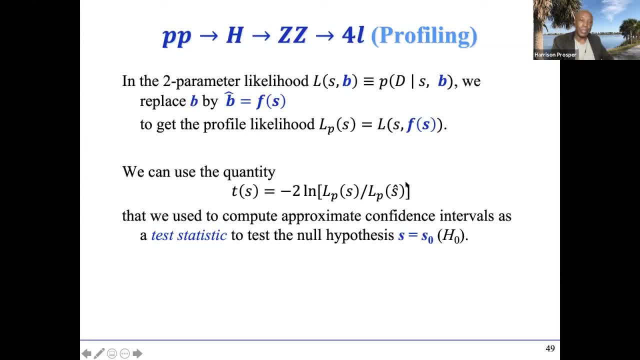 value for the signal, and then this quantity absolutely looks like a chi-square density when you simulate it, and this is true even for relatively small counts. This is what I find amazing: is that even if you do this for relatively small counts, this really has a 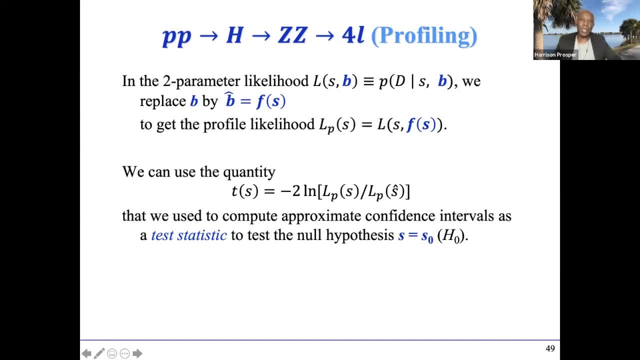 category distribution. Why is that a good thing? Well, it's a good thing because then you know what the distribution of t is, which means you don't have to simulate it. and secondly, since you know what the distribution of t is, you can calculate p-values and a whole bunch of other. 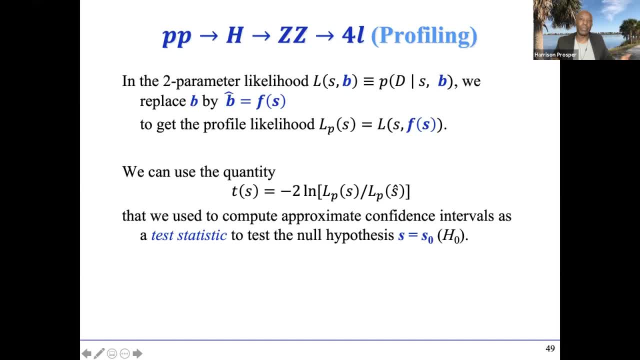 things. You can find limits and intervals and what have you. So you could choose a different number here, that's for sure, and that is done in this paper that I referenced. but then you have to work out what then the distribution would be, given that. 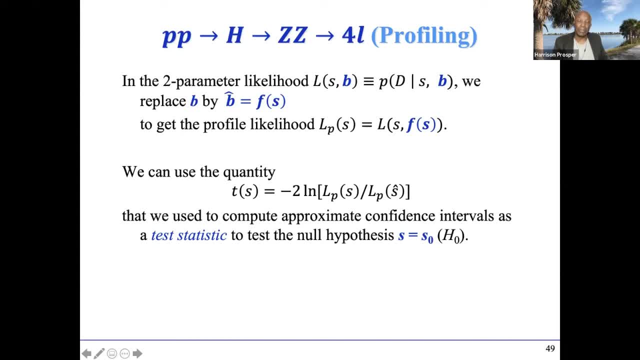 choice. So it's really because of that theorem. that's why it's done. Thank you, Shabtiki. Can I please unmute and ask your question? Hello, can you hear me? I can. yes, please go ahead, Shabtiki. 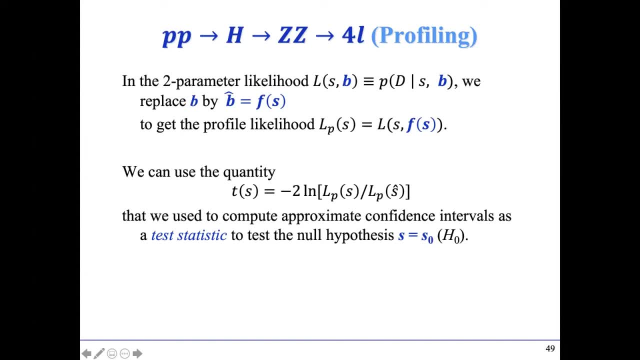 Yeah, Hi Harrison, Thanks for the great two lectures. I have two questions, one on the frequentist and the other one on Bayesian. So the priors are in some sense non-objective And you know, I think that's a good question. I think that's a good question. 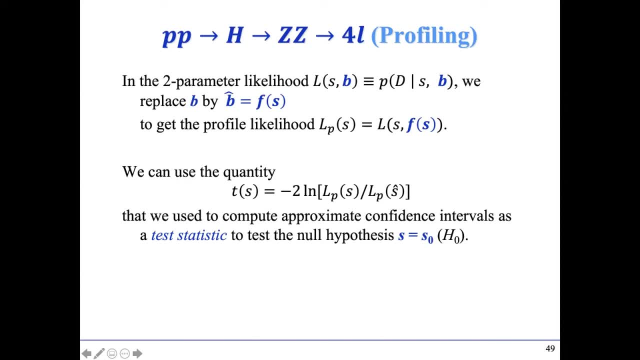 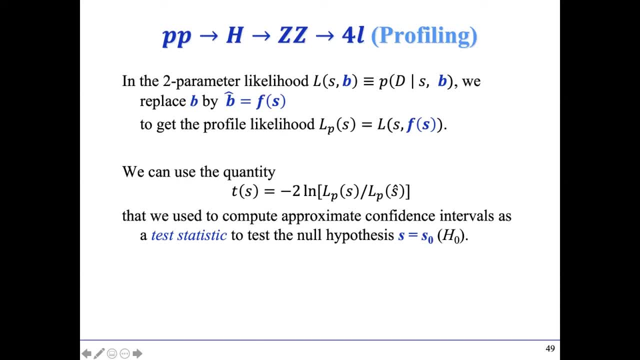 SUSY parameters and another person who does know about previous experiments having put limits on the SUSY parameter space. So they would construct. is it natural that they would construct two different priors to look at the same data? Yes, And if yeah, so if that's the 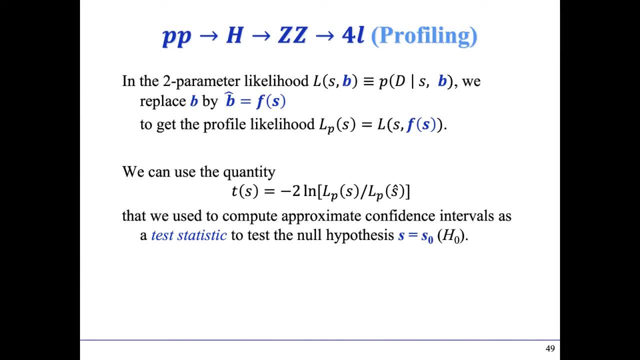 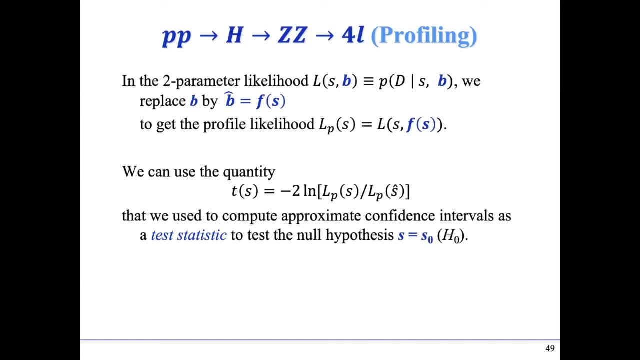 But the two experimenters should converge at the same conclusion. Yes, that is correct. Yes, So it can be shown again with certain conditions and so on. it can be shown that, indeed, as you have more and more data, the likelihood becomes sharper and sharper. 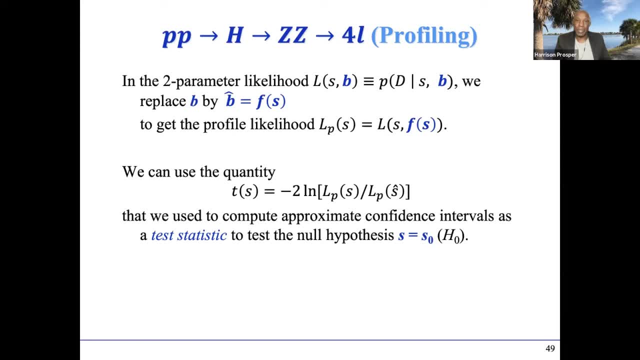 and sharper And therefore the effect of the prior basically disappears. So really the problem of the prior is really the problem of the prior occurs when the amount of data you have is really rather few, right when you have very few counts. 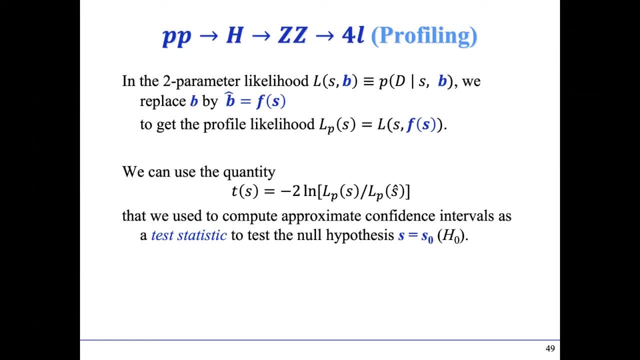 and so on. That's when you have most influence on the prior, But you're absolutely right that that effect disappears as you get more and more data. But let me make a point, though, about the you know. so this is a problem. Some people think this is a problem, But the reason why people 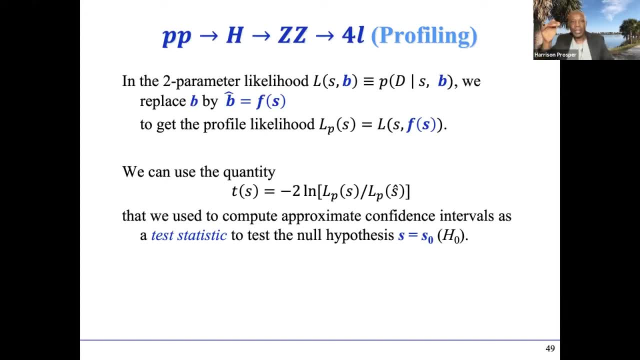 think it's a problem is because they mistakenly think that there is quote, unquote, the answer right, And I've been trying to emphasize repeatedly that this is not physics, this is mathematics And if you make different assumptions, you'll get different answers from the same data. 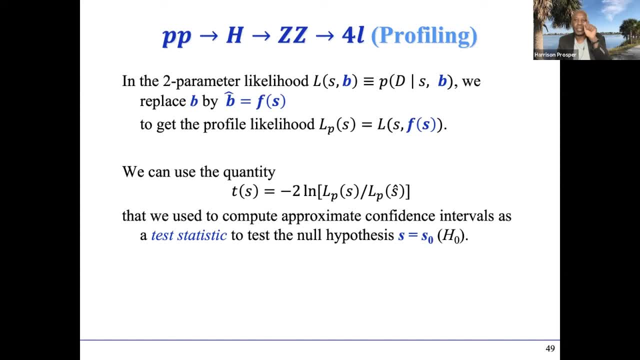 Same thing is true in the frequentist approach. If Sharma chooses a different statistic than I do, using the same data will have different results, And that's normal right, And so the fact that the same data can lead to different. you know conclusions. you know they may be consistent with each other, but they're different. 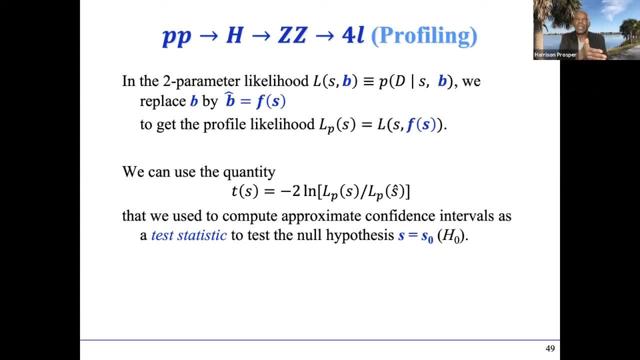 it's not a problem, And one thing is: it's inevitable because the data are consistent with lots of different conclusions within some distribution, So it's not surprising that you can arrive at different results. In fact, this is striking, Just as if 10 people analyze the same. 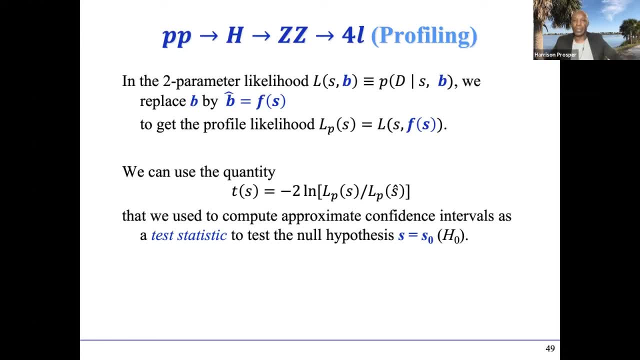 data and do different optimizations and so on, they will arrive at 10 different results. Nothing strange about it. So I think that this fact that there's not a unique answer is intrinsic to inference, But the good news is that as we get more and more data in both approaches- 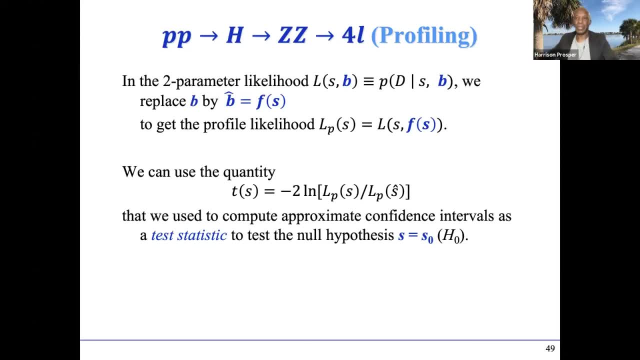 the effect of these differences disappear In general, not always, but in general. Right, Yeah, thanks, Yeah, so yeah, absolutely. It's natural that the same set of data can lead to, depending on the amount of data, also can lead to different conclusions with yeah And then. 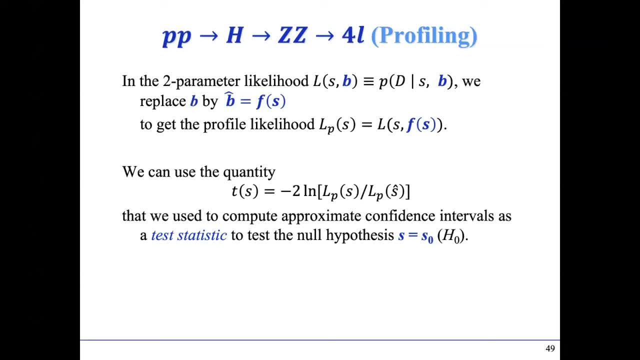 but eventually, with, with increasing data, all of those should, should converge And I guess if, even if one constructs a toy experiment with increasing data, one should be able to see that that absolutely even, yeah, even if I start with different priors. 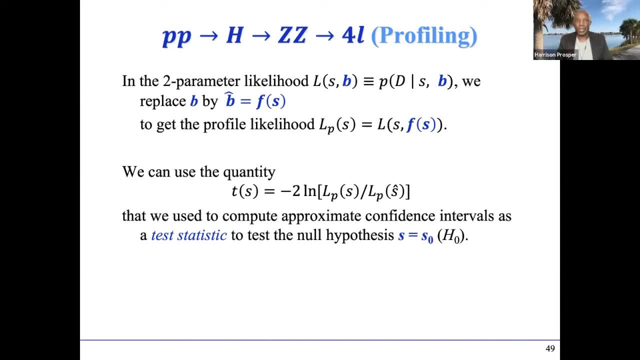 Absolutely, And in fact, this is also true of likelihoods, right? So if you, if you, if I, have an example somewhere where you begin with a likelihood that's very, that's very non-Gamson is really has a strange shape And, of course, 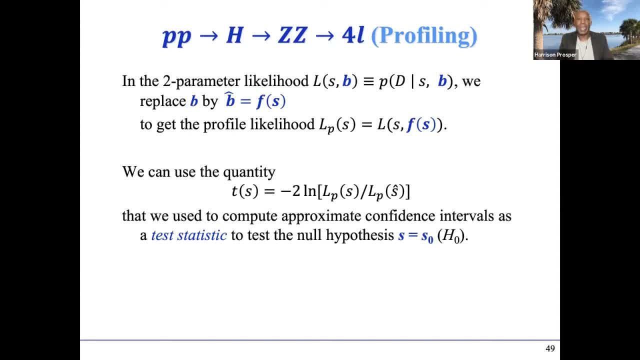 for those likelihoods. none of none of the theory works, But as you as, but you can show, as you add more and more data, these strange distortions in the likelihood disappear and the thing becomes more and more Gaussian Right. But here's the problem though. 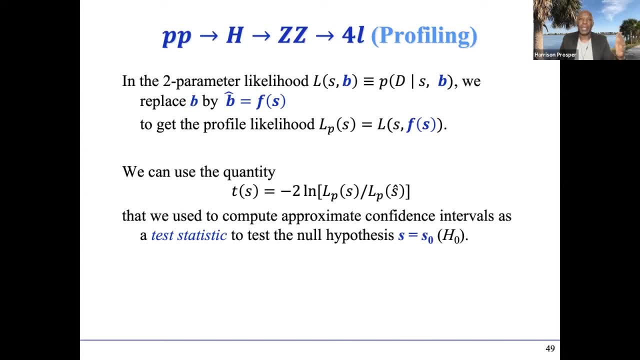 is that we are in a workshop in which we're thinking about Suzy and searching for Suzy. Necessarily, it means that we are going to be working where we are in the unfortunately in the, in the regime where we have few counts. 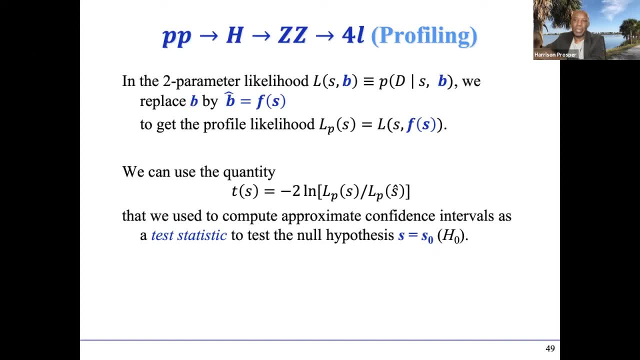 We are in the tails, we are in phases, in phase-phase, that are more difficult, trickier, And unfortunately that's exactly where assumptions matter the most. So it's kind of unfortunate. Thanks, So, with the chair's permission, because time is, the clock is ticking. 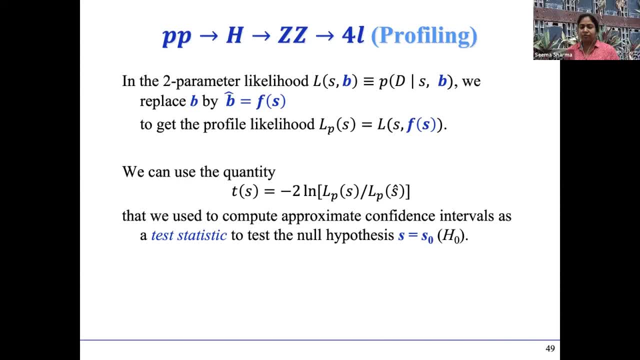 I had another quick question on the Wilkes theorem. If it's not super urgent, then maybe we can move to Ritopanna quickly and relieve Harrison. It's already close to 2 am for him. Yeah, I had a question about Wilkes theorem, but actually 3 am for me. 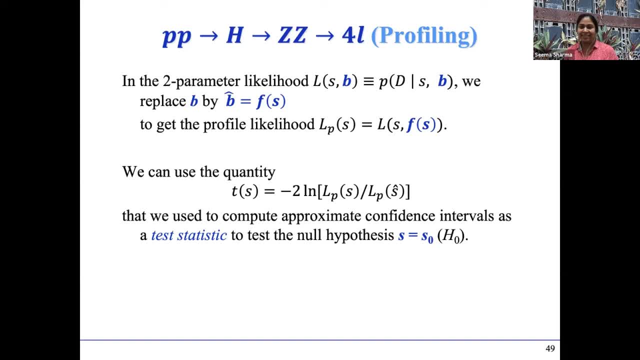 3 am for him. yeah, Yeah, sorry to interrupt Shartaki, but I think let's take one last question and that's from Ritopanna. So my question was: while you were comparing two analyses based on alpha, 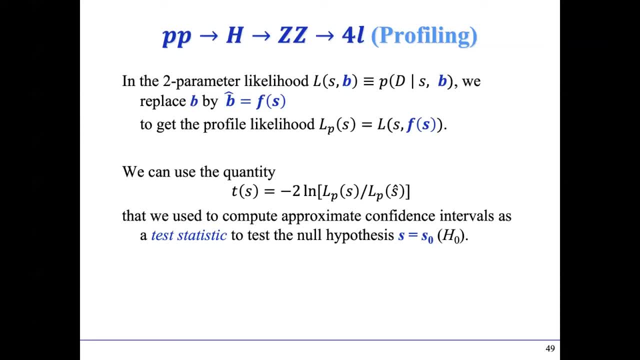 so what did you mean by analysis there? I mean, is it using Bayesian or frequentist, or what did you mean by analysis? Okay so, let me okay, so, any analysis, but let me be very concrete. Suppose you are testing a particular point in the parameter space right of the NMSSM. 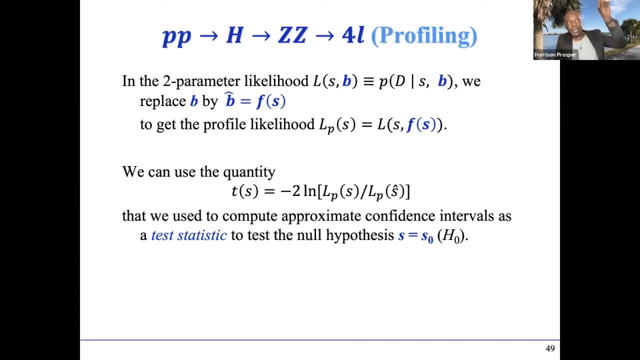 So your theory colleague tells you this point is particularly interesting and you're going to design analysis. So you're going to design analysis to test that particular point, to really investigate that point. okay, So you simulate, you know events at that point, so you have a whole bunch of signal events. 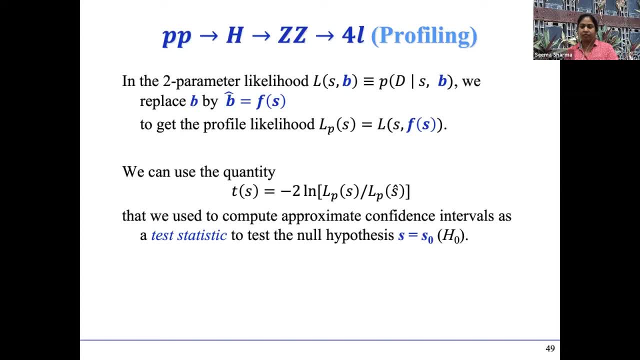 and of course, you have some model events that you generated And now, because you want to have an optimal analysis, you choose to use a machine learning model to build a classifier. So you have signals that you've generated at that particular point for the NMSSM. 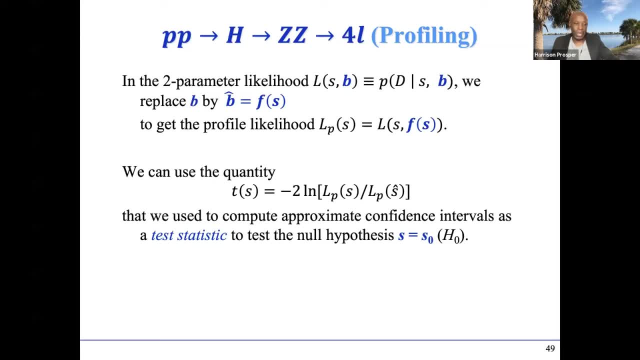 You have some model events that you've generated. You use that to construct A, to construct a. you know a machine learning descript classifier. Now another person comes along, does the same thing. They also build a machine learning classifier, but they present you with different variables than you have. 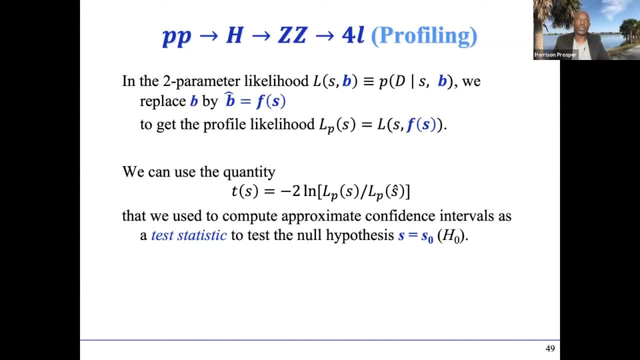 Okay, And so now you want to compare your two analyses. And so what do you? so you both agree, let's, let's apply different alpha thresholds, right? That corresponds to different cuts on your machine learning model. Let's say you're going from zero to one. 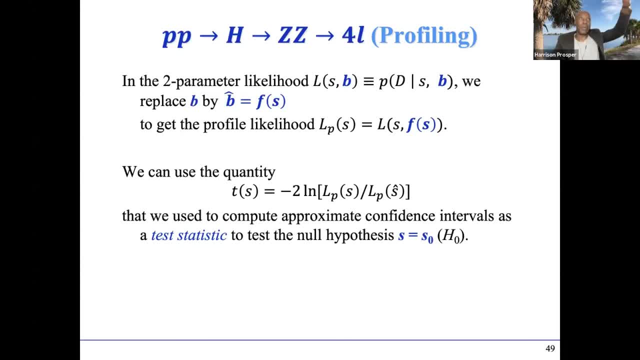 And now you, you make this plot of you know the power of your analysis, right, You know versus, versus the, versus, this cut, And and the point is, if you do that, it could well, it could be that your analysis is always going to be better for every possible threshold. 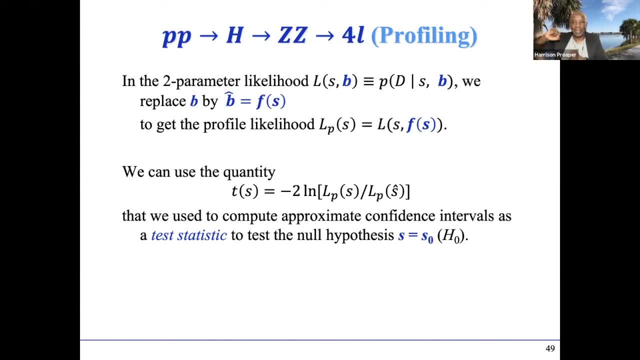 Which case, of course, you win and you should do. we should do your analysis and forget about the other. Or it could happen that for some threshold you do better, Okay, And for other thresholds the other analysis does better, right. 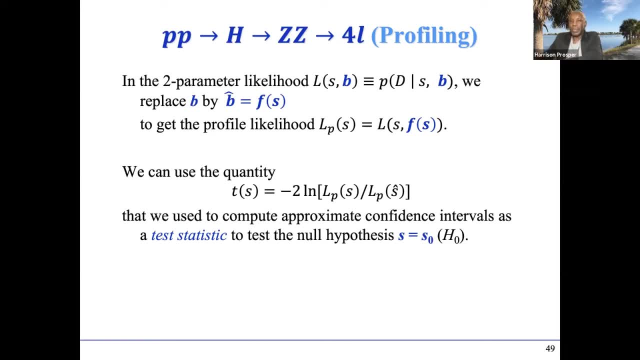 That's, that's one example, And it could also be that you do a basic analysis and the person does frequent analysis. It doesn't matter, but you can still compare your analysis on the same curve, right. It's a bit. it's a bit like the rock curve right. 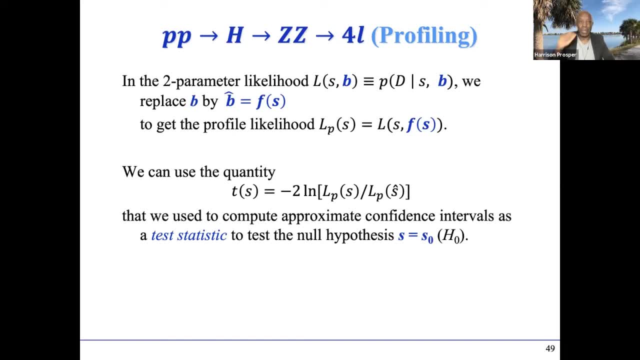 When, when people build machine learning models, as you, as you will learn from from my colleague when he talks about machine learning, one of the ways of comparing different machine learning models that you, you look at the rock curve And that tells you, you know how. 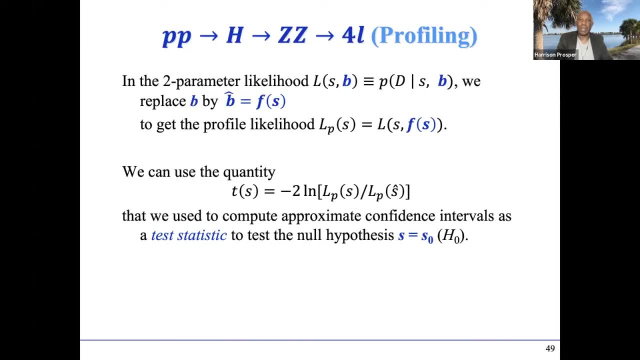 How well one is doing versus the other. So that's what I mean by an analysis. It doesn't depend upon whether it's frequencies of Bayesian or whatever, It's just just a direct way to compare. Am I, is my analysis better able to distinguish between the this N-MSS, this N-MSSM point at a particular parameter point and and some other particular theory as a function of different thresholds? 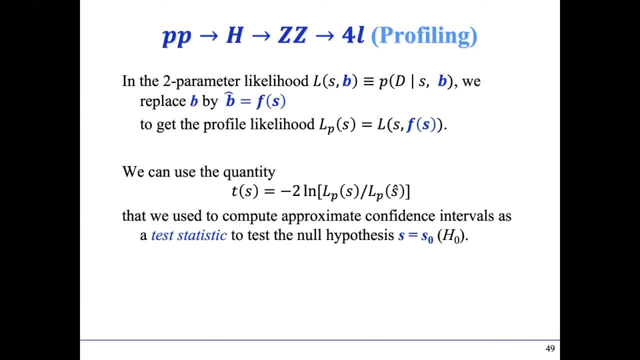 and not like that. I mean how important that it is actually for humans. Thank you very much, Harrison. So anyone, I think I will hold on to the questions beyond this point, But sorry, Shaktik, you've interrupted me, but we can start with a discussion session later on. 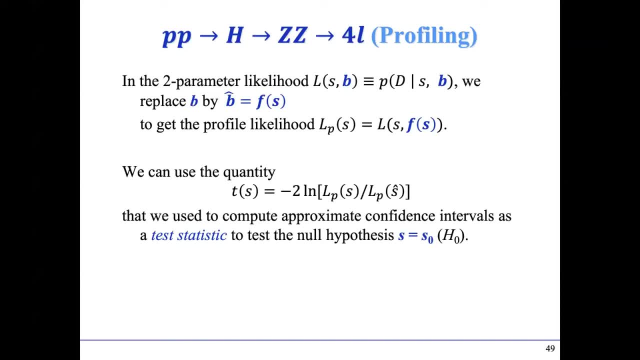 In coming weeks or coming months? Satyaki, I hope one. We have talked about it in the past year, but now it's close to 1.30, so no problem. Actually, if Shamas is willing, I can entertain one more question from Satyaki. 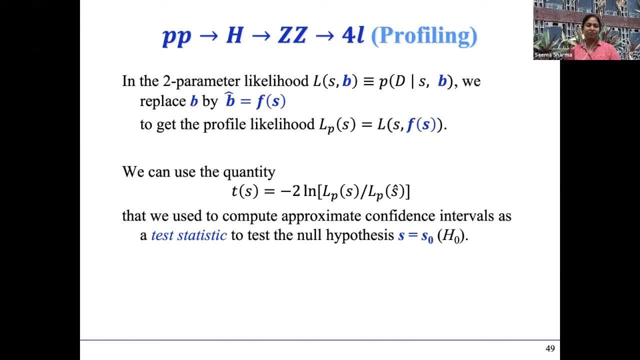 Sure, please go ahead if you're okay. Okay, so a quick question. So I think you mentioned today also that Wilkes' theorem has this right or right, that the parameters cannot be on the boundary of the…. That is correct, Yeah, so in our case? so the null hypothesis, that standard model, is true. is it not a case where S equals zero is on the boundary because…. 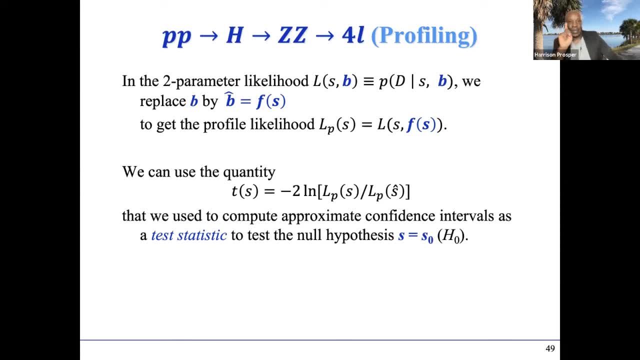 Ah, so what is…. Yes, so you are correct that S equals zero is the boundary. However, the theorem requires that the maximum likelihood estimate of S is away from the boundary. The problem, of course, arises if you get an estimate of S that is negative. 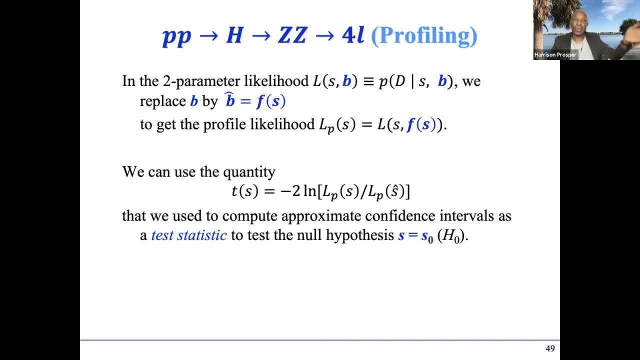 And in that case, since you know the parameter space is bounded at zero, you basically set your S hat equal to zero. And then now you have your S hat at the boundary and then Wilkes' theorem fails. And actually I wish I knew that when I was in my 20s. 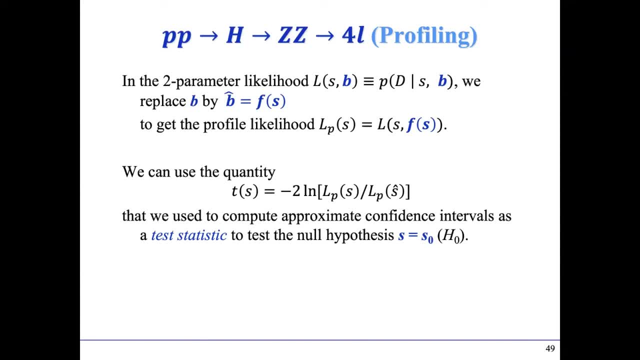 Because when I was in my 20s I worked on an experiment in Grenoble, France, looking for neutron antigen oscillations, And in that experiment I got a negative signal and I did not know that this happened. It would have been useful to have known that then. 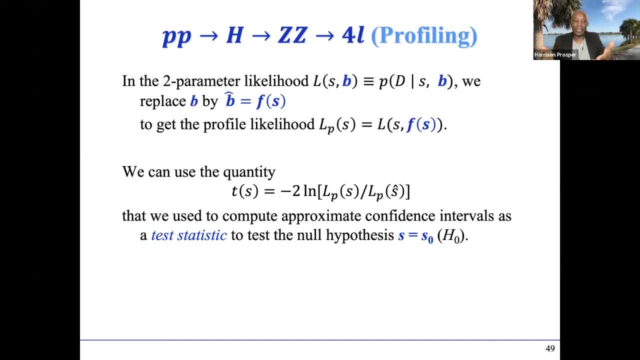 But yes, you're right. So if you have to get a negative signal, just by chance you get a negative signal. Nothing wrong with that. That happens. But you know that the parameter space is bounded at zero And typically what we do is that we say, OK, fine. 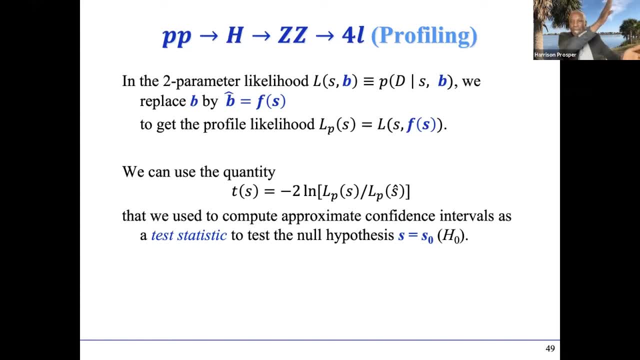 Well, negative signal doesn't make any sense. So then we set the signal equal to zero by S hat, And then that destroys Wilkes' theorem. Yeah, And in Kahn's paper- Kahn and three other authors that paper- they do take care of it in that way that demand that S hat cannot go below zero. 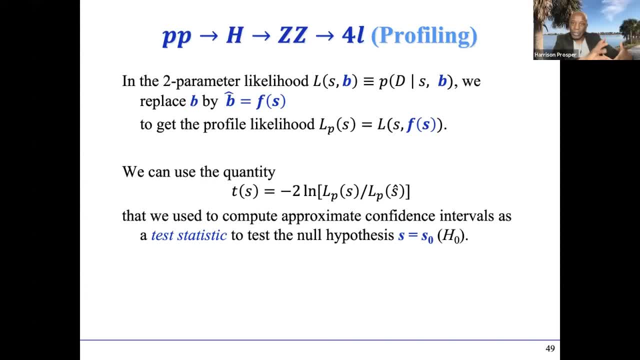 Yeah, And then they use the Wald's approximation to derive Approximate probability densities for those situations. It's no longer chi-square, It's not the Wilkes' theorem anymore, but some different distribution. Yeah, It's a modified Exactly. 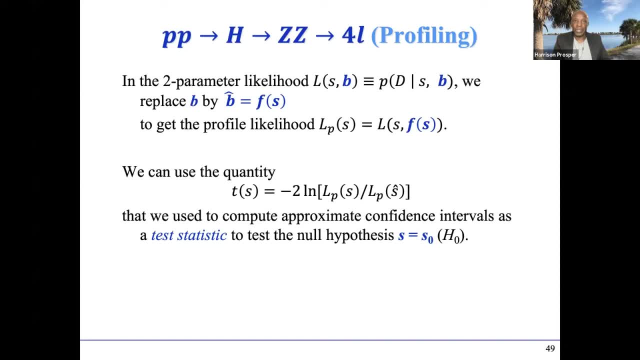 Yeah, And actually it's really instructive actually to do a simulation where you do or you do not set the negative parameters to zero. If you don't set the negative parameters to zero and just take whatever The next thing Michael gives you, then you get a perfectly beautiful application of Wilkes' theorem. 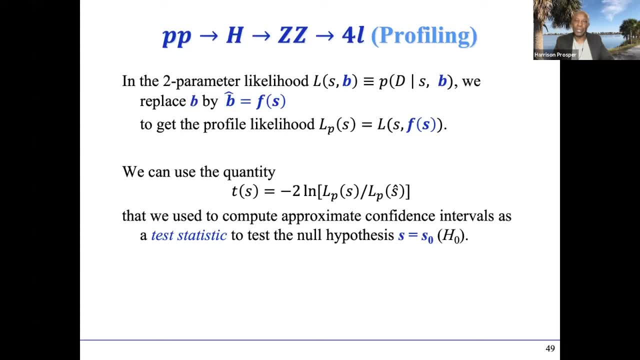 It just works even for incredibly small numbers. But as soon as you do this truncation and set S hat equal to zero whenever it is negative, it doesn't satisfy Wilkes' theorem, And actually it doesn't satisfy any of the things in Glenn Cowan and company's paper either.